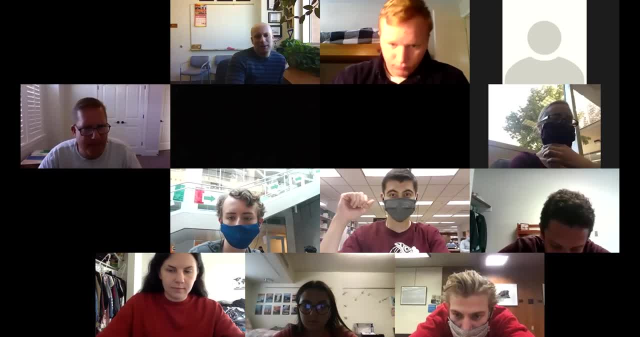 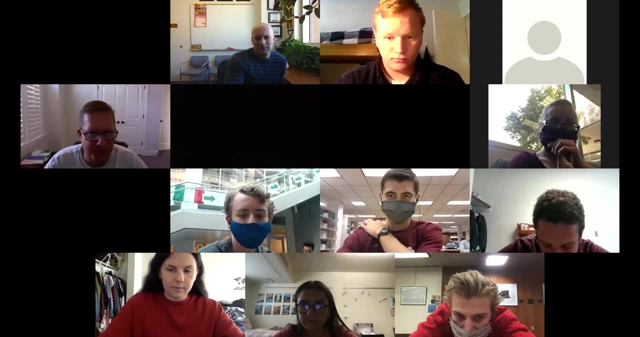 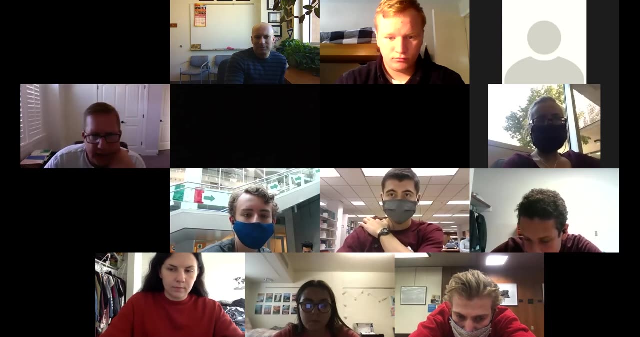 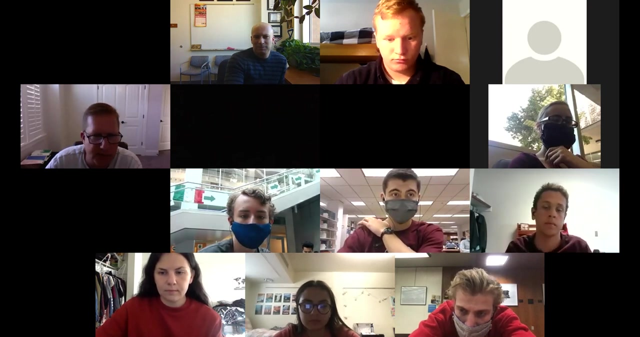 That's to protect the anonymous nose pickers out there, And so we have to be careful and conscientious of those. Oh man, Okay, Well, anyways, yeah, no, I appreciate the opportunity to come talk to y'all, And what I appreciate more is the fact that I can start seeing some of your names so that when you come into my classes, I will have a better chance of remembering them. 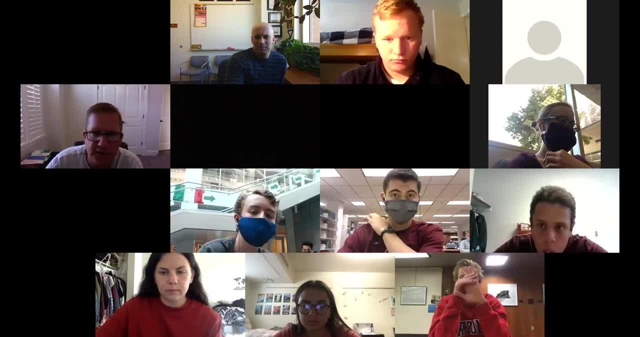 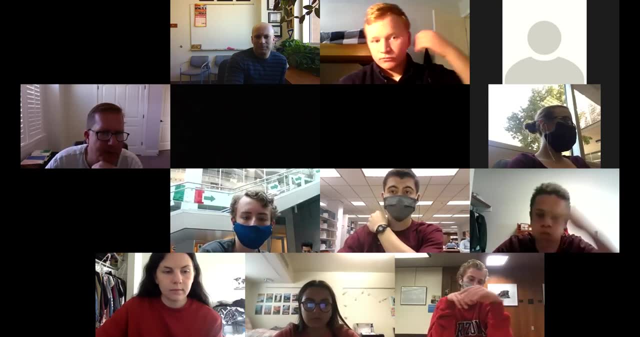 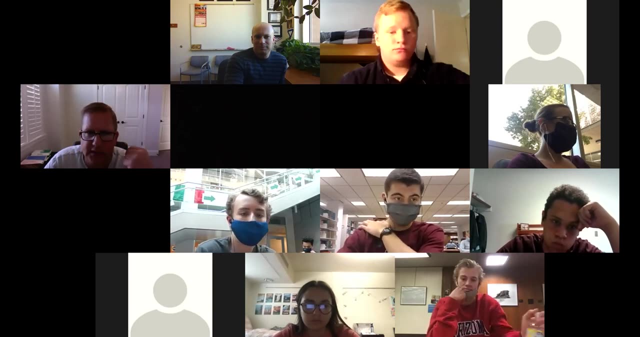 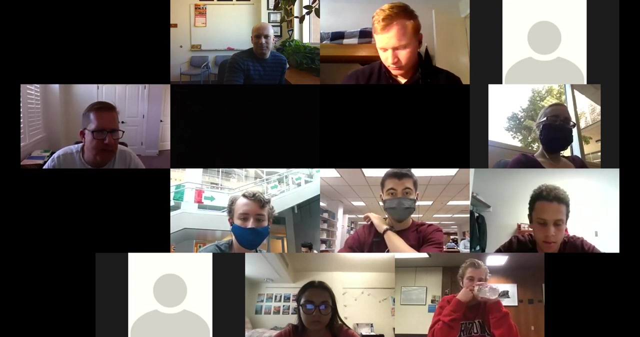 I'm looking for any unique or interesting names here. Looks like you got it. You got all the standard ones. Kevin, There's okay. Nick without a K, That's kind of unique. Just the NIC, That's kind of fun. Cecily, I knew a Cecily, But okay, I got a. I see everybody's here. Well, good, What happened to all the Daves? What happened to the years when you had, like Mary and Martha and Dave and John? Do you have any Johns? 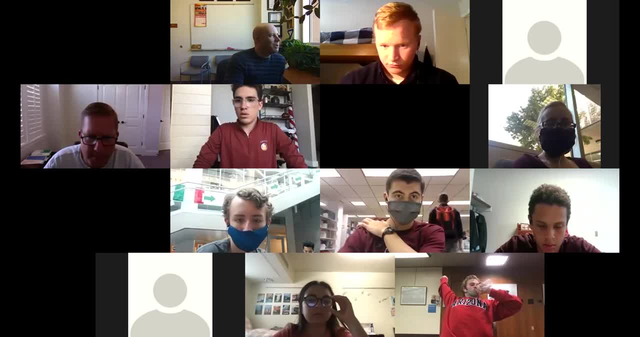 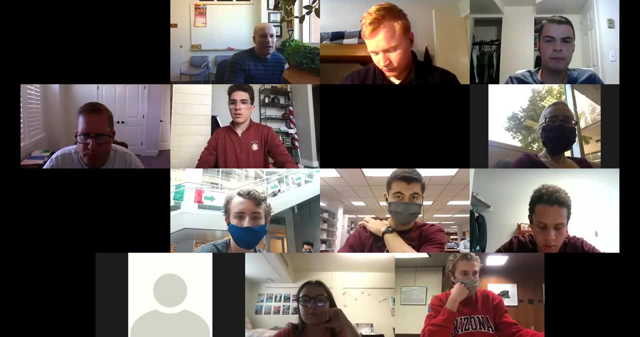 One of the things I've learned: after you've had this job long enough, you get to see the trends of what, how parents named their kids. There was a period where we had lots of Daves, But I don't see that very often anymore. 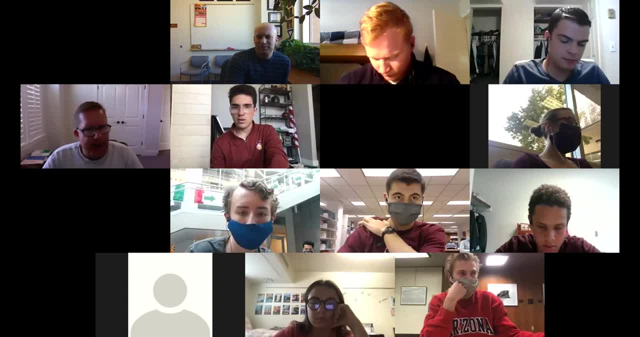 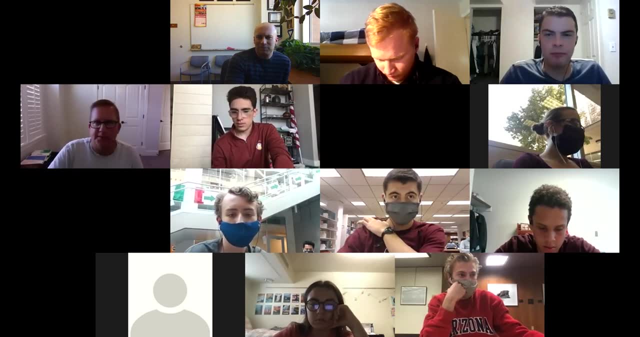 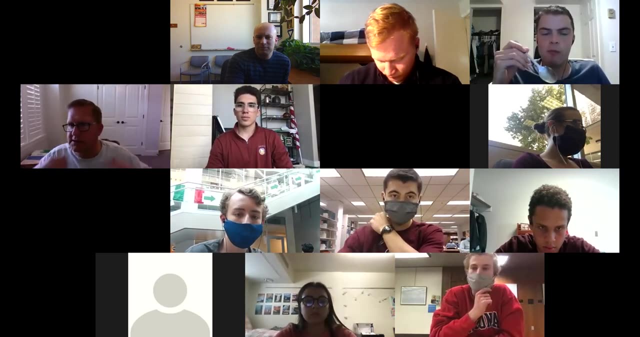 No, Daves. Oh, I see a Mary, That's good. And Haley and okay, Well, hi everybody. So yes, it's Kevin Franke. your professor said My name is Dr Ames. I'm a professor of civil and environmental engineering. I am dressed down today. This is casual Tuesday. I didn't come into campus So I decided to. 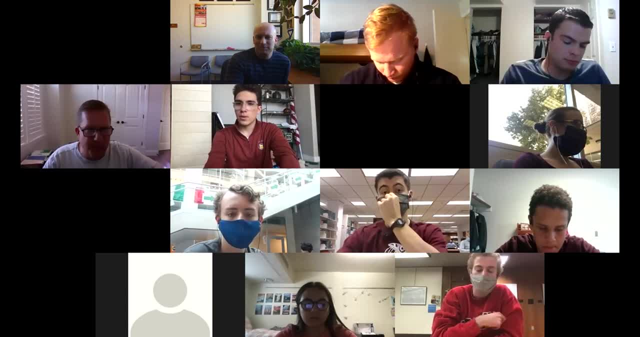 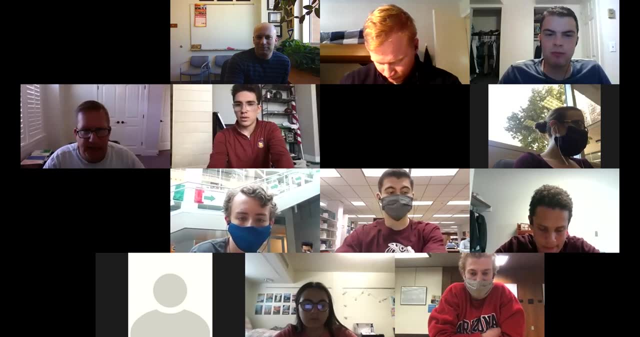 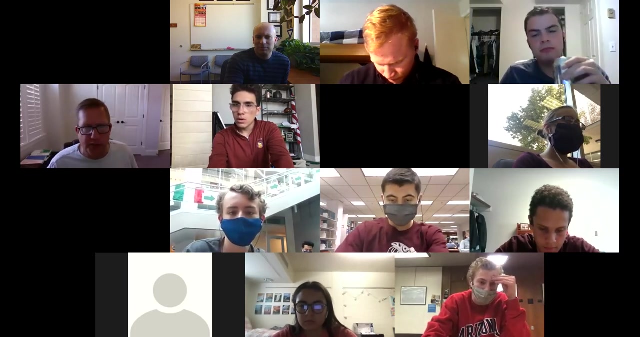 to dress down and keep it easy, And I've got my Diet Mountain Dew. here I'm sitting in my home office and a bag of M&M's And just really having a good time, And I've been looking forward to talking to y'all since I got invited a couple months ago. I want to talk to you today about sort of what is water resources engineering, keeping in mind that what I'm going to be telling you or sharing with you is like my view, my world view- of water resources engineering. 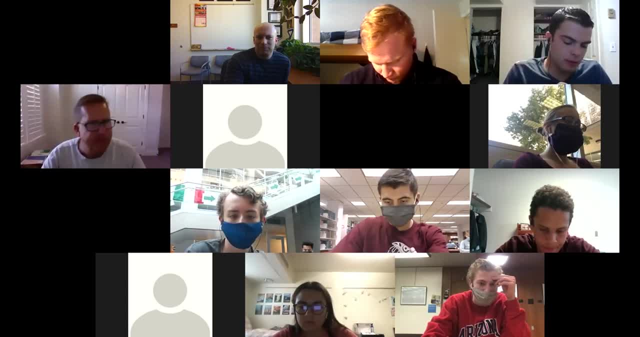 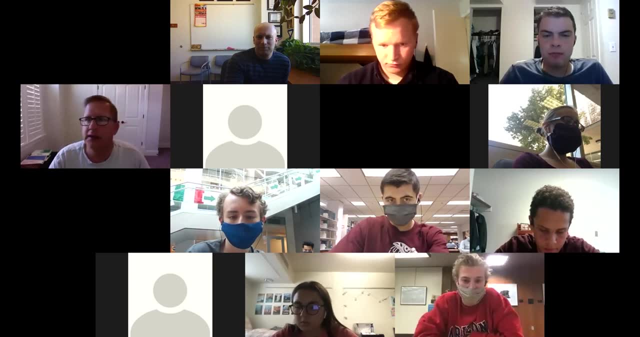 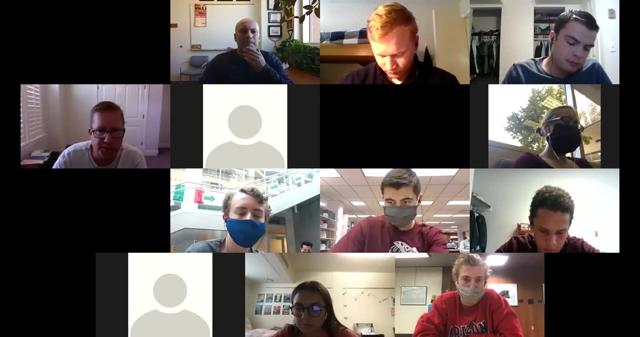 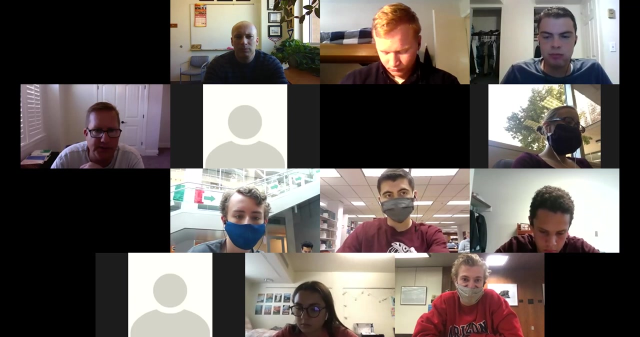 It's a huge field. It's a huge field. It's kind of like you're probably already discovering that civil is a huge field and people say, oh, you're in civil engineering. What is that? You're like, oh man, where do I start? Because there's so much to it And it's kind of like I feel that way about water resources engineering. There's just a lot. So let me see if I can share my screen. I'll share with you a couple slides and talk a little bit about this. What is water resources engineering? 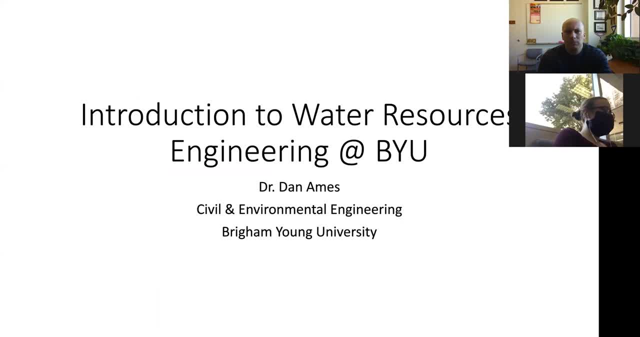 All right, Okay, is that showing up as the presentation mode? Yep, Awesome, Thank you. And, by the way, Heather, it's good to see you again. Heather's in one of my other classes. So, yeah, I suggest, I suggest you all. She is a quality human being right there, Like if they wanted to select somebody to represent the Society of Women in Civil Engineering. 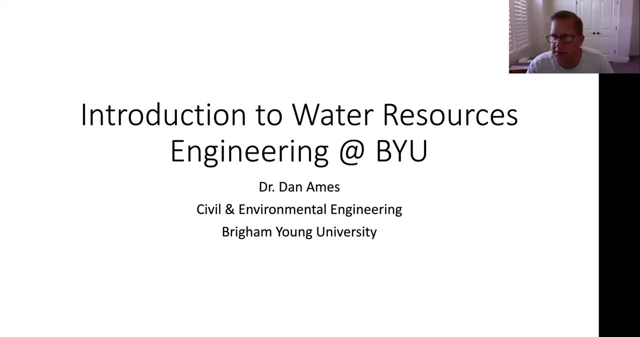 Heather's your girl right there, because she is hardworking, quality person. I recommend y'all go join. And did you say you're providing free food too? It's on Zoom, So normally there will be free food when it's back to real life. 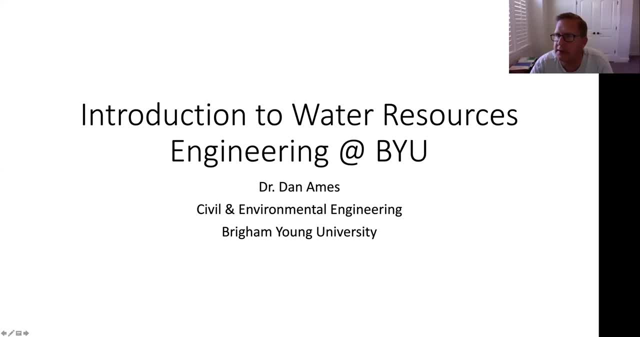 That's the worst thing about all this Zoom. BYU is, and Dr Frank, you probably attest- BYU gives away more free food to students at student society meetings and meetings and events than anywhere I've ever been. So you don't call it the freshman 15 for nothing. 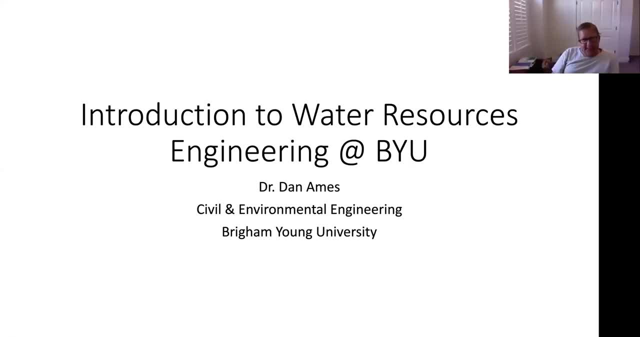 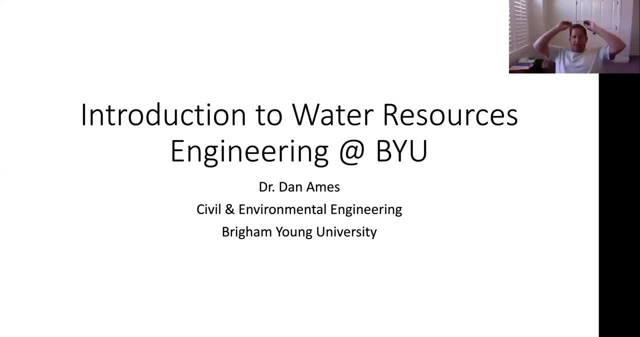 Yeah, Yeah, Yeah, Yeah, Yeah. So what are you says engineering is kind of cool because water pervades everything in civil. In fact, you know, you, you, if you want to get into transportation, you're going to deal with culverts and how waters. water runs off the top of roadways and also outruns underneath roadways. 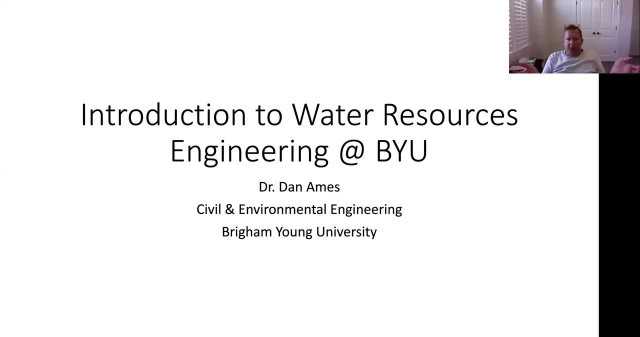 If you're going to get into geotechnical, you're going to have some interactions: water engineering, because geotechnical is here and water resources is here. in between is groundwater And the way that the saturated zone and the the all of the water at the water table affects what happens with geotechnical engineering. 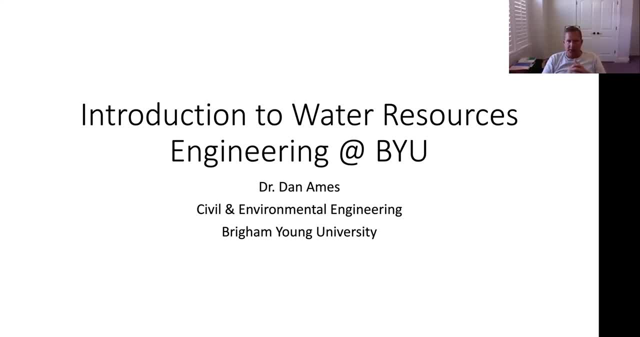 If you build a foundation for- whether it's for a road or a building or anything- you're going to deal with water. Construction engineers deal with water all the time, not only sort of natural water systems, but also engineered water systems, such as water supply and wastewater treatment and water treatment. 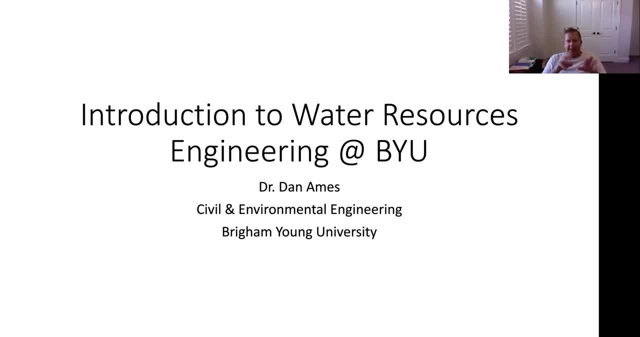 And so, really, water resource engineering has its little fingers in all of the features, And so you're going to get into the fields of civil, And that's okay, Because what that means is any one of you, you know, will benefit from taking a water class or two, or even if you decide to emphasize in water, you'll find that you'll use it in your career wherever you go. 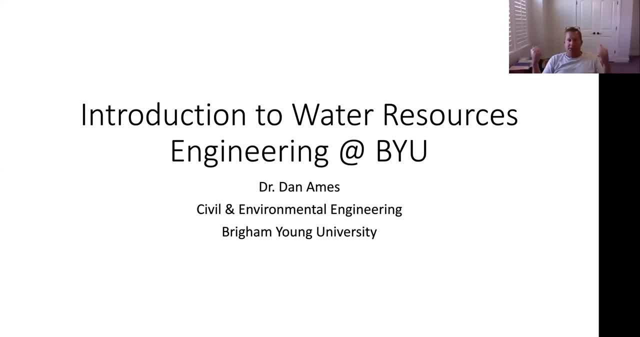 My brother- my big brother- at Utah State University was a year ahead of me in the program. He got his master's degree in water resource engineering and ended up going to work for UDOT as a transportation planning engineer and does project planning, project management. 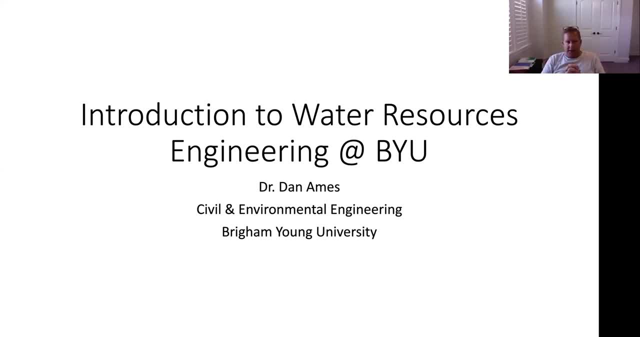 And all kinds of stuff, So All kinds of UDOT-y type things. But he said that at the end of the day it worked out great for him because transportation is very traffic and water behave very similarly in a lot of ways. 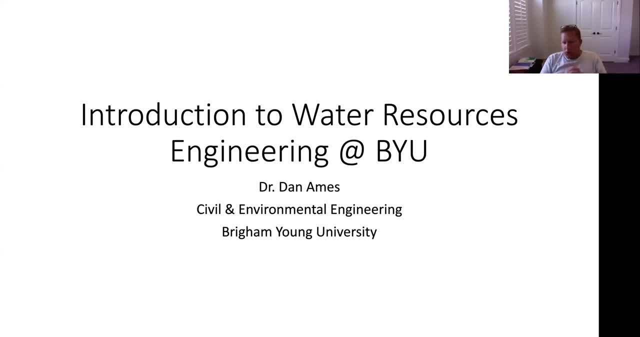 A lot of it's about flow and control And then, of course, just the knowledge of the water health. So I always have to give this little speech that you guys that are literally at the beginning of your program. I don't want you to pigeonhole yourself as well. I'm only going to do structures. 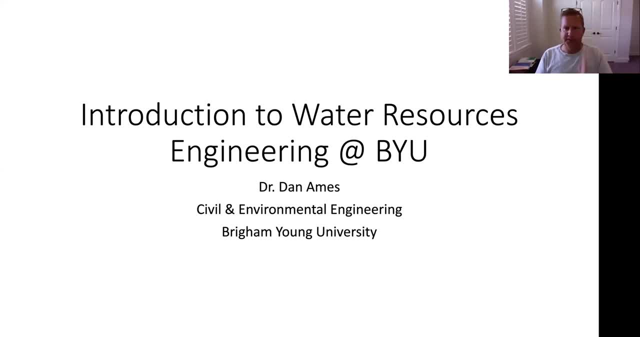 I shall design steel beams until the day I die. Or Oh, I'm only going to be a traffic engineer And I'm going to come up with the craziest, wackiest traffic patterns anybody can think of, And I'm going to test drive them all right here in Provo and Orem. 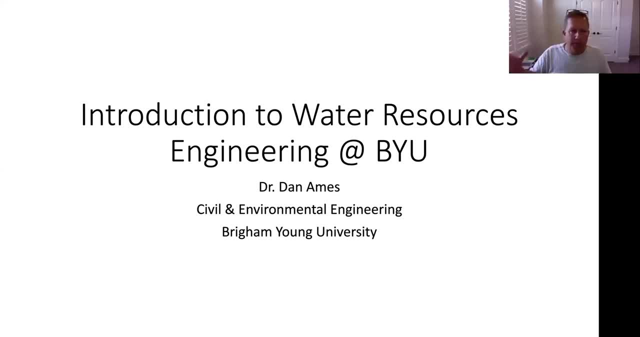 Don't like put that in your head right now, because there's so civil engineering is so broad, There's so many cool things you can do, including water, And I would actually recommend people sort of be as broad and diverse as possible as you carry on with your program. 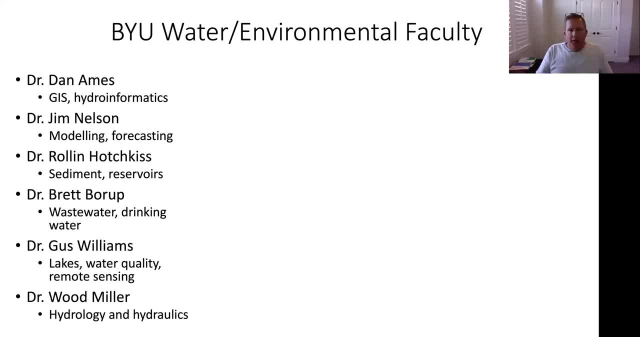 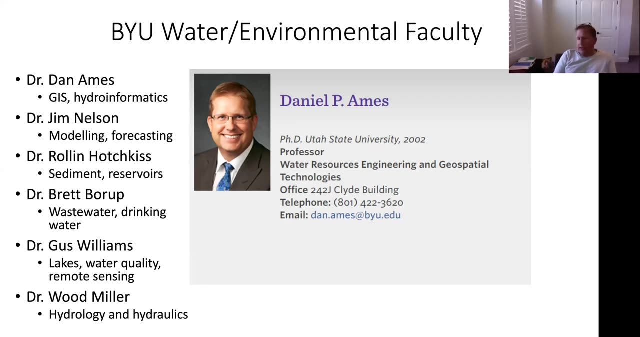 So water, Water and environmental faculty at BYU were sort of a loose cohort of people that are involved in water, And there's myself up there. I'm sort of water resource engineering and geospatial technology, So I teach classes on GIS and surveying and geomatics as well as do water-based things and modeling. 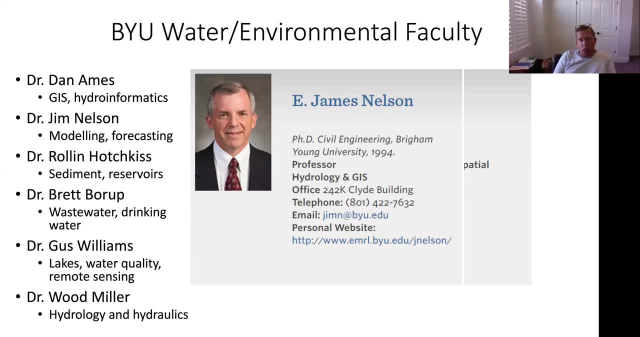 Dr Nelson does a lot of modeling and simulation and forecasting And he's been in the news lately because he's been developing models that simulate water flow every single river around the world in real time. It's really ridiculous what he's been able to accomplish and get a lot of good publicity for. 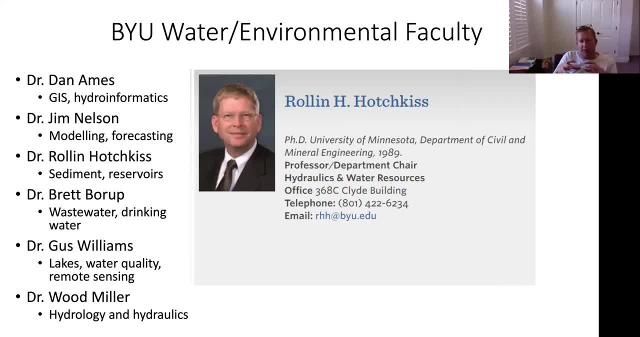 Dr Hotchkiss. he's really interested in a local scale of water and particularly what's happening with sediment and rivers, How sediment builds up in lakes and rivers and how it moves through lakes and rivers. And he now- keep in mind, by the way, some of you might be going- whoa, whoa, whoa. 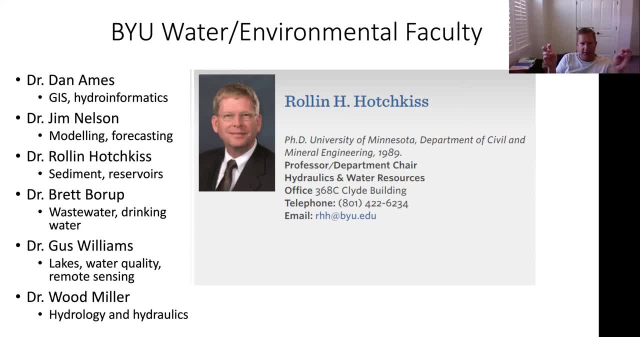 I care what these professors are- quote unquote- interested in: Just give me my dang degree and let me get out and get my job. Well, the point here is that all of us teach classes across the spectrum of water and environment and GIS and modeling and things. 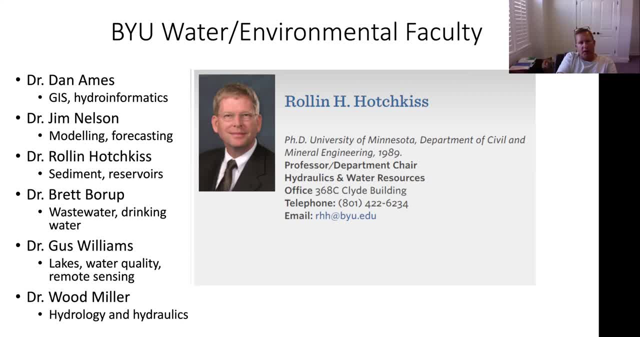 But we also hire students as undergraduates to work in our research labs. So when I say we're interested in such and so really what I'm saying is: hey, we've got some cool, interesting research projects going on in these areas. 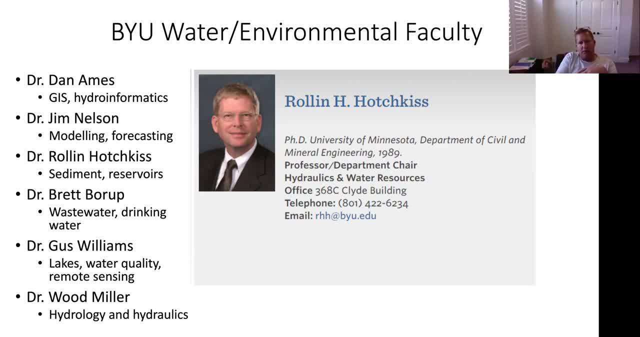 And if you want to do undergraduates, If you want to do undergraduate research and get paid while you're going to BYU, rather than flipping burgers over at you know wherever, then try to get involved in one of the research groups and research labs. 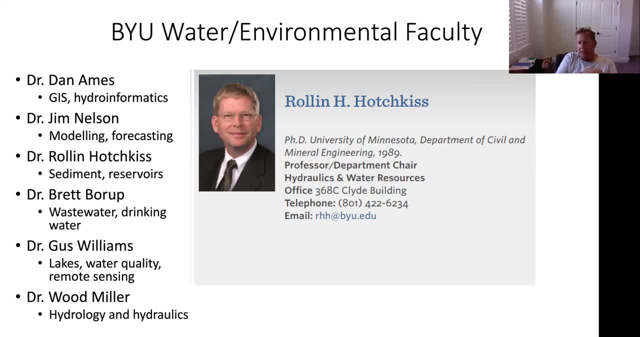 So Dr Hotchkiss, he hires students, undergraduate students, to study sediment and think about. He also does this really cool work where he looks at how little low head dams, water flows over the top of them, And when I say low head meaning it's like a short dam, maybe a meter or two high and water is just flowing over it- and how people die in those. 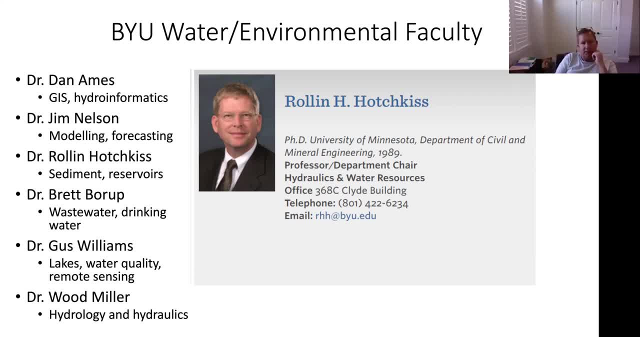 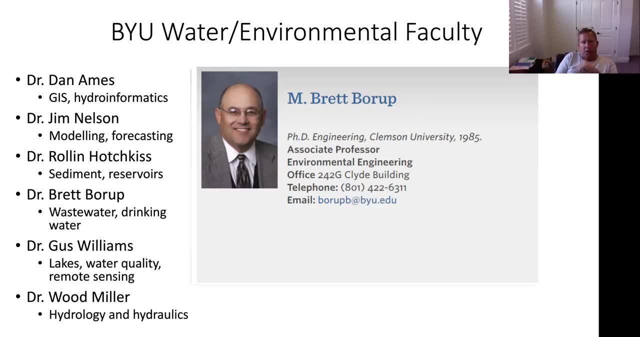 And if you can re-engineer those, how you can keep people from dying. So that's some of the research he does. Then Dr Borup: he's one of our environmental engineers. He teaches classes on water quality and like wastewater treatment. 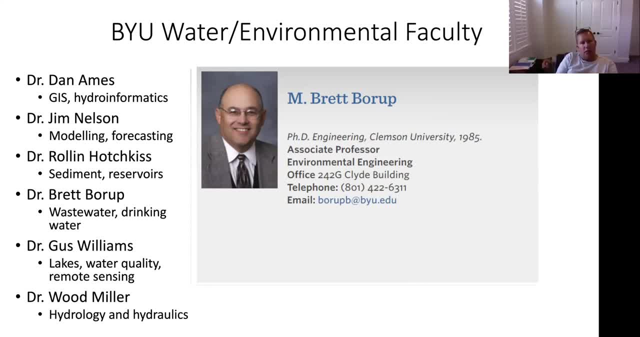 If you're going to get into construction, you're going to have to deal with water supply and water wastewater treatment, And so he teaches classes on water quality modeling or not, water quality treatment for water, for drinking water and also for wastewater. Dr Williams is a professor also on a little bit more on the environmental side. 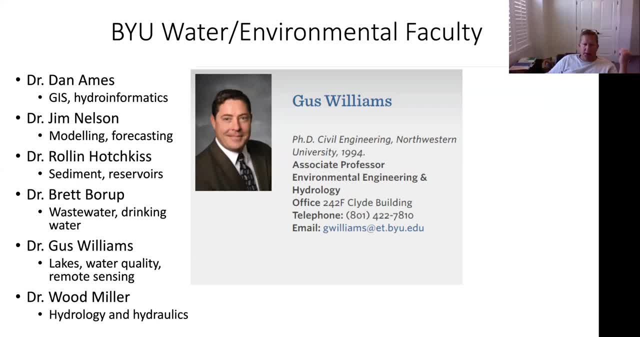 He has a lot of experience. Yeah, He has a lot of experience with the army and actually some kind of top secret military stuff. But he also does cool work where he looks to reservoirs and lakes from satellites in space and tries to determine the quality of the water from space. 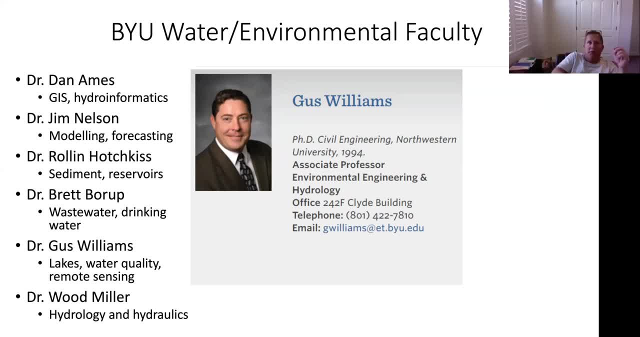 It's really ridiculous how we can do that. I mean, we're basically looking at reflectance and different patterns in the signal of reflectance. going back to the satellite, You can sort of tease apart: Is this got it? Does this water have algebra or what kind of 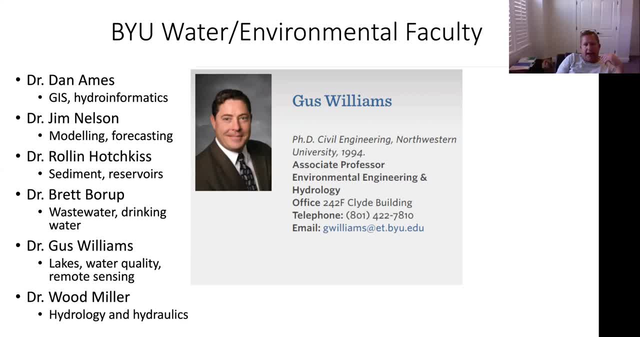 What kind of water quality problems are going on in that lake. And part of his work is fun too, because he takes students out in boats to go paddle around lakes and to check the water quality and then compare it to what they're getting from satellites. 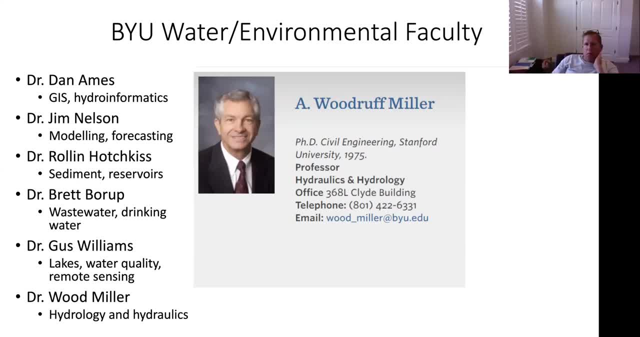 And then finally Dr Miller, he also. he's been around here a little bit of a while, As you can see. he got his PhD in 1975. But Dr Miller teaches a bunch of our hydrology and hydraulics classes. 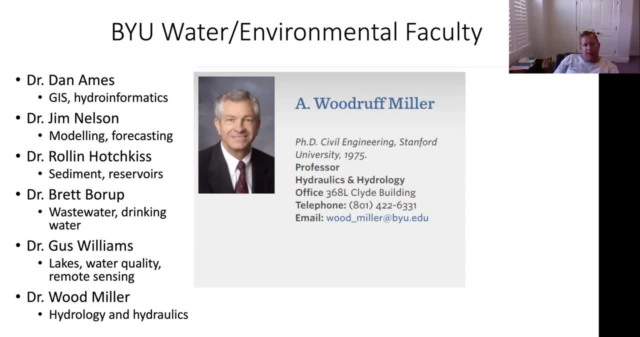 And his research area is quite interesting too. He likes to go up to Yellowstone National Park and study the water quality And all the lakes up there And for years has sent students up there to do that and analyzes it. So that's the basic group of faculty. 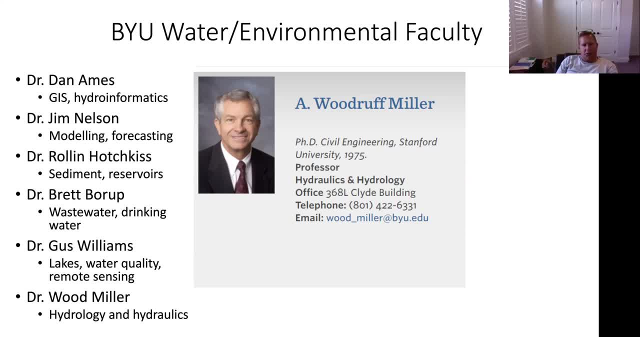 We also have Dr. I actually need to include on your Dr Jones, Norm Jones. He sort of has his foot in this. He's more of a geotechnical engineer but because he does groundwater he's also related to us. 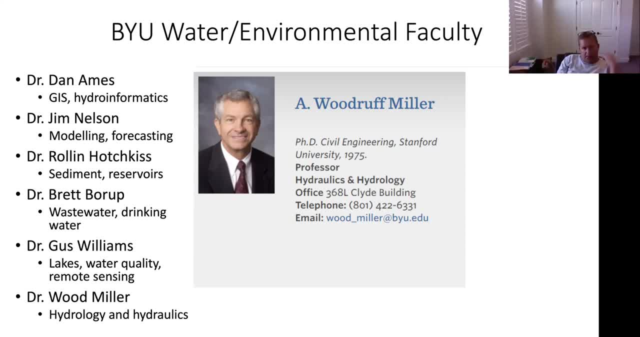 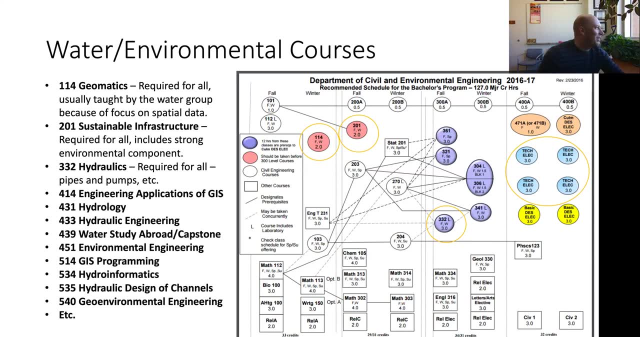 So he's our department chair and does studies groundwater. For the record He has he has quoted and said in public that he's part of the water group, So That that would be our chair. Dr Jones Got him to the slide. 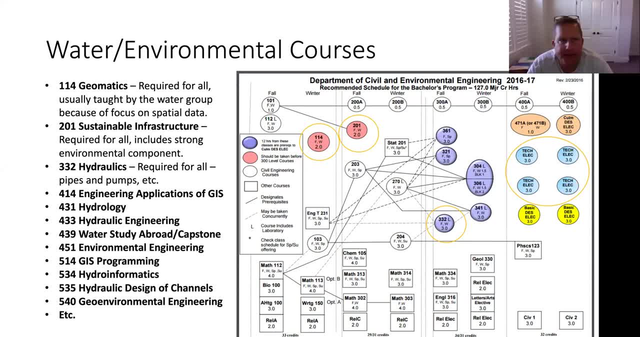 Take in Classes now called 214. geomatics is required for everyone. It's usually taught by somebody in our group. We do spatial data stuff And and just like Dr Frankie covers a lot of these one on one classes, I usually cover the geomatics 214. 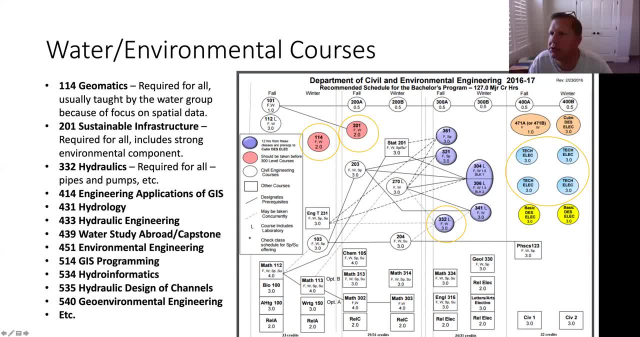 So if you're, some of you may be in my genetics class, If you're in my geomatics class, say something on a chat so that I can say hi to you. Jim Maddox is pretty fun. We start semester with surveying and then we get into using GPS to collect data. 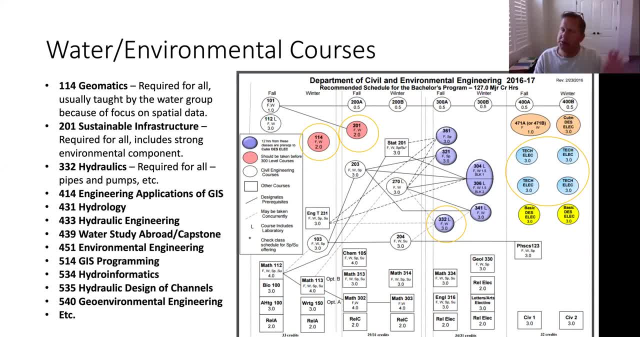 And we look at satellite and a little bit of imagery stuff And then we download a lot of data from the web and we put it in software to make maps and learn how to build maps and how to analyze a little bit of spatial data. That's a fun class. 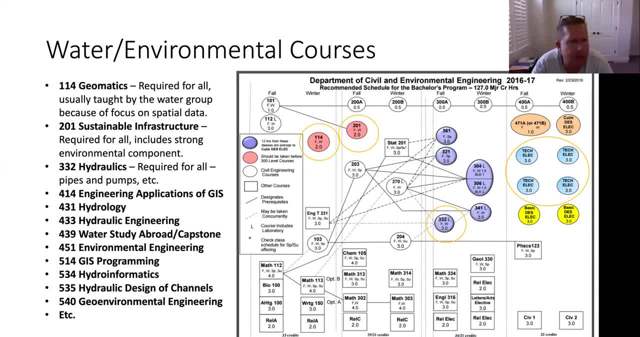 And if you haven't taken it yet, you can take it next. semester 201 is sustainable infrastructure. We also teach out of our group hydraulics for 14 class, If you're interested in maps, map making, spatial data and modeling and all that kind of stuff. 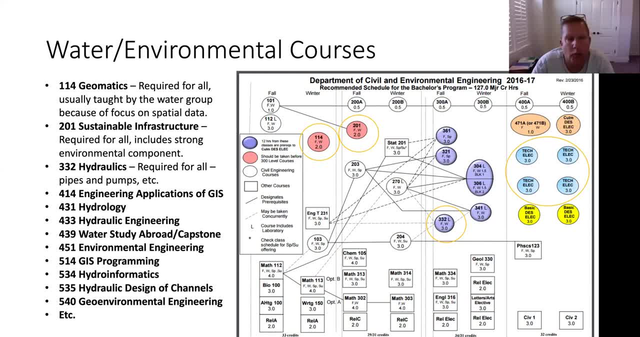 Or if you want to end up working in one of the research labs, like the hydroinformatics lab, the transportation lab or even Dr Dr Frankie- Dr Frank's lab, Dr Schultz's lab- all have benefited from having students that took 414 sooner than later. 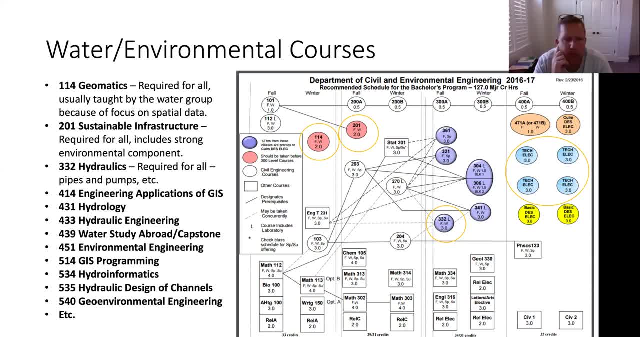 So that's one you could take sort of in your junior year. You can even take it in your sophomore year if you have room for it. So don't hold it out until the senior year, because this also gets you internships. If you take 414 early, then you can go get internships outside of campus at engineering companies and tell them that you know GIS, and they'll just be thrilled. 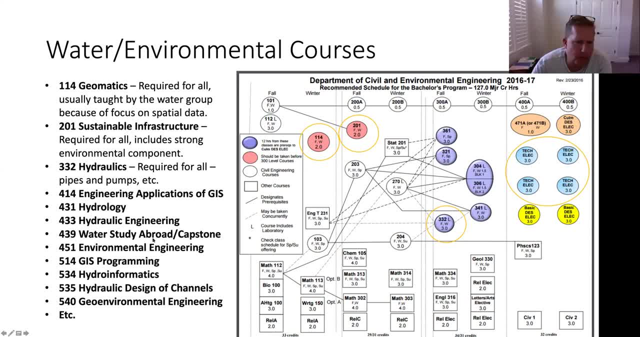 Hydrology, hydraulics 439,. I'm going to show you some pictures of our water resources study abroad program. And then there's some environmental engineering and an advanced GIS programming class and hydroinformatics and some other fun stuff. geoenvironmental engineering. 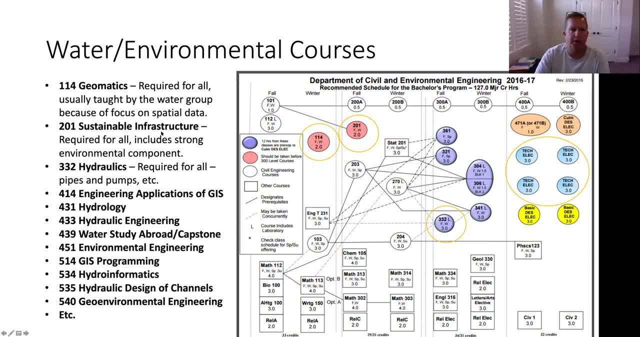 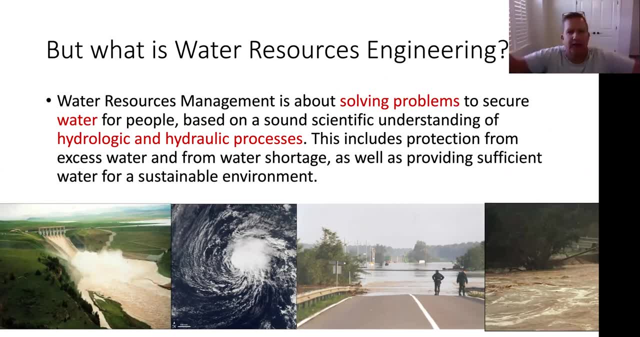 So these are the types of classes That come out of the water group. But you may ask, Dr Ames, what is water resources engineering? Well, I'm about to answer that for you. Water resources management and engineering is about solving problems to secure water for people. 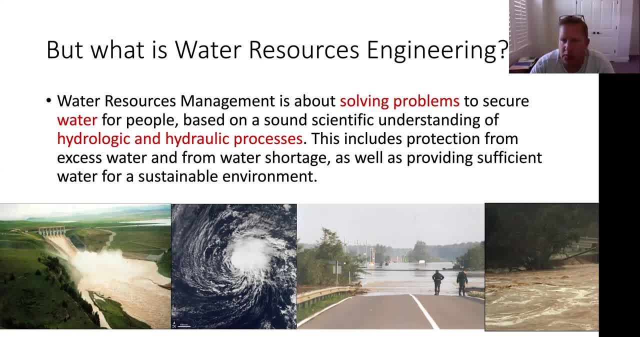 And so we're basically, in a nutshell, we're looking for the right amount of water and the quality of water to sustain life and the environment. And so quantity of water. We could have issues related to drought, We could have issues related to flooding. 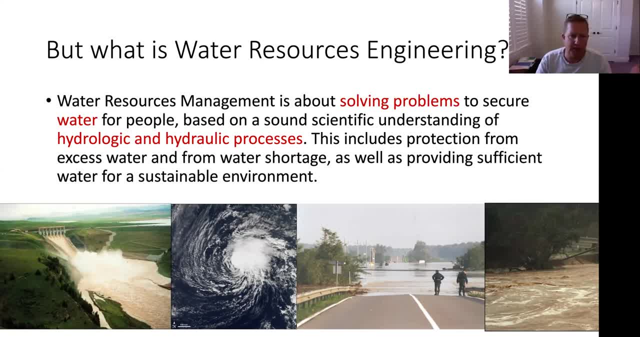 Quality of water. You can have clean water and very contaminated water and everything in between, And there are issues in protecting the water so it stays clean, And there's also issues in cleaning water using treatment methods. So overall, it's all about water. 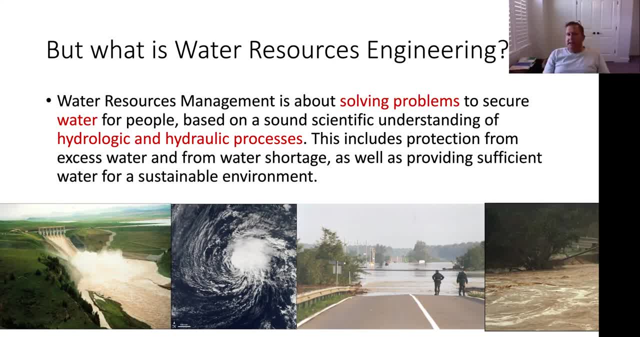 In fact, I sat on an airplane a few years ago. I was flying back, I think, from Washington DC, back to Utah, Back to Washington DC, Back when we used to have airplanes and we'd go on flights to travel to places. 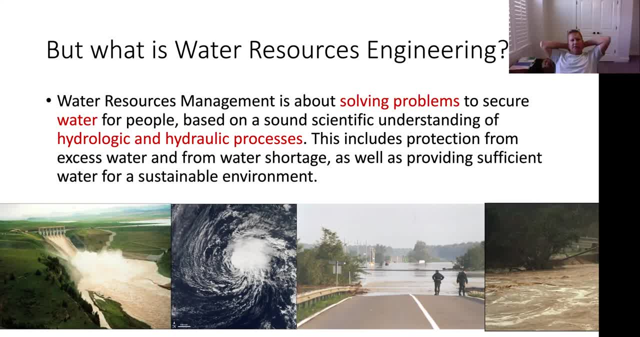 I'm using air quotes because I haven't traveled anywhere in months. And I sat down next to this lady and she said like very first thing, hey, oh nice to meet you, blah, blah, blah. And the first thing she asked me was: what do you do for a living? 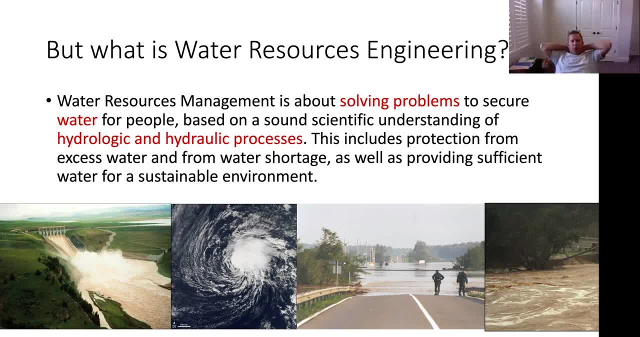 And so I'm a professor. And then I was like trying to fall asleep again And she's like, oh well, what do you teach? And I started to learn my lesson. you're supposed to say math. I know it's lying. 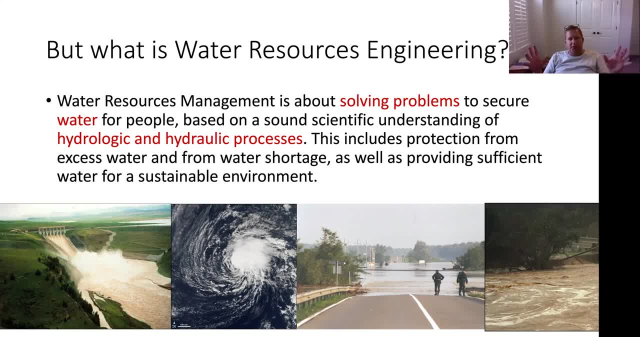 But you can cross your fingers when you do it and then it's allowed. You're supposed to say math, Because everybody understands math. They've all taken a class in college on math. So if you say you teach math, then they go. oh, 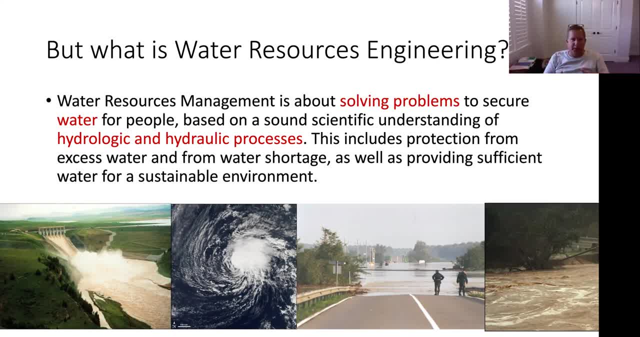 And then they didn't like it. So they never ask you more questions about it And then you go back to sleep. But instead I forgot to say math and instead I said: oh, civil engineering, and focus on water. Civil engineering, she said. 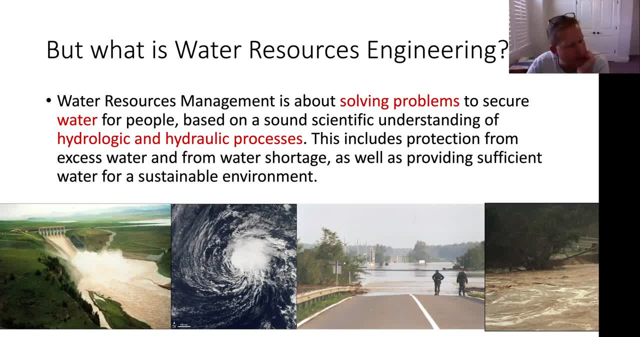 Civil engineering. Now, I've heard of mechanical engineering and electrical engineering. I haven't really heard of civil, But I guess that's one of those words, Those ones that doesn't really affect people on a daily basis too much, And I'm like, hmm, 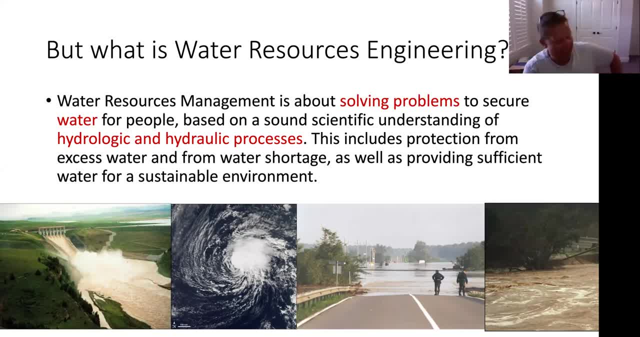 Suddenly I'm awake. I have something to say. Well, actually, as I rotated my chair toward her, I said, actually, if I could be impertinent and ask you, did you take a shower this morning? Oh well, yes. 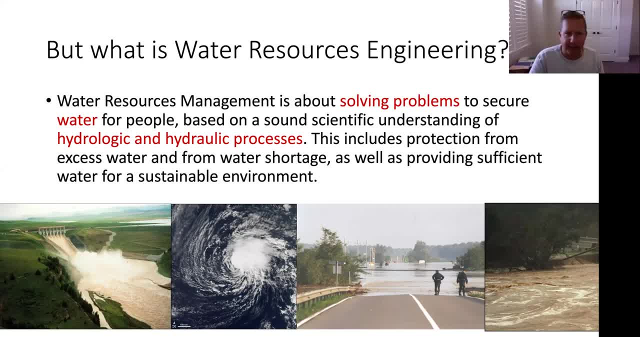 And I said I suppose you also flushed the toilet today. Yes, Okay, And she said I'm a water engineer in water resources engineering for making it possible for you to take a shower and flush the toilet. Oh, And then I went on about how she got to the airport: on roads that were designed by transportation engineers and foundations designed by geotechnical engineers, and on and on, and on. 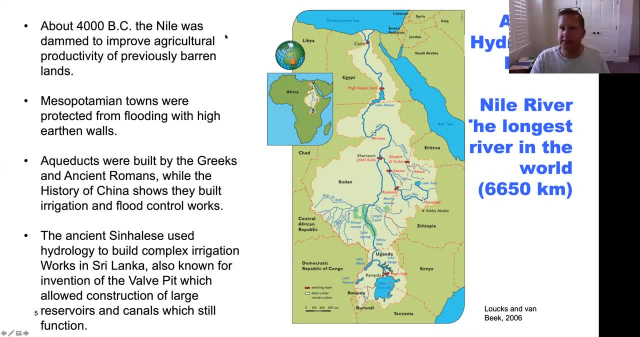 And I think by the time we were done she would have wished she hadn't asked me. You're all welcome to use those talking points. Water resources engineering started 4,000 years BC or more. That's the first known engineering project where the Nile was dammed to improve agricultural productivity in this barren land. 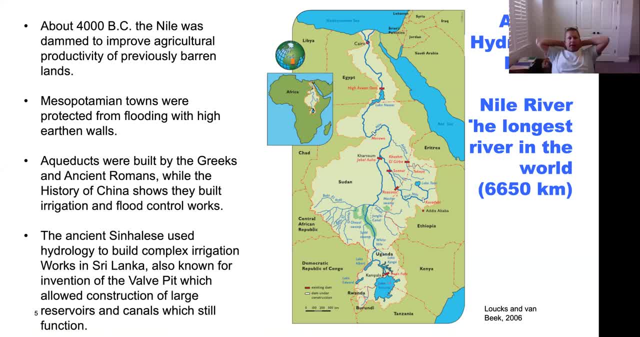 So I'm sure people were damming little streams and stuff before then. But to dam the Nile River was kind of a big deal. And then there was there's flooding in the Mesopotamian towns, the aqueducts built by the Greeks and the Romans. 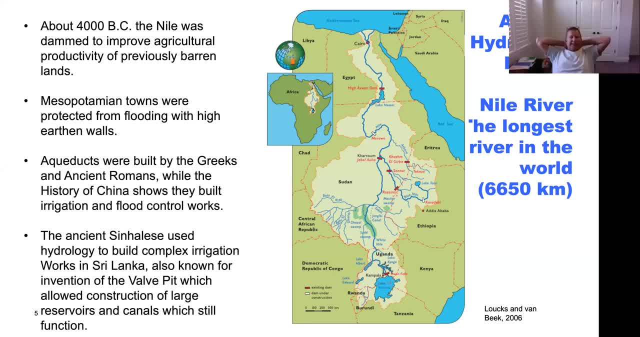 China was building irrigation and flood control works. The Sinalese in Sri Lanka were using hydrology to build rivers, And then the Nile was dammed to improve agricultural productivity in this barren land. So I'm sure people were damming little streams and stuff before then. 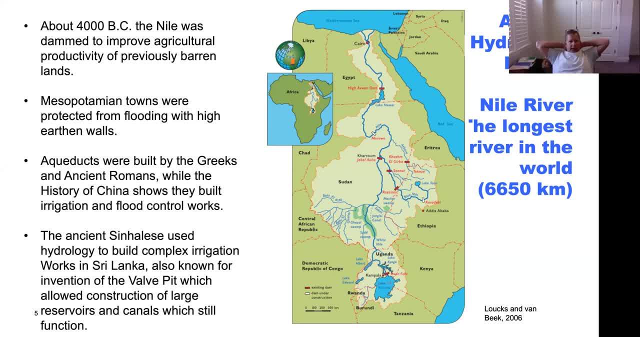 But to dam the Nile was dammed to improve agricultural productivity in this barren land, So I'm sure people were damming little streams and stuff before then. But to dam the Nile was dammed to improve agricultural productivity in this barren land, So I'm sure people were damming little streams and stuff before then. 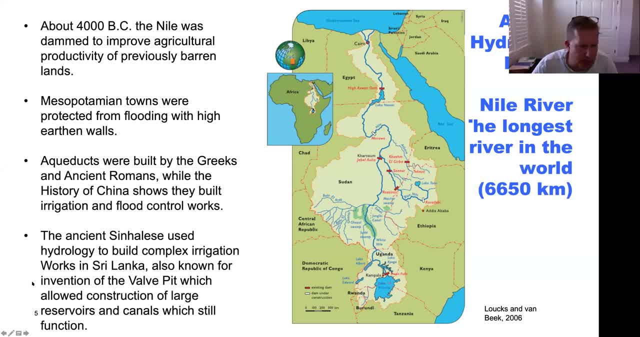 But to dam the Nile was dammed to improve agricultural productivity in this barren land, So I'm sure people were damming little streams and stuff before then. But to dam the Nile was dammed to improve agricultural productivity in this barren land, So I'm sure people were damming little streams and stuff before then. 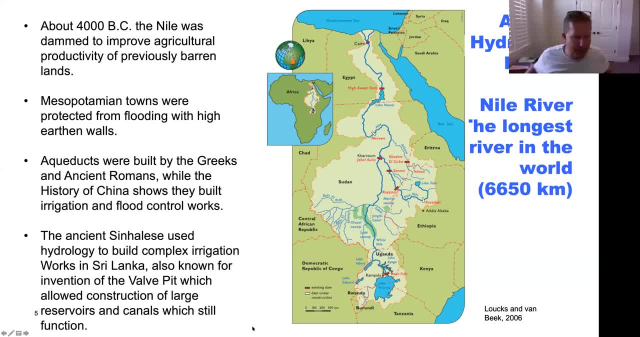 But to dam the Nile was dammed to improve agricultural productivity in this barren land, So I'm sure people were damming little streams and stuff before then. But to dam the Nile was dammed to improve agricultural productivity in this barren land, So I'm sure people were damming little streams and stuff before then. 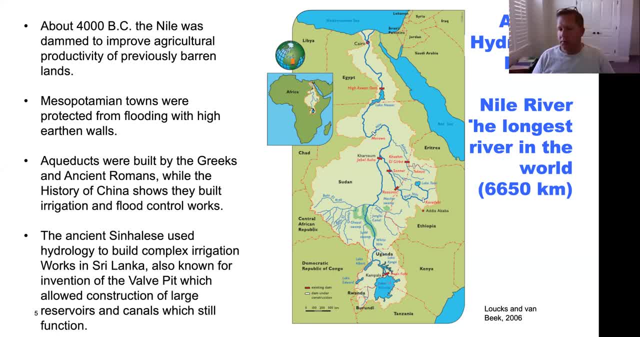 But to dam the Nile was dammed to improve agricultural productivity in this barren land, So I'm sure people were damming little streams and stuff before then. But to dam the Nile was dammed to improve agricultural productivity in this barren land, So I'm sure people were damming little streams and stuff before then. 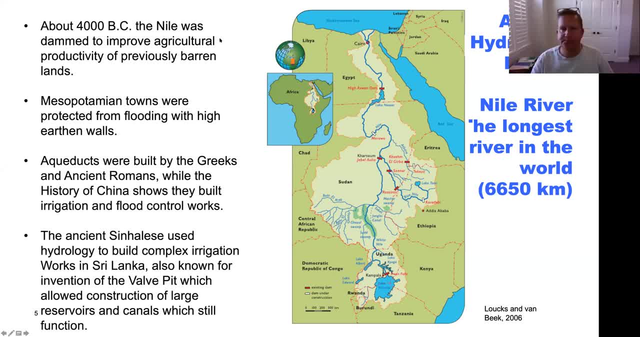 But to dam the Nile was dammed to improve agricultural productivity in this barren land, So I'm sure people were damming little streams and stuff before then. But to dam the Nile was dammed to improve agricultural productivity in this barren land, So I'm sure people were damming little streams and stuff before then. 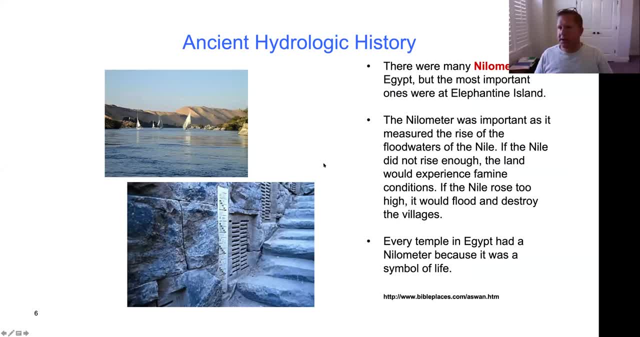 But to dam the Nile was dammed to improve agricultural productivity in this barren land, So I'm sure people were damming little streams and stuff before then. But to dam the Nile was dammed to improve agricultural productivity in this barren land, So I'm sure people were damming little streams and stuff before then. 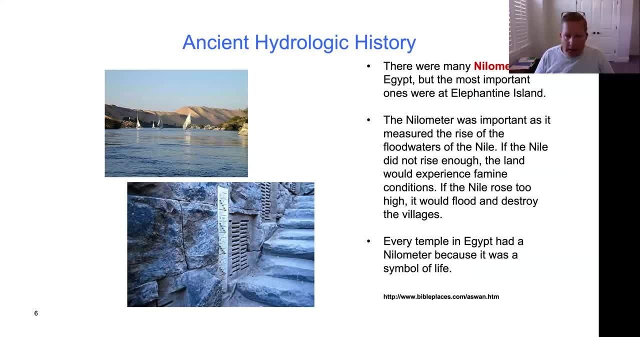 But to dam the Nile was dammed to improve agricultural productivity in this barren land, So I'm sure people were damming little streams and stuff before then. But to dam the Nile was dammed to improve agricultural productivity in this barren land, So I'm sure people were damming little streams and stuff before then. 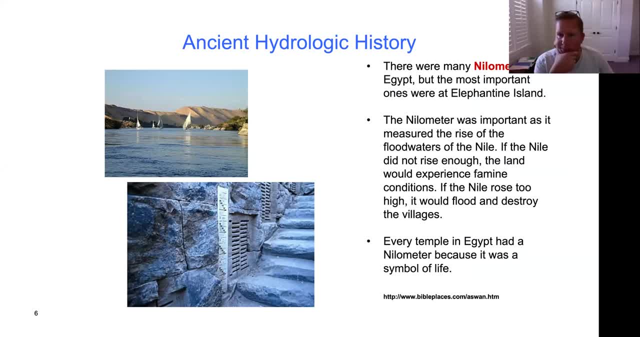 But to dam the Nile was dammed to improve agricultural productivity in this barren land, So I'm sure people were damming little streams and stuff before then. But to dam the Nile was dammed to improve agricultural productivity in this barren land, So I'm sure people were damming little streams and stuff before then. 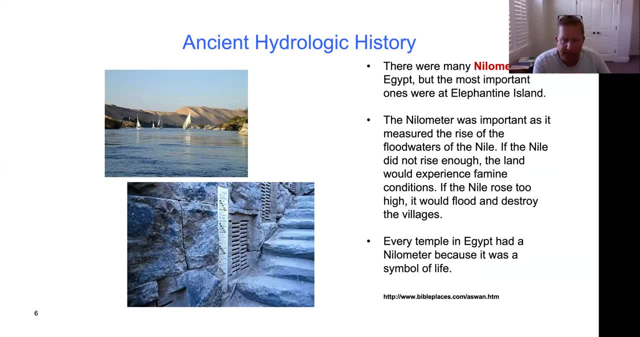 But to dam the Nile was dammed to improve agricultural productivity in this barren land, So I'm sure people were damming little streams and stuff before then. But to dam the Nile was dammed to improve agricultural productivity in this barren land, So I'm sure people were damming little streams and stuff before then. 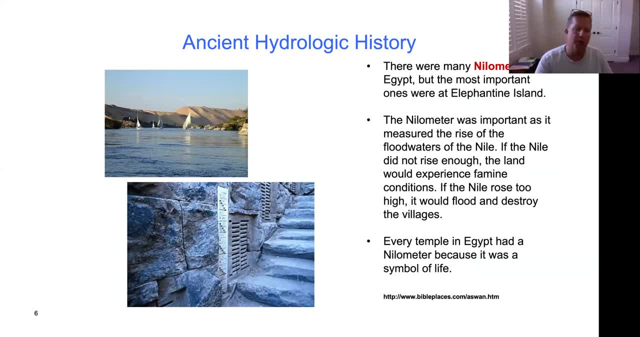 But to dam the Nile was dammed to improve agricultural productivity in this barren land, So I'm sure people were damming little streams and stuff before then. But to dam the Nile was dammed to improve agricultural productivity in this barren land, So I'm sure people were damming little streams and stuff before then. 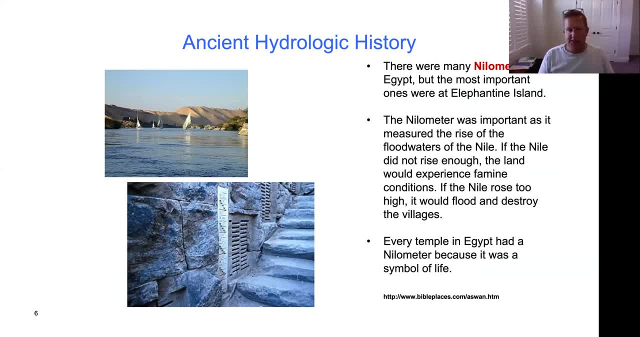 But to dam the Nile was dammed to improve agricultural productivity in this barren land, So I'm sure people were damming little streams and stuff before then. But to dam the Nile was dammed to improve agricultural productivity in this barren land, So I'm sure people were damming little streams and stuff before then. 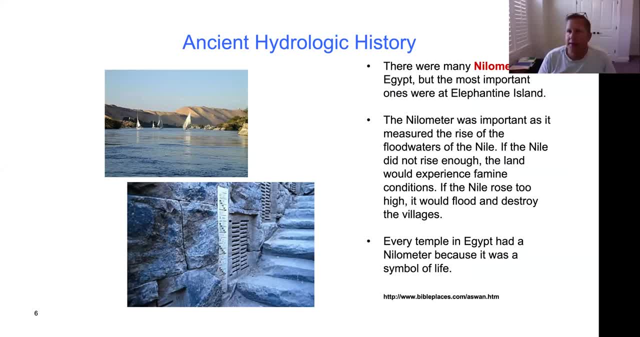 But to dam the Nile was dammed to improve agricultural productivity in this barren land, So I'm sure people were damming little streams and stuff before then. But to dam the Nile was dammed to improve agricultural productivity in this barren land, So I'm sure people were damming little streams and stuff before then. 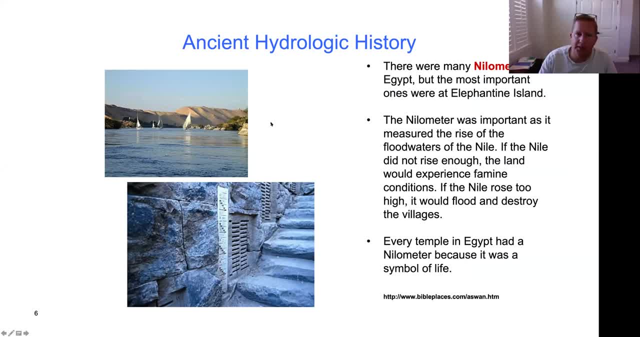 But to dam the Nile was dammed to improve agricultural productivity in this barren land, So I'm sure people were damming little streams and stuff before then. But to dam the Nile was dammed to improve agricultural productivity in this barren land, So I'm sure people were damming little streams and stuff before then. 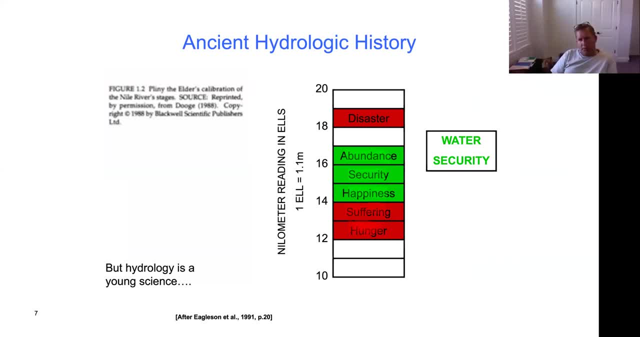 But to dam the Nile was dammed to improve agricultural productivity in this barren land, So I'm sure people were damming little streams and stuff before then. But to dam the Nile was dammed to improve agricultural productivity in this barren land, So I'm sure people were damming little streams and stuff before then. 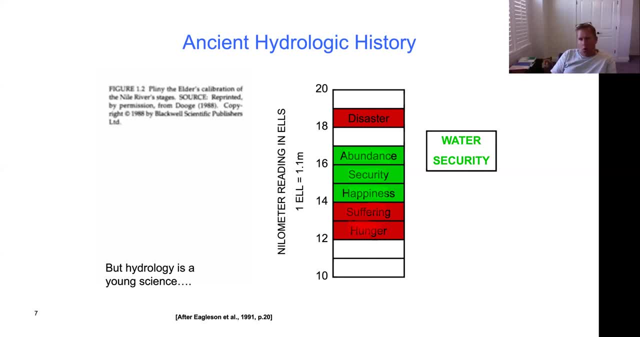 But to dam the Nile was dammed to improve agricultural productivity in this barren land, So I'm sure people were damming little streams and stuff before then. But to dam the Nile was dammed to improve agricultural productivity in this barren land, So I'm sure people were damming little streams and stuff before then. 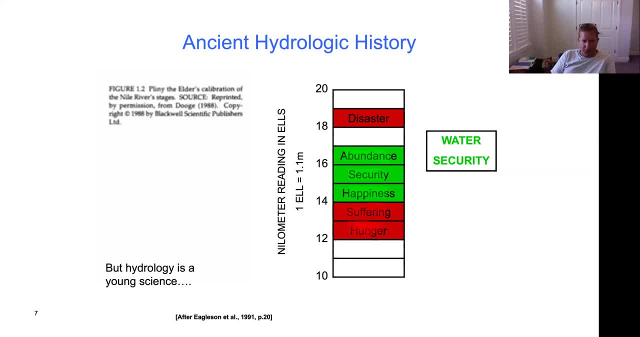 But to dam the Nile was dammed to improve agricultural productivity in this barren land, So I'm sure people were damming little streams and stuff before then. But to dam the Nile was dammed to improve agricultural productivity in this barren land, So I'm sure people were damming little streams and stuff before then. 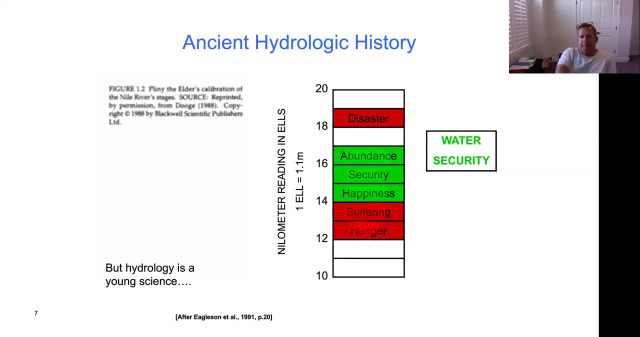 But to dam the Nile was dammed to improve agricultural productivity in this barren land, So I'm sure people were damming little streams and stuff before then. But to dam the Nile was dammed to improve agricultural productivity in this barren land, So I'm sure people were damming little streams and stuff before then. 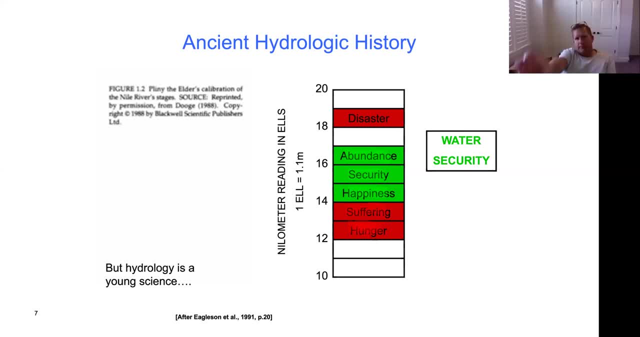 But to dam the Nile was dammed to improve agricultural productivity in this barren land, So I'm sure people were damming little streams and stuff before then. But to dam the Nile was dammed to improve agricultural productivity in this barren land, So I'm sure people were damming little streams and stuff before then. 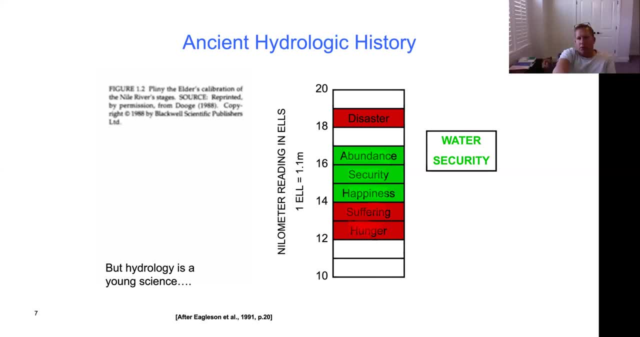 But to dam the Nile was dammed to improve agricultural productivity in this barren land, So I'm sure people were damming little streams and stuff before then. But to dam the Nile was dammed to improve agricultural productivity in this barren land, So I'm sure people were damming little streams and stuff before then. 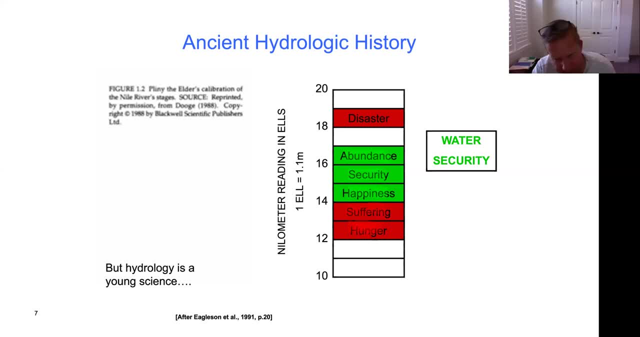 But to dam the Nile was dammed to improve agricultural productivity in this barren land, So I'm sure people were damming little streams and stuff before then. But to dam the Nile was dammed to improve agricultural productivity in this barren land, So I'm sure people were damming little streams and stuff before then. 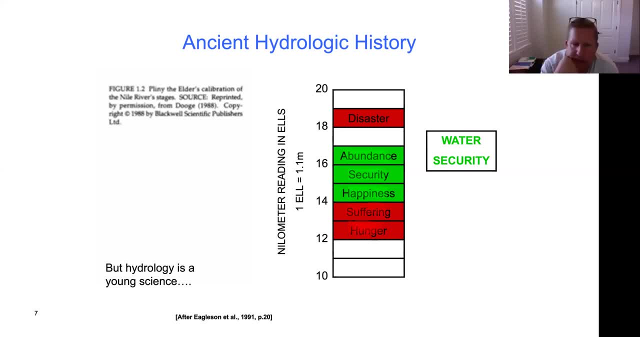 But to dam the Nile was dammed to improve agricultural productivity in this barren land, So I'm sure people were damming little streams and stuff before then. But to dam the Nile was dammed to improve agricultural productivity in this barren land, So I'm sure people were damming little streams and stuff before then. 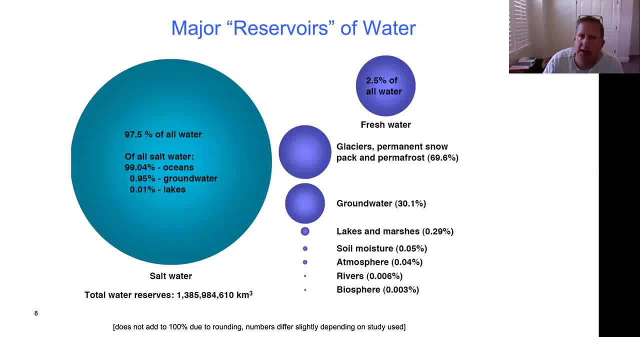 But to dam the Nile was dammed to improve agricultural productivity in this barren land, So I'm sure people were damming little streams and stuff before then. But to dam the Nile was dammed to improve agricultural productivity in this barren land, So I'm sure people were damming little streams and stuff before then. 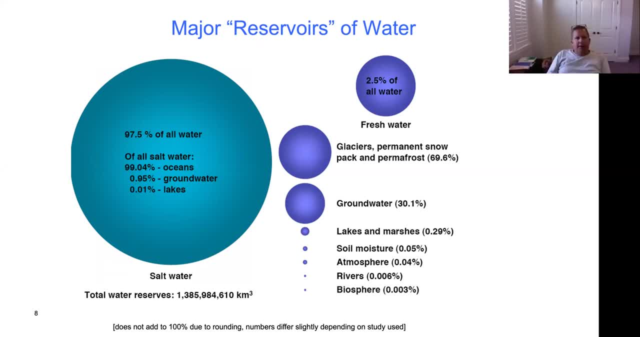 But to dam the Nile was dammed to improve agricultural productivity in this barren land, So I'm sure people were damming little streams and stuff before then. But to dam the Nile was dammed to improve agricultural productivity in this barren land, So I'm sure people were damming little streams and stuff before then. 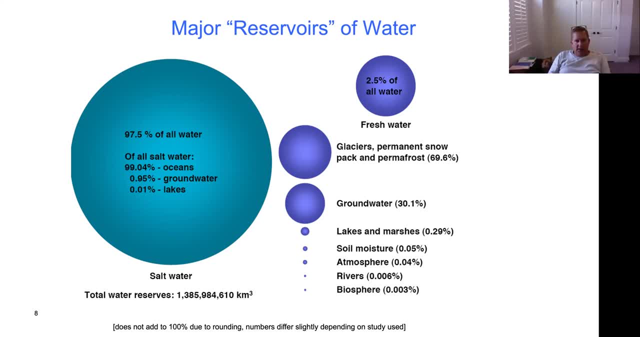 But to dam the Nile was dammed to improve agricultural productivity in this barren land, So I'm sure people were damming little streams and stuff before then. But to dam the Nile was dammed to improve agricultural productivity in this barren land, So I'm sure people were damming little streams and stuff before then. 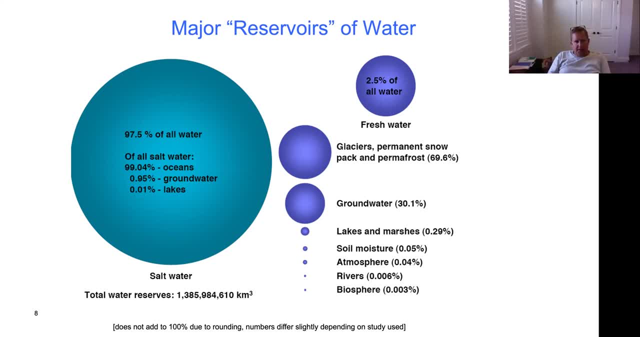 But to dam the Nile was dammed to improve agricultural productivity in this barren land, So I'm sure people were damming little streams and stuff before then. But to dam the Nile was dammed to improve agricultural productivity in this barren land, So I'm sure people were damming little streams and stuff before then. 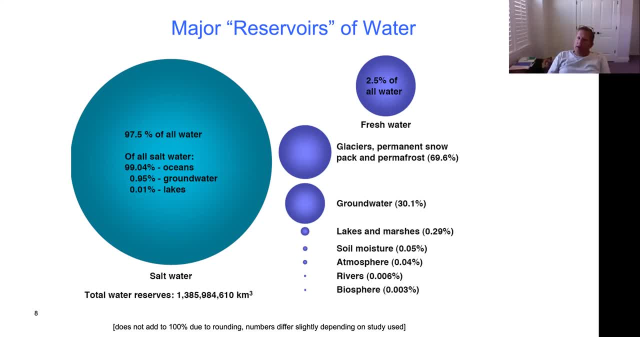 But to dam the Nile was dammed to improve agricultural productivity in this barren land, So I'm sure people were damming little streams and stuff before then. But to dam the Nile was dammed to improve agricultural productivity in this barren land, So I'm sure people were damming little streams and stuff before then. 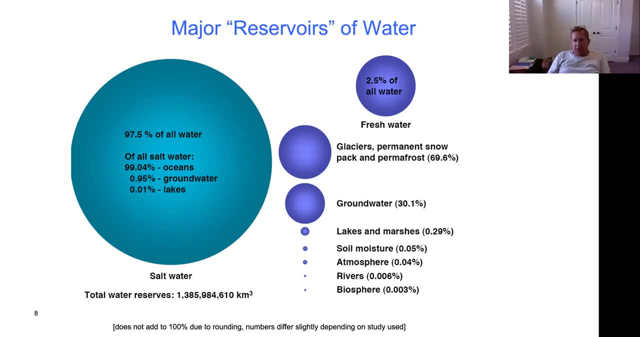 But to dam the Nile was dammed to improve agricultural productivity in this barren land, So I'm sure people were damming little streams and stuff before then. But to dam the Nile was dammed to improve agricultural productivity in this barren land, So I'm sure people were damming little streams and stuff before then. 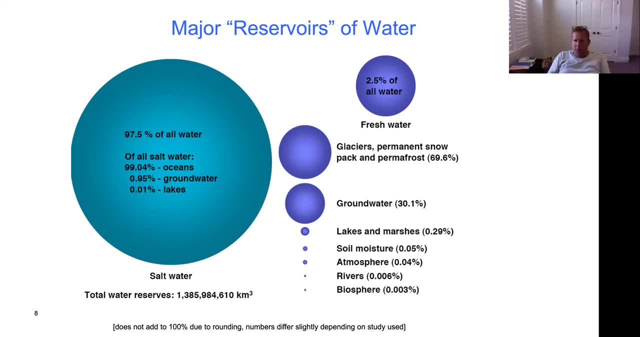 But to dam the Nile was dammed to improve agricultural productivity in this barren land, So I'm sure people were damming little streams and stuff before then. But to dam the Nile was dammed to improve agricultural productivity in this barren land, So I'm sure people were damming little streams and stuff before then. 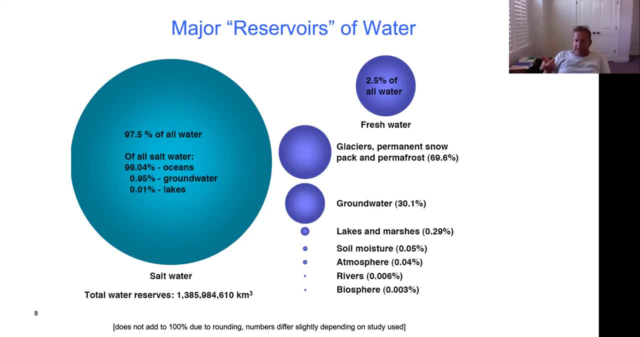 But to dam the Nile was dammed to improve agricultural productivity in this barren land, So I'm sure people were damming little streams and stuff before then. But to dam the Nile was dammed to improve agricultural productivity in this barren land, So I'm sure people were damming little streams and stuff before then. 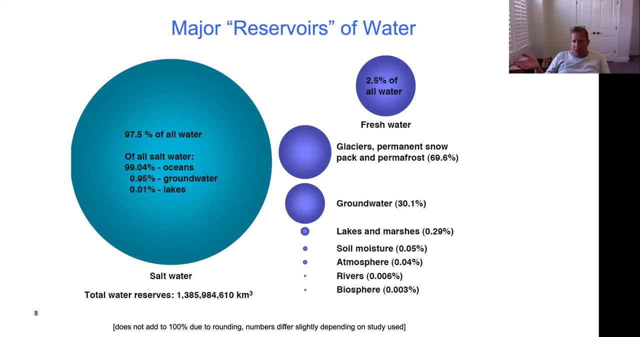 But to dam the Nile was dammed to improve agricultural productivity in this barren land, So I'm sure people were damming little streams and stuff before then. But to dam the Nile was dammed to improve agricultural productivity in this barren land, So I'm sure people were damming little streams and stuff before then. 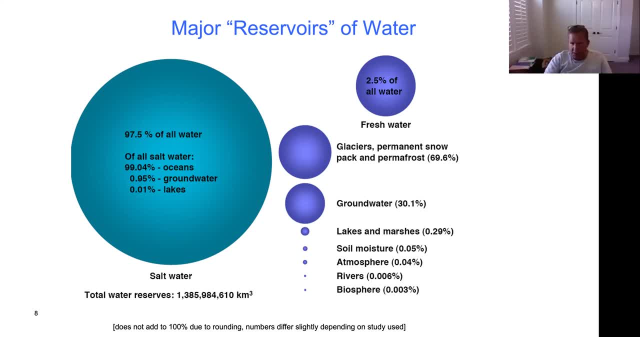 But to dam the Nile was dammed to improve agricultural productivity in this barren land, So I'm sure people were damming little streams and stuff before then. But to dam the Nile was dammed to improve agricultural productivity in this barren land, So I'm sure people were damming little streams and stuff before then. 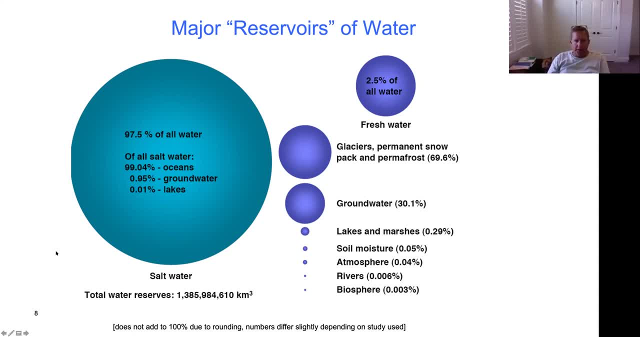 But to dam the Nile was dammed to improve agricultural productivity in this barren land, So I'm sure people were damming little streams and stuff before then. But to dam the Nile was dammed to improve agricultural productivity in this barren land, So I'm sure people were damming little streams and stuff before then. 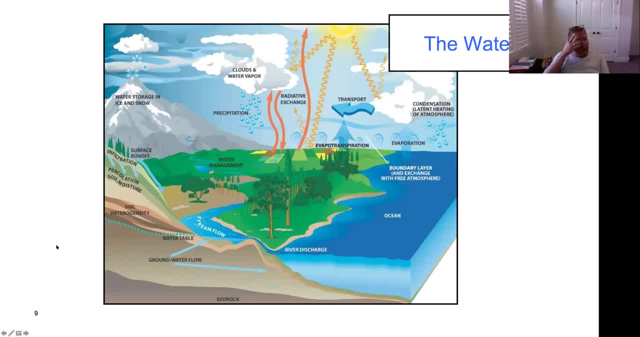 But to dam the Nile was dammed to improve agricultural productivity in this barren land, So I'm sure people were damming little streams and stuff before then. But to dam the Nile was dammed to improve agricultural productivity in this barren land, So I'm sure people were damming little streams and stuff before then. 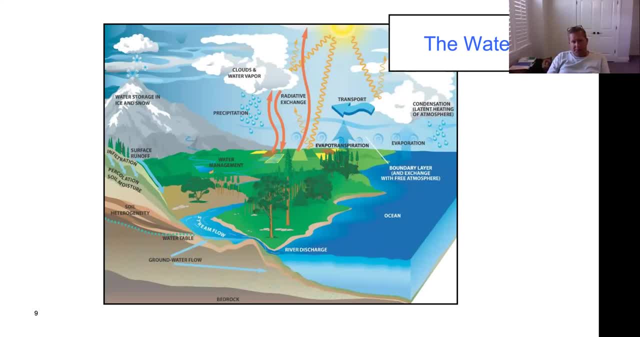 But to dam the Nile was dammed to improve agricultural productivity in this barren land, So I'm sure people were damming little streams and stuff before then. But to dam the Nile was dammed to improve agricultural productivity in this barren land, So I'm sure people were damming little streams and stuff before then. 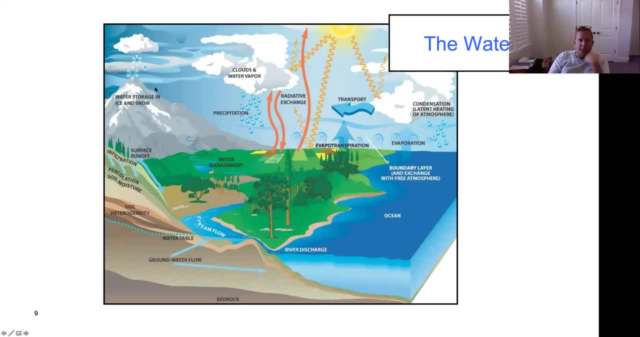 But to dam the Nile was dammed to improve agricultural productivity in this barren land, So I'm sure people were damming little streams and stuff before then. But to dam the Nile was dammed to improve agricultural productivity in this barren land, So I'm sure people were damming little streams and stuff before then. 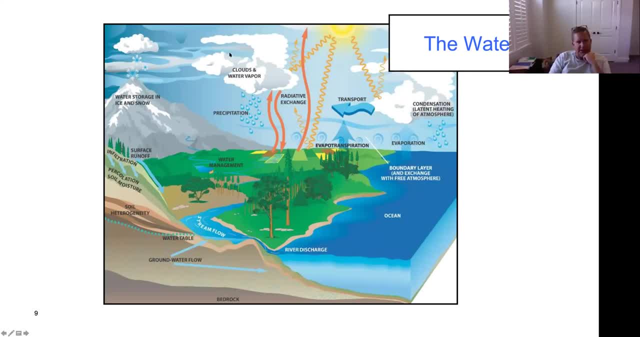 But to dam the Nile was dammed to improve agricultural productivity in this barren land, So I'm sure people were damming little streams and stuff before then. But to dam the Nile was dammed to improve agricultural productivity in this barren land, So I'm sure people were damming little streams and stuff before then. 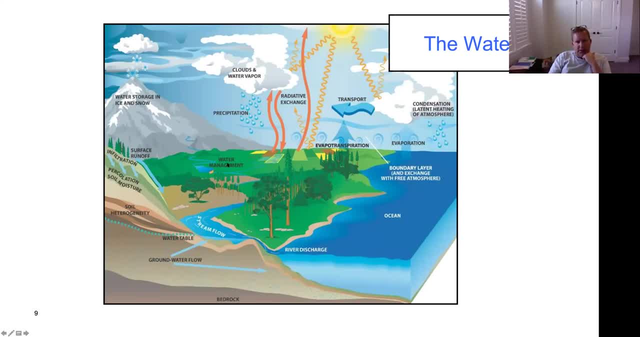 But to dam the Nile was dammed to improve agricultural productivity in this barren land, So I'm sure people were damming little streams and stuff before then. But to dam the Nile was dammed to improve agricultural productivity in this barren land, So I'm sure people were damming little streams and stuff before then. 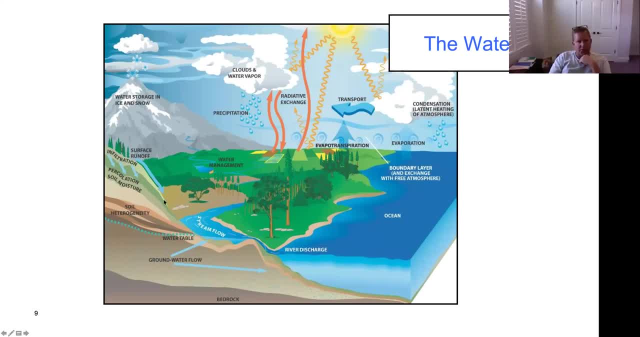 But to dam the Nile was dammed to improve agricultural productivity in this barren land, So I'm sure people were damming little streams and stuff before then. But to dam the Nile was dammed to improve agricultural productivity in this barren land, So I'm sure people were damming little streams and stuff before then. 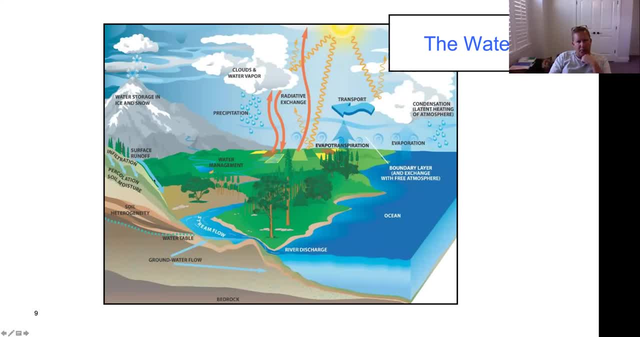 But to dam the Nile was dammed to improve agricultural productivity in this barren land, So I'm sure people were damming little streams and stuff before then. But to dam the Nile was dammed to improve agricultural productivity in this barren land, So I'm sure people were damming little streams and stuff before then. 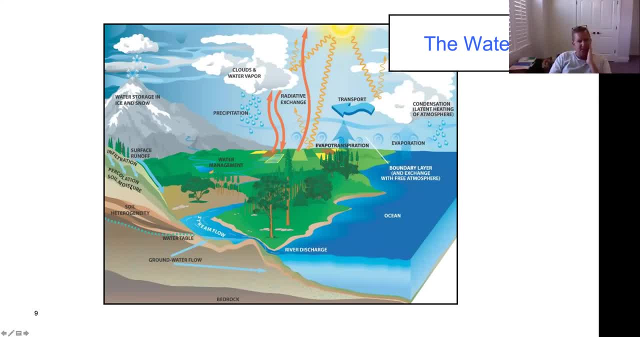 But to dam the Nile was dammed to improve agricultural productivity in this barren land, So I'm sure people were damming little streams and stuff before then. But to dam the Nile was dammed to improve agricultural productivity in this barren land, So I'm sure people were damming little streams and stuff before then. 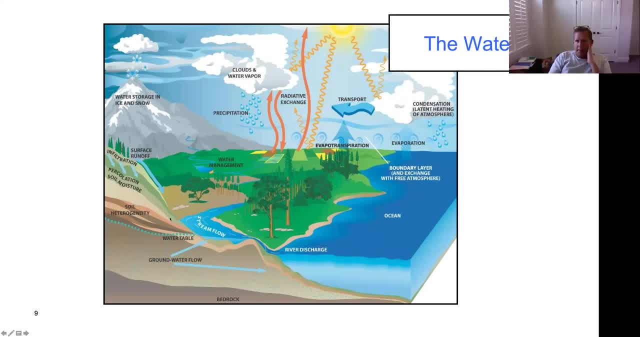 But to dam the Nile was dammed to improve agricultural productivity in this barren land, So I'm sure people were damming little streams and stuff before then. But to dam the Nile was dammed to improve agricultural productivity in this barren land, So I'm sure people were damming little streams and stuff before then. 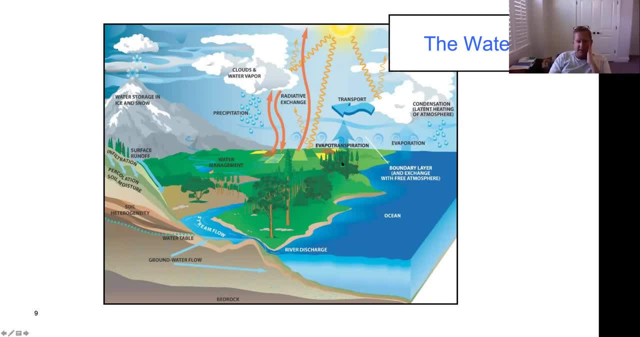 But to dam the Nile was dammed to improve agricultural productivity in this barren land, So I'm sure people were damming little streams and stuff before then. But to dam the Nile was dammed to improve agricultural productivity in this barren land, So I'm sure people were damming little streams and stuff before then. 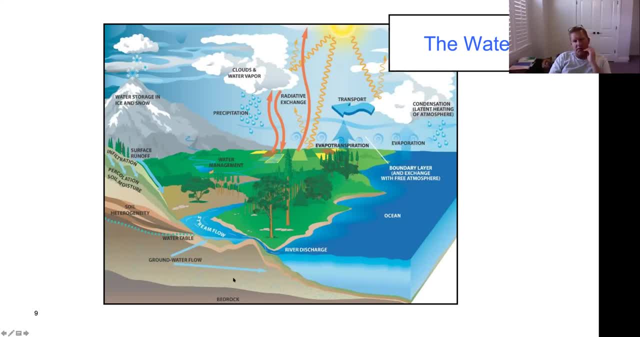 But to dam the Nile was dammed to improve agricultural productivity in this barren land, So I'm sure people were damming little streams and stuff before then. But to dam the Nile was dammed to improve agricultural productivity in this barren land, So I'm sure people were damming little streams and stuff before then. 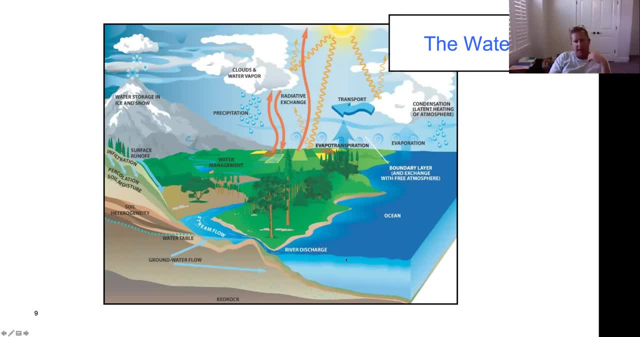 But to dam the Nile was dammed to improve agricultural productivity in this barren land, So I'm sure people were damming little streams and stuff before then. But to dam the Nile was dammed to improve agricultural productivity in this barren land, So I'm sure people were damming little streams and stuff before then. 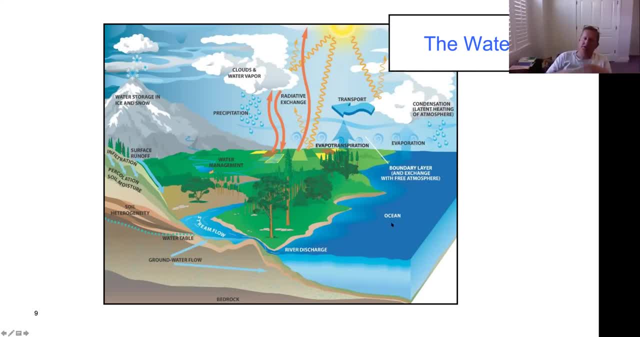 But to dam the Nile was dammed to improve agricultural productivity in this barren land, So I'm sure people were damming little streams and stuff before then. But to dam the Nile was dammed to improve agricultural productivity in this barren land, So I'm sure people were damming little streams and stuff before then. 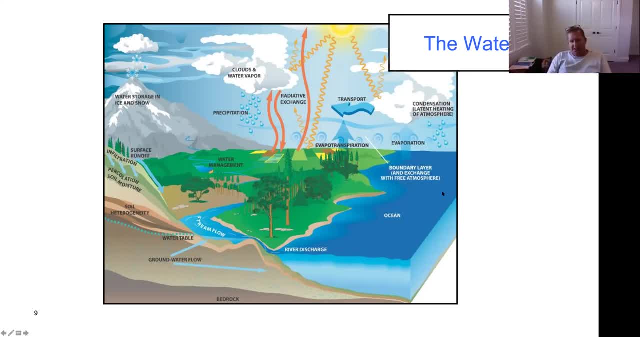 But to dam the Nile was dammed to improve agricultural productivity in this barren land, So I'm sure people were damming little streams and stuff before then. But to dam the Nile was dammed to improve agricultural productivity in this barren land, So I'm sure people were damming little streams and stuff before then. 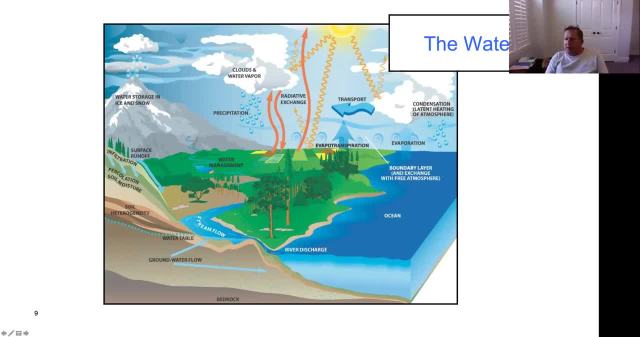 But to dam the Nile was dammed to improve agricultural productivity in this barren land, So I'm sure people were damming little streams and stuff before then. But to dam the Nile was dammed to improve agricultural productivity in this barren land, So I'm sure people were damming little streams and stuff before then. 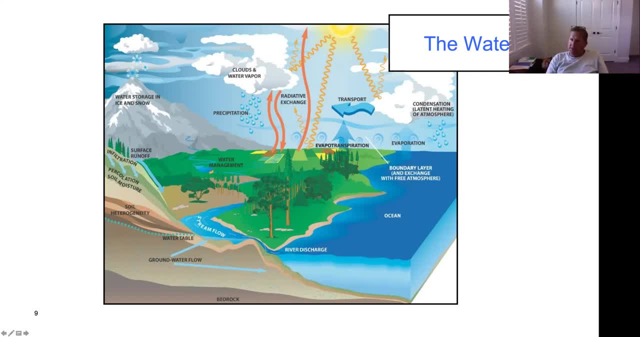 But to dam the Nile was dammed to improve agricultural productivity in this barren land, So I'm sure people were damming little streams and stuff before then. But to dam the Nile was dammed to improve agricultural productivity in this barren land, So I'm sure people were damming little streams and stuff before then. 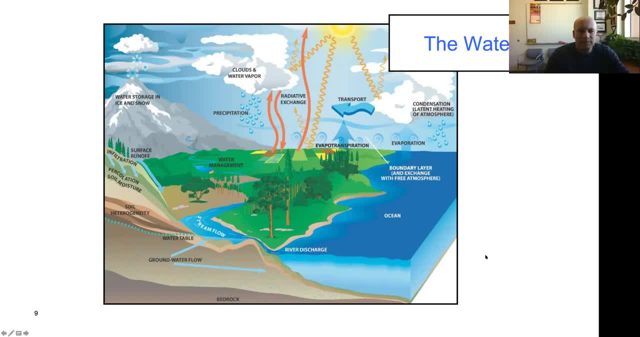 But to dam the Nile was dammed to improve agricultural productivity in this barren land, So I'm sure people were damming little streams and stuff before then. But to dam the Nile was dammed to improve agricultural productivity in this barren land, So I'm sure people were damming little streams and stuff before then. 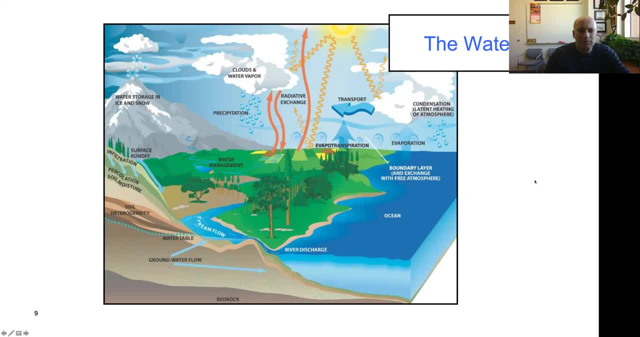 But to dam the Nile was dammed to improve agricultural productivity in this barren land, So I'm sure people were damming little streams and stuff before then. But to dam the Nile was dammed to improve agricultural productivity in this barren land, So I'm sure people were damming little streams and stuff before then. 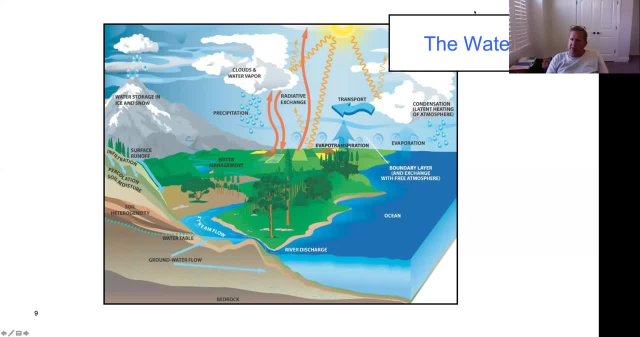 But to dam the Nile was dammed to improve agricultural productivity in this barren land, So I'm sure people were damming little streams and stuff before then. But to dam the Nile was dammed to improve agricultural productivity in this barren land, So I'm sure people were damming little streams and stuff before then. 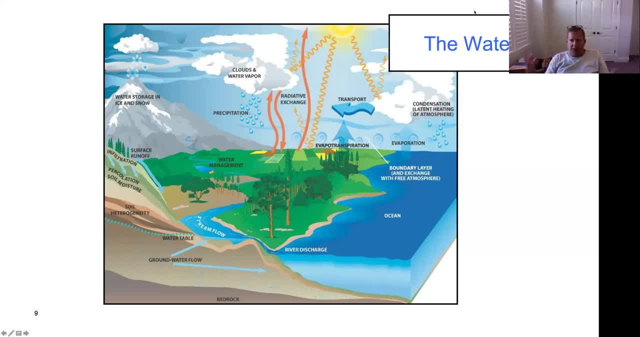 But to dam the Nile was dammed to improve agricultural productivity in this barren land, So I'm sure people were damming little streams and stuff before then. But to dam the Nile was dammed to improve agricultural productivity in this barren land, So I'm sure people were damming little streams and stuff before then. 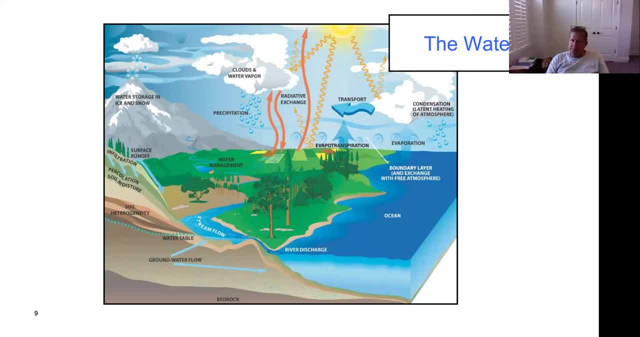 But to dam the Nile was dammed to improve agricultural productivity in this barren land, So I'm sure people were damming little streams and stuff before then. But to dam the Nile was dammed to improve agricultural productivity in this barren land, So I'm sure people were damming little streams and stuff before then. 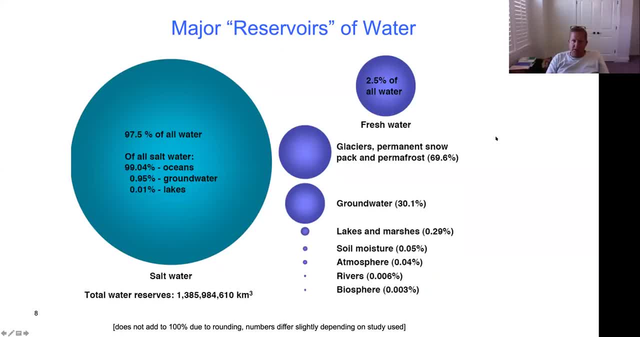 But to dam the Nile was dammed to improve agricultural productivity in this barren land, So I'm sure people were damming little streams and stuff before then. But to dam the Nile was dammed to improve agricultural productivity in this barren land, So I'm sure people were damming little streams and stuff before then. 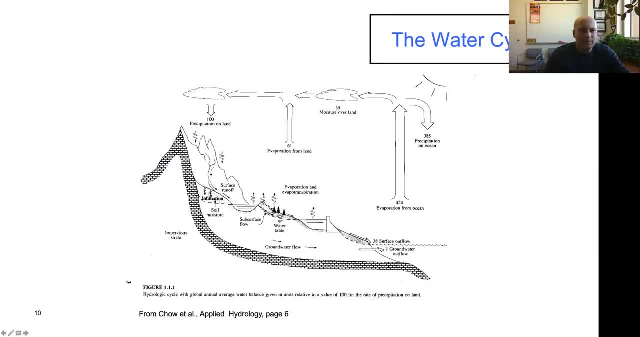 But to dam the Nile was dammed to improve agricultural productivity in this barren land, So I'm sure people were damming little streams and stuff before then. But to dam the Nile was dammed to improve agricultural productivity in this barren land, So I'm sure people were damming little streams and stuff before then. But to dam the Nile was dammed to improve agricultural productivity in this barren land, So I'm sure people were damming little streams and stuff before then. But to dam the Nile was dammed to improve agricultural productivity in this barren land, So I'm sure people were damming little streams and stuff before then. 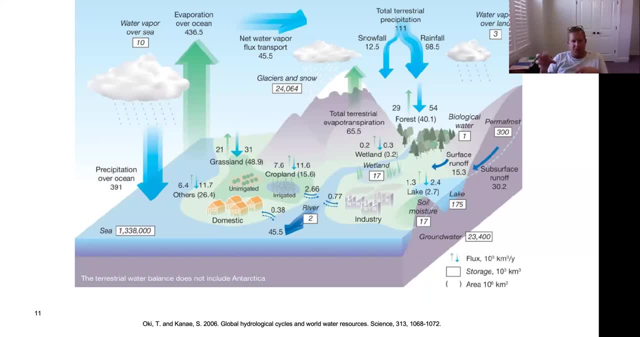 But to dam the Nile was dammed to improve agricultural productivity in this barren land, So I'm sure people were damming little streams and stuff before then. But to dam the Nile was dammed to improve agricultural productivity in this barren land, So I'm sure people were damming little streams and stuff before then. 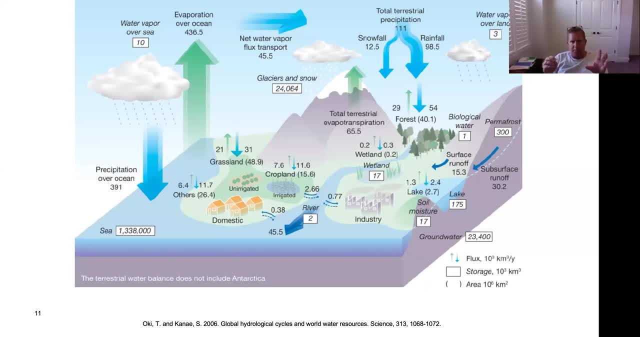 But to dam the Nile was dammed to improve agricultural productivity in this barren land, So I'm sure people were damming little streams and stuff before then. But to dam the Nile was dammed to improve agricultural productivity in this barren land, So I'm sure people were damming little streams and stuff before then. But to dam the Nile was dammed to improve agricultural productivity in this barren land, So I'm sure people were damming little streams and stuff before then. But to dam the Nile was dammed to improve agricultural productivity in this barren land, So I'm sure people were damming little streams and stuff before then. 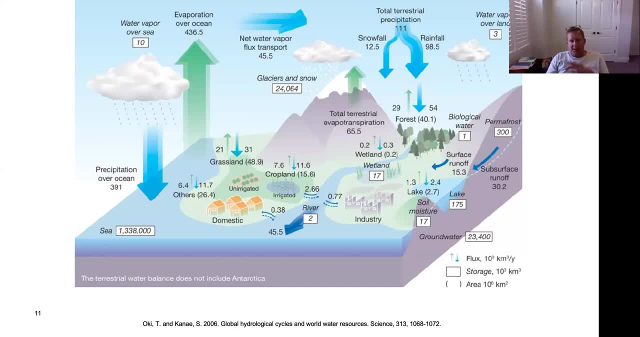 But to dam the Nile was dammed to improve agricultural productivity in this barren land, So I'm sure people were damming little streams and stuff before then. But to dam the Nile was dammed to improve agricultural productivity in this barren land, So I'm sure people were damming little streams and stuff before then. 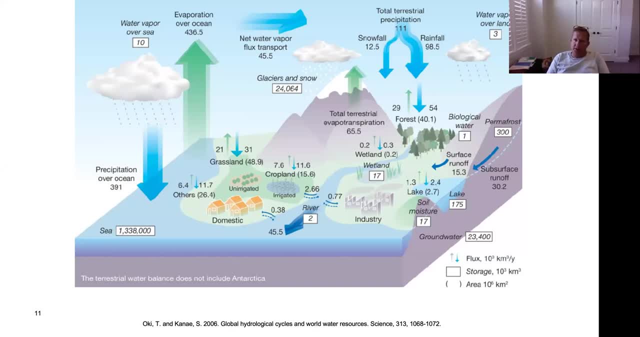 But to dam the Nile was dammed to improve agricultural productivity in this barren land, So I'm sure people were damming little streams and stuff before then. But to dam the Nile was dammed to improve agricultural productivity in this barren land, So I'm sure people were damming little streams and stuff before then. But to dam the Nile was dammed to improve agricultural productivity in this barren land, So I'm sure people were damming little streams and stuff before then. But to dam the Nile was dammed to improve agricultural productivity in this barren land, So I'm sure people were damming little streams and stuff before then. 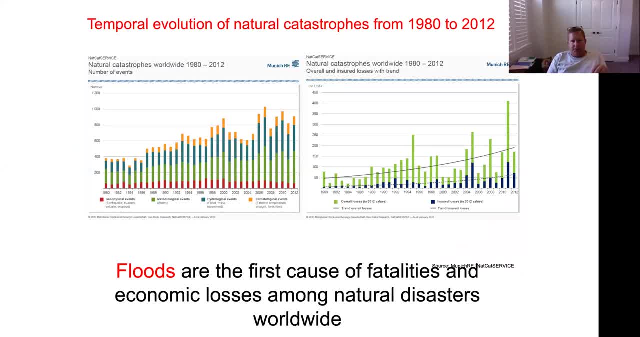 But to dam the Nile was dammed to improve agricultural productivity in this barren land, So I'm sure people were damming little streams and stuff before then. But to dam the Nile was dammed to improve agricultural productivity in this barren land, So I'm sure people were damming little streams and stuff before then. 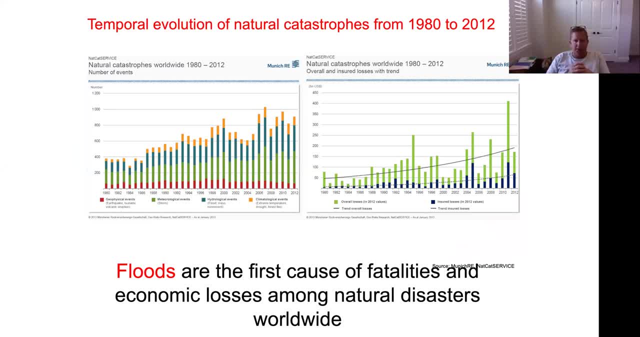 But to dam the Nile was dammed to improve agricultural productivity in this barren land, So I'm sure people were damming little streams and stuff before then. But to dam the Nile was dammed to improve agricultural productivity in this barren land, So I'm sure people were damming little streams and stuff before then. 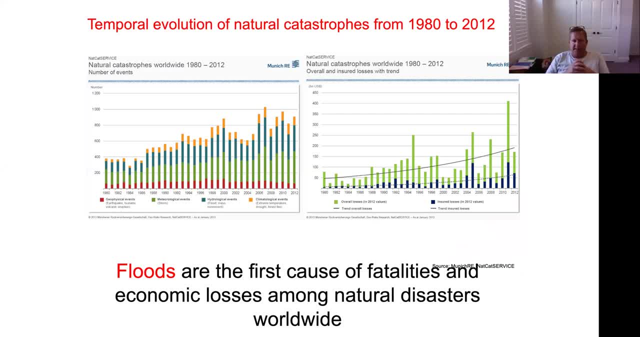 But to dam the Nile was dammed to improve agricultural productivity in this barren land, So I'm sure people were damming little streams and stuff before then. But to dam the Nile was dammed to improve agricultural productivity in this barren land, So I'm sure people were damming little streams and stuff before then. 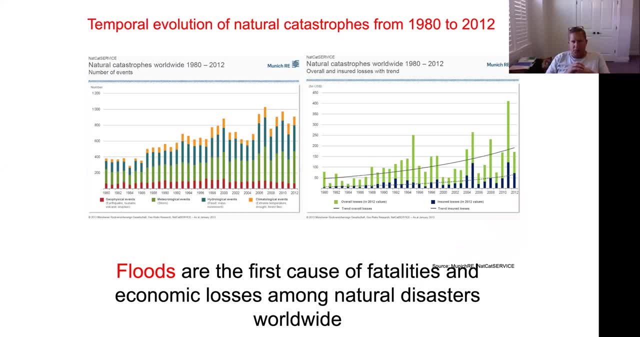 But to dam the Nile was dammed to improve agricultural productivity in this barren land, So I'm sure people were damming little streams and stuff before then. But to dam the Nile was dammed to improve agricultural productivity in this barren land, So I'm sure people were damming little streams and stuff before then. 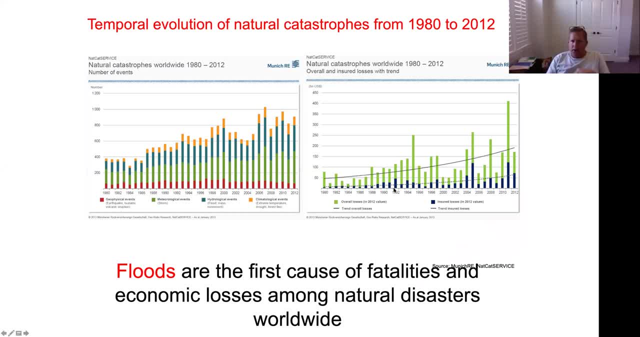 But to dam the Nile was dammed to improve agricultural productivity in this barren land, So I'm sure people were damming little streams and stuff before then. But to dam the Nile was dammed to improve agricultural productivity in this barren land, So I'm sure people were damming little streams and stuff before then. 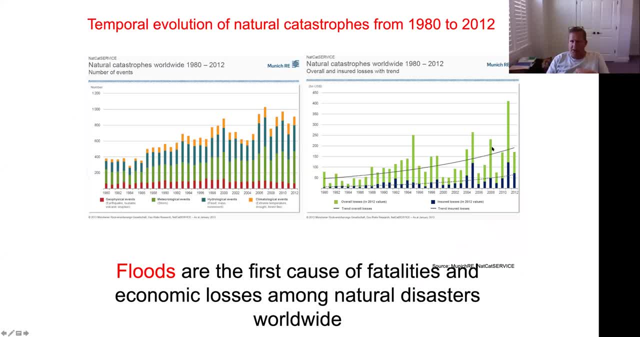 But to dam the Nile was dammed to improve agricultural productivity in this barren land, So I'm sure people were damming little streams and stuff before then. But to dam the Nile was dammed to improve agricultural productivity in this barren land, So I'm sure people were damming little streams and stuff before then. 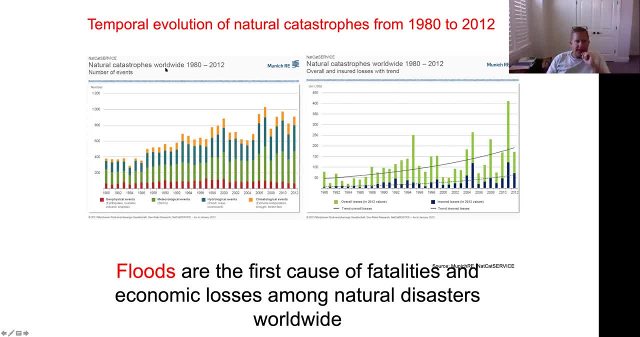 But to dam the Nile was dammed to improve agricultural productivity in this barren land, So I'm sure people were damming little streams and stuff before then. But to dam the Nile was dammed to improve agricultural productivity in this barren land, So I'm sure people were damming little streams and stuff before then. 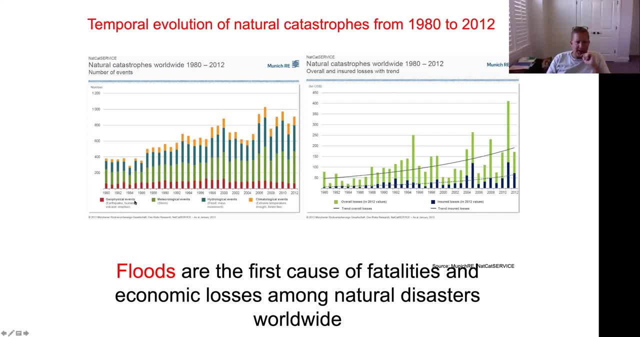 But to dam the Nile was dammed to improve agricultural productivity in this barren land, So I'm sure people were damming little streams and stuff before then. But to dam the Nile was dammed to improve agricultural productivity in this barren land, So I'm sure people were damming little streams and stuff before then. 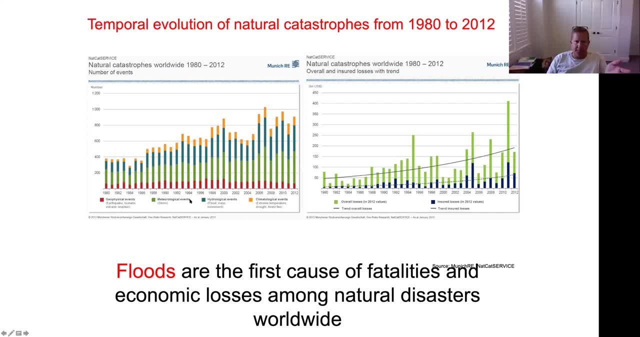 But to dam the Nile was dammed to improve agricultural productivity in this barren land, So I'm sure people were damming little streams and stuff before then. But to dam the Nile was dammed to improve agricultural productivity in this barren land, So I'm sure people were damming little streams and stuff before then. 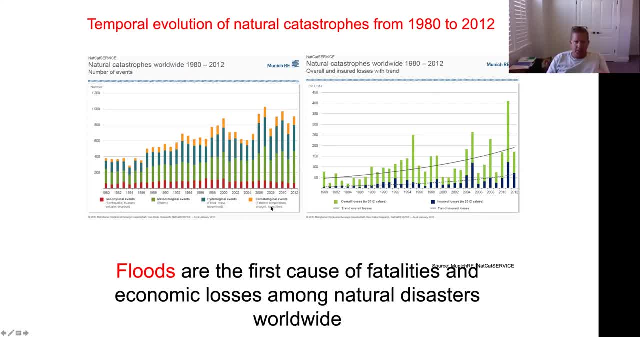 But to dam the Nile was dammed to improve agricultural productivity in this barren land, So I'm sure people were damming little streams and stuff before then. But to dam the Nile was dammed to improve agricultural productivity in this barren land, So I'm sure people were damming little streams and stuff before then. 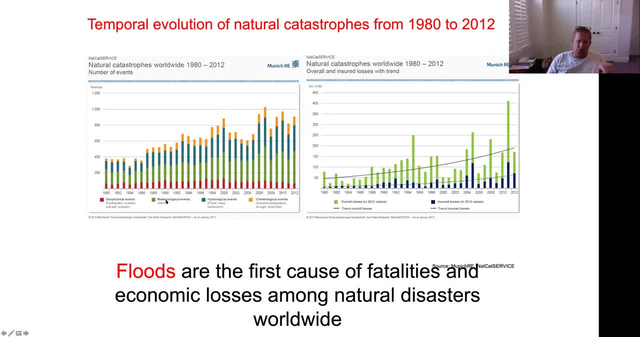 But to dam the Nile was dammed to improve agricultural productivity in this barren land, So I'm sure people were damming little streams and stuff before then. But to dam the Nile was dammed to improve agricultural productivity in this barren land, So I'm sure people were damming little streams and stuff before then. 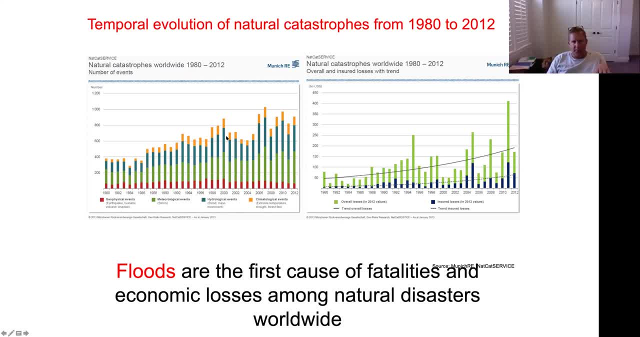 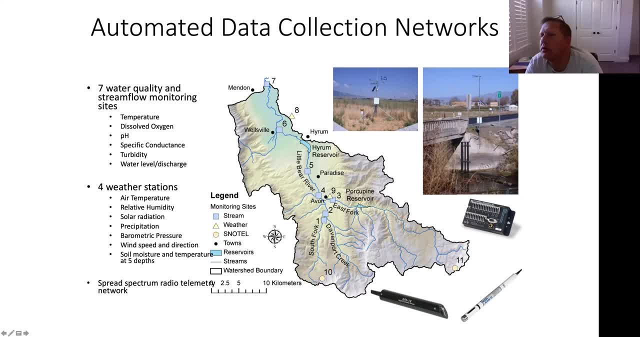 see a hand go or a hand go up. i can't see who it is, though. ian hua, do you have a question? i think everyone's just got their hands up for a roll. okay, still, we're just saying we're here. yeah, we're here, we're here, don't forget me. so when jeff started putting in all this equipment, he 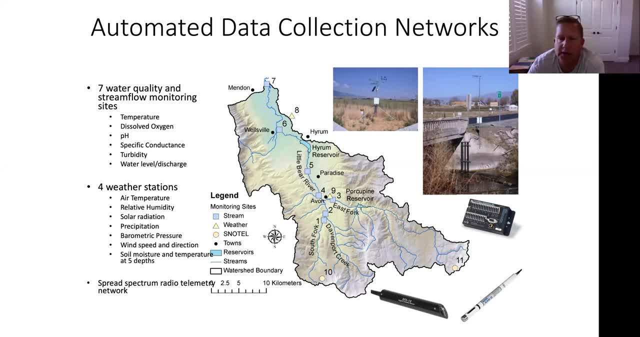 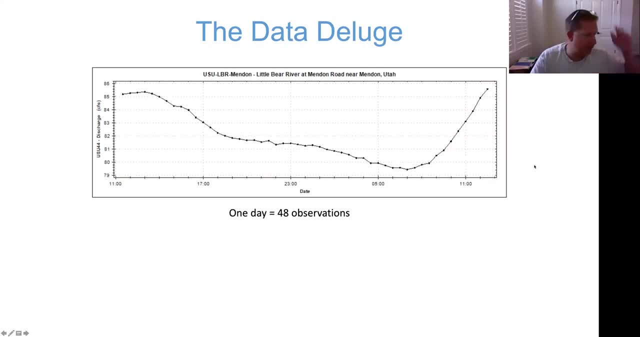 built little radio sensors in there and he could transmit the water quality and the water information from that sensor to a central tower. and then they start collecting it and we start developing something called the data deluge. the term deluge is a water term, obviously for a 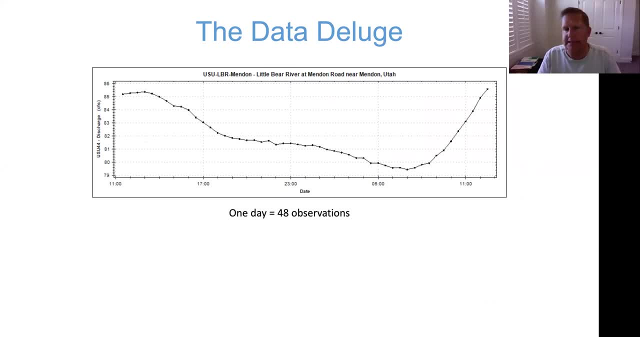 pun, and a purposeful pun. a data deluge is what happens when you collect water measurements. with a little sensor out in the river like this is measuring flow in cubic feet per second in a river channel and it looks like over one day he's measuring the flow 48. 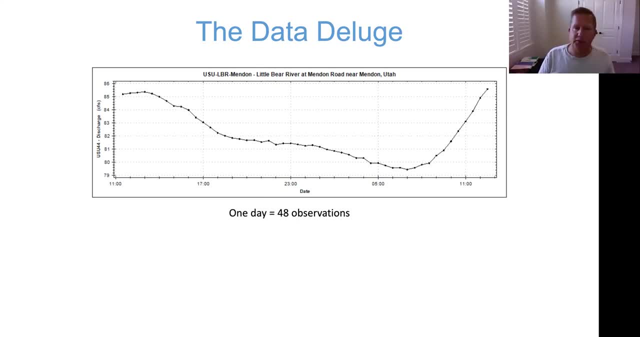 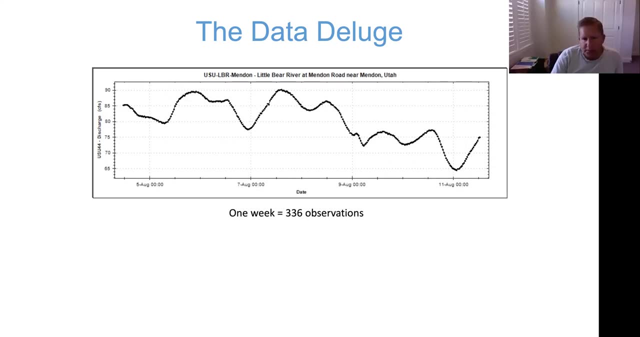 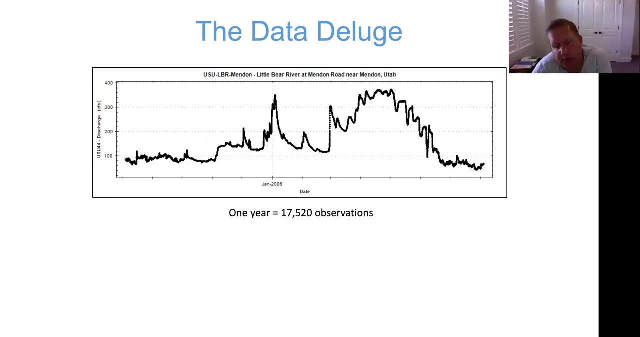 different times to see how fast, how much water is flowing down the channel. at the little bear river, at mendon road near mendon utah, in a week he gets 336 observations and he gets a lot more in a year: 17 000 observations. so the the field of hydroinformatics is: how do 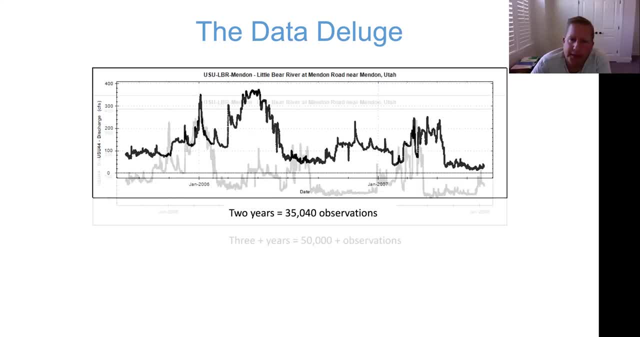 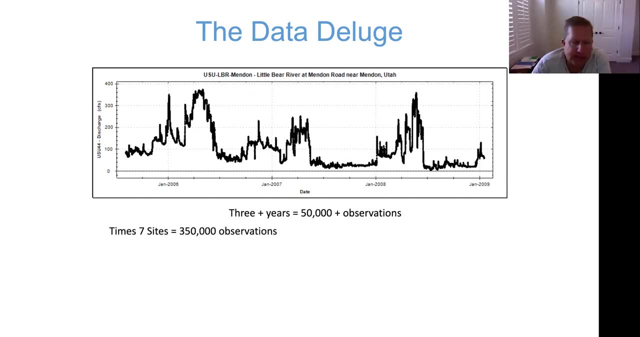 you collect this data and then what do you do with it and how can you make sense of it? in three years he's got 50 000 observations at that one station, but he has seven sites and he has 10 variables at each site- that where he's collecting information. so he wants to know. 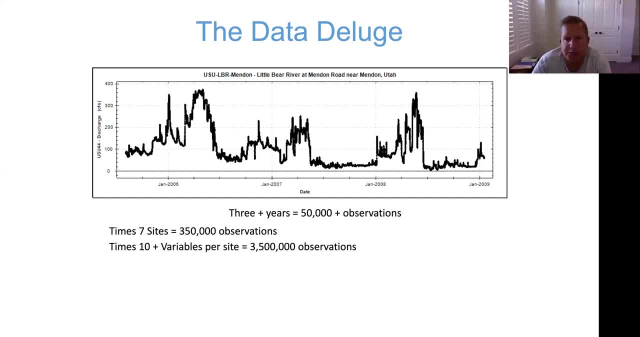 like not just how fast, how much water is flowing, but what's the temperature of the water, how much dissolved oxygen is in the water, a lot of things that he can sense from these probes that he's put in the river. so he's um, he's got, depending on what data is looking at, over seven million observations. 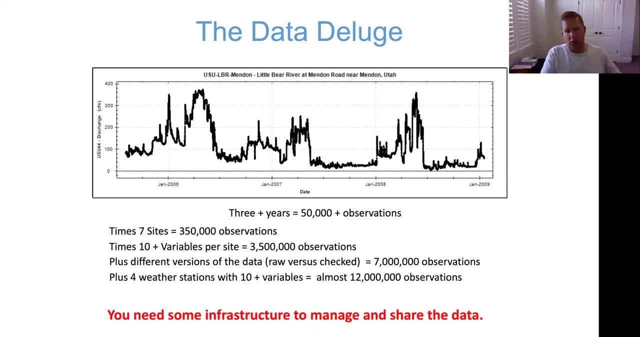 in just a few years. and if you bring in the weather stations you get up to 12 million observations. so suddenly you have more than you can just type into an spreadsheet and make a cute little graph in Excel and look at and make sense of. So that's where we have to start building databases and using cloud. 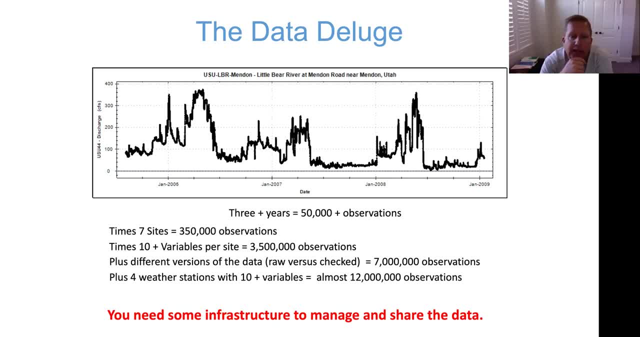 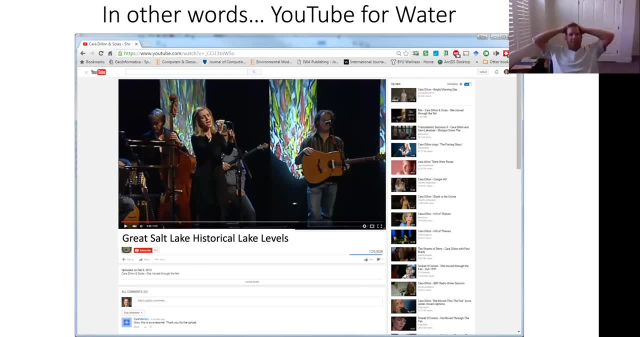 computing and using machine learning and artificial neural networks to analyze the data, try to make sense of it and determine, basically determine you know what's going on in the river and if there's a problem, if we're going to be flooding, if we're going to have water quality issues, etc. In one way to one way that 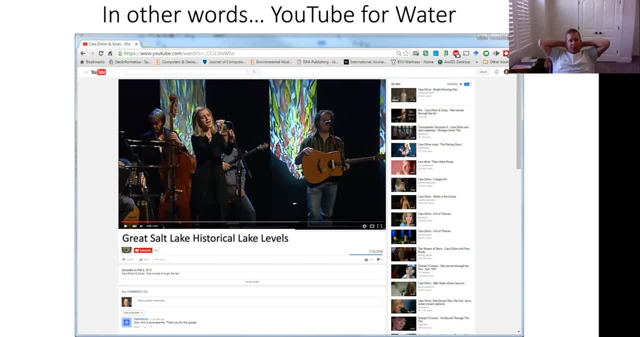 we here at BYU have worked to address this problem has been to build a software system called HydroShare, HydroSharecom, HydroShare, excuse me, org, HydroShareorg. It's sort of like a YouTube for water, meaning that it's a place where people can stick information, just like you can stick a. 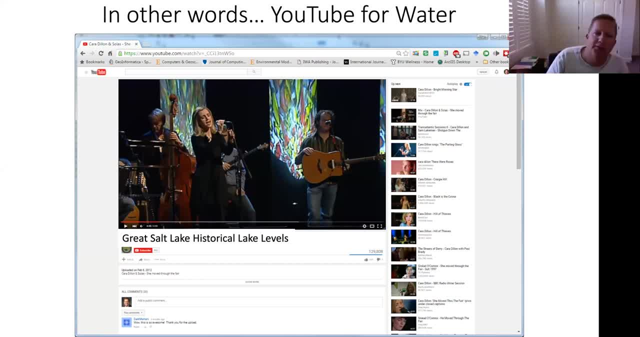 video up on YouTube. people can stick water data up on HydroShare. So instead of that singer, it's now this chart. And it's not just a chart, it's the rod chart. So, instead of that singer, it's now this chart. And it's not just a chart, it's the rod chart. 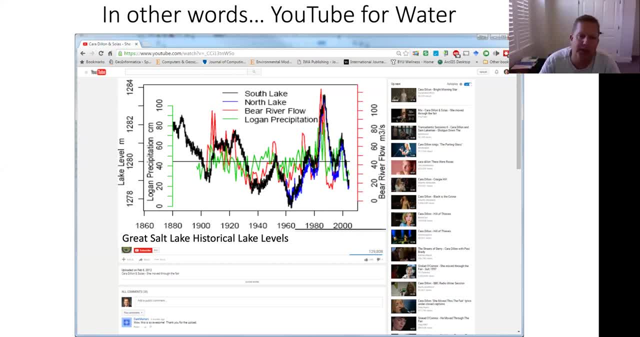 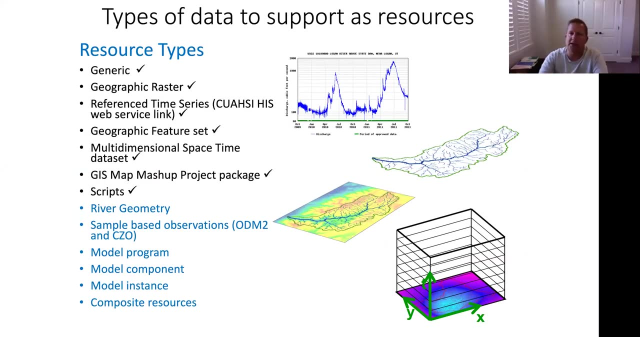 So instead of that singer, it's now this chart And it's the rod chart, So you can put up data and it's information about the data. You can put up gigabytes of data. You can store it out here. Instead of having all kinds of YouTube videos, you can have access to all kinds of water data. And I've just got these charts in here just as a rough idea to show you a little bit of the concept behind HydroShare. But really HydroShare is taking not just chart data like that, but also spatial data like where are the river networks and stuff like this heat map and elevation maps and three-dimensional data, and putting it all in a system. This is actually HydroShare. 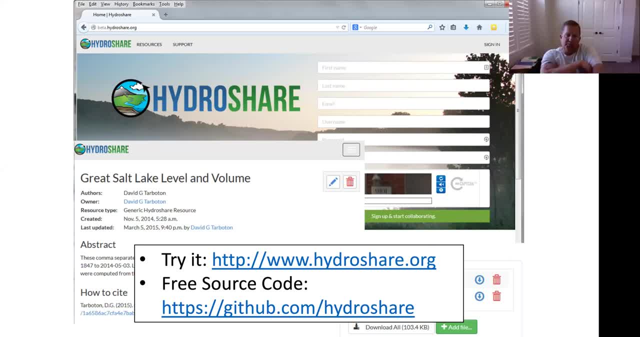 So this is one of the projects we've worked on here extensively at BYU for the last several years. It's a team project. It's being led by Utah State University And we've got colleagues at University of Virginia and Duke and North Carolina and some places in Boston. Anyway, a bunch of different universities have gotten together with researchers to build this system to store and share data. So this is a 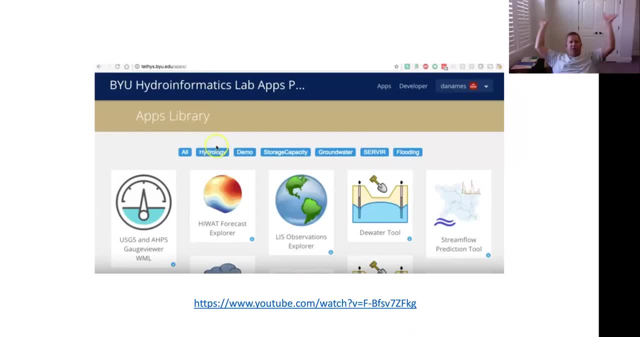 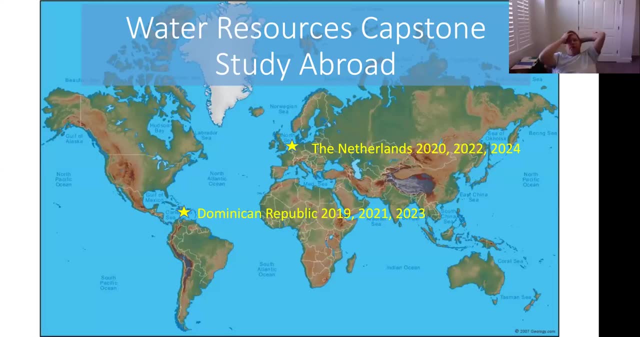 Hydroinformatics problem. It's water combined with information science, information systems. Another cool thing we do in the water resources group here at BYU is we try to host a study abroad program every year as a capstone senior project for people. So 2019,, 21,, 23,- in odd-numbered years- we're taking groups of students to the Dominican Republic. 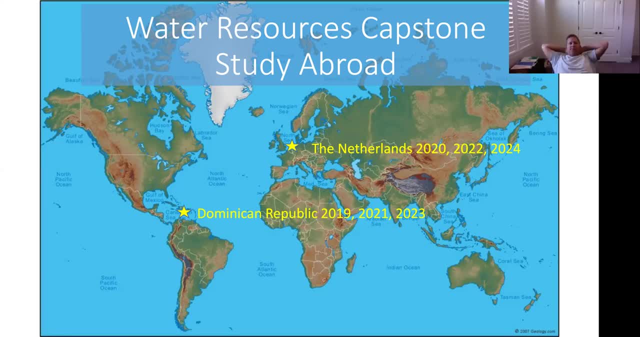 And then, in even-numbered years, we take groups of students to the Netherlands. And you may ask- you should be asking this right now, actually, Dr Ames- why the Dominican Republic and the Netherlands? What's so special about those two countries? 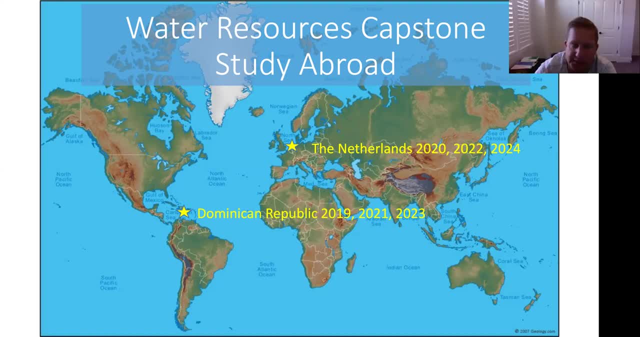 The answer is nothing's particularly special. I mean, they're cool countries. Dr Nelson served his mission in the Dominican Republic And I have a bunch of colleagues and people I work with and do research with in the Netherlands. Well, what's really cool? 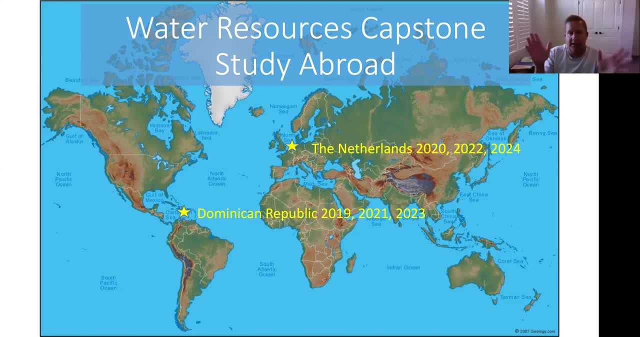 About these two places is they create this interesting like yin and yang or a dichotomy of water, where in the Dominican Republic it's a developing country where water is very scarce, water management and information and modeling and so forth is not very advanced. 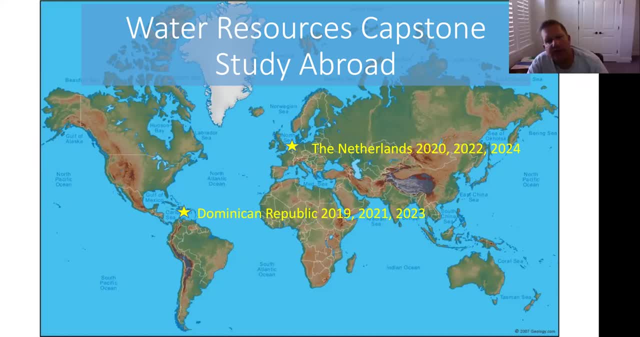 And so we send BYU students to the DR to teach them about better water management In the Netherlands. the Netherlands has, for a thousand plus years, been the leaders in water resources management, building dams and dikes, And if, without water management, about two thirds of their country is actually at or below sea level. 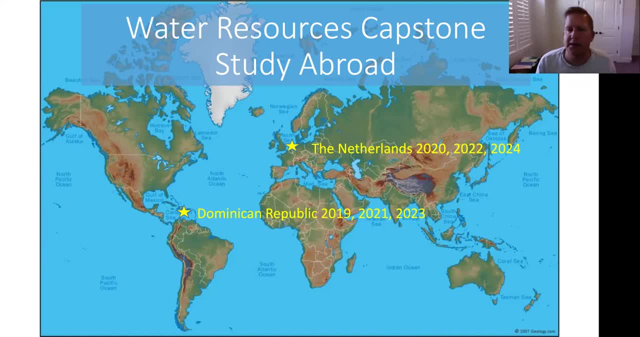 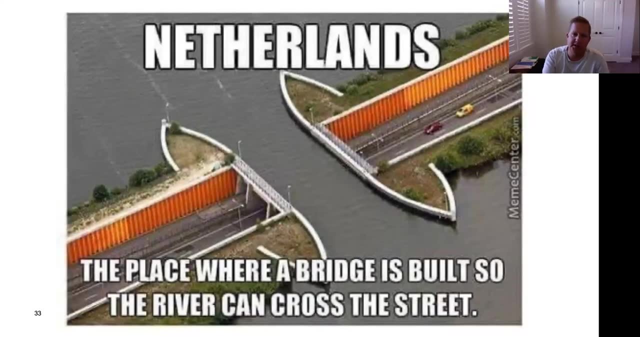 So some of the best water engineering schools and best water engineering methods come out of the Netherlands. So we go to the Netherlands in even a number of years to learn about water engineering. Either way, it makes for a fun study abroad. Here's the Netherlands, the place where a bridge is built so the river can cross the street. 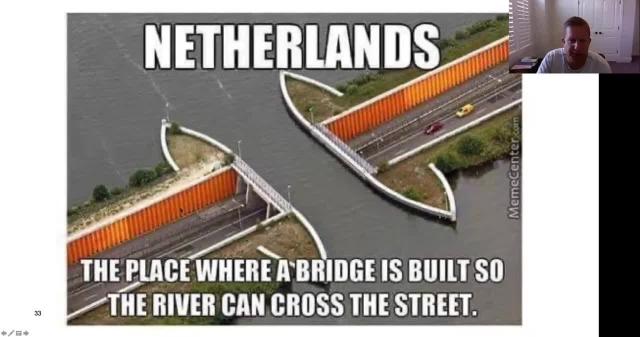 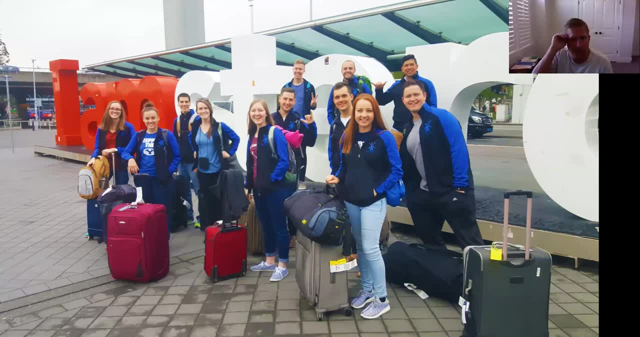 That is true. This is a place where the street goes underneath the river. Love it. This is just a group of our study abroad group That went to the Netherlands a few years ago And you can see they're very happy, cheerful people with matching jackets and the sign says I Amsterdam. 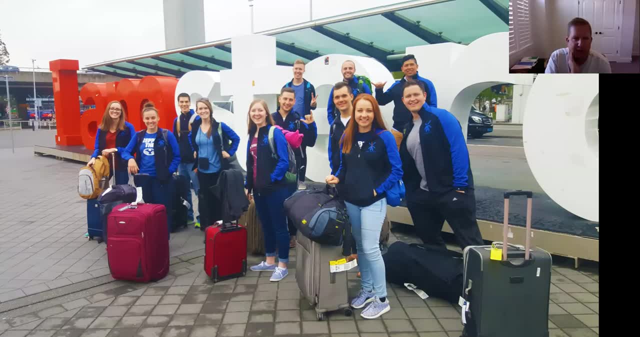 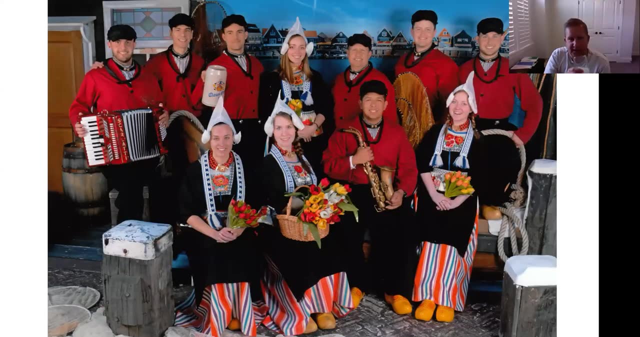 And if any of you have been to the Netherlands, if so, please say so in the chat, Then on the oh, and then they also. when we're studying water, we always dress like this. It makes people respect you more when you're walking around the streets dressed in natural. just kidding. 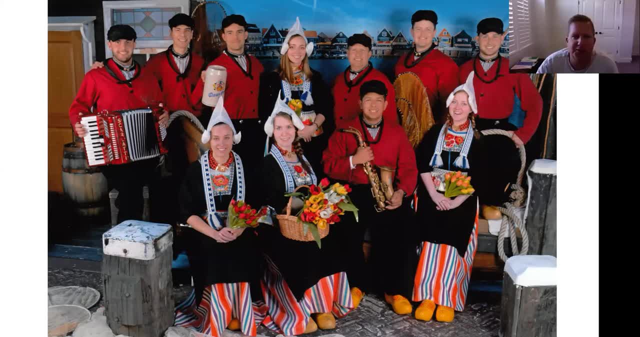 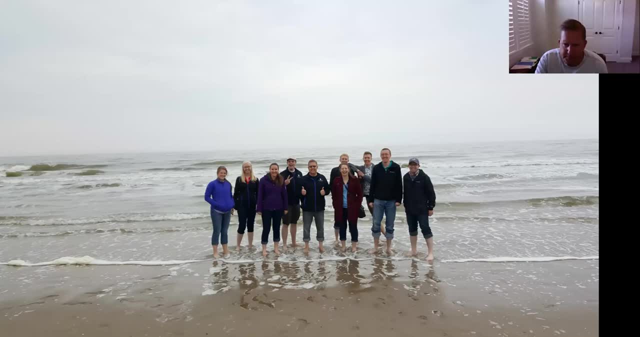 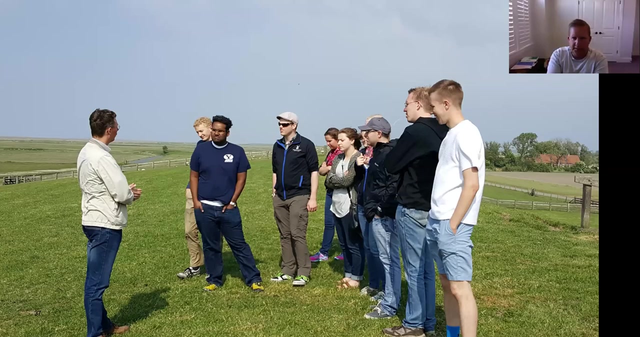 This is the Netherlands. This is actually obviously a little studio where you can go get your picture taken. I believe same group and some of maybe the same group might be a different group. I think this is a different group. Another year is standing on the North sea and freezing cold weather that time, but it was pretty fun and learning. 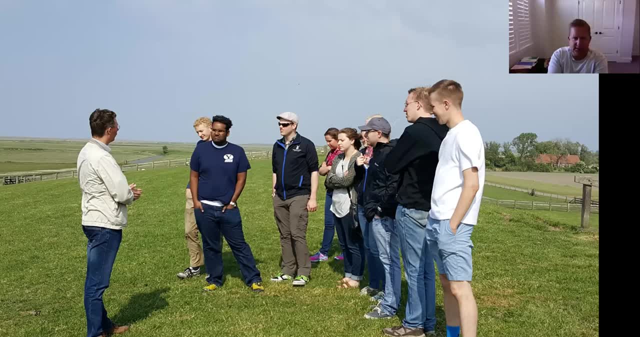 We're actually standing on a dike here. There's a different group standing on the dike, Um, on the left, On the left-hand side, you have the North sea. Well, if it's winter, this whole area will be flooded and there'll be storms lashing up against this ground on the left to protect that little house on the right. 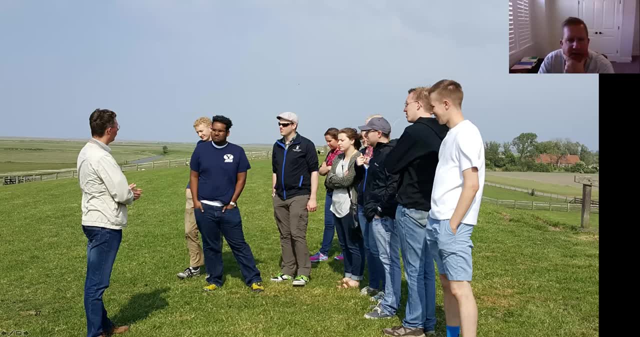 There's actually a whole villages and stuff back there on the right And these, these massive dikes extend all the way across the uh and around parts of the Netherlands to check mark. really interesting to see how they do that, And they've got some of the leading edge technology also. 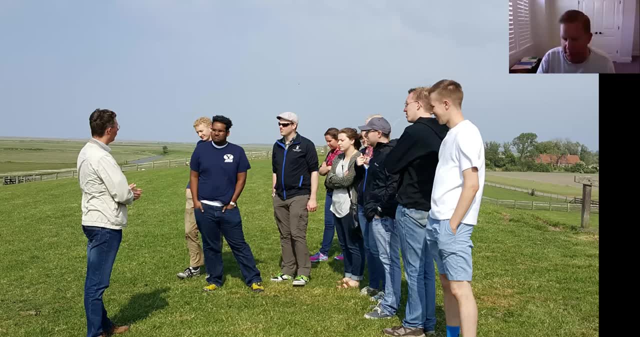 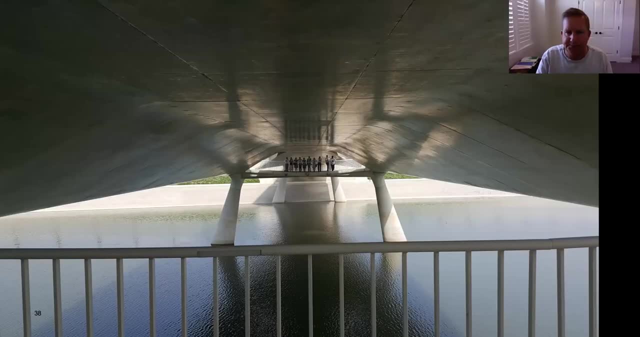 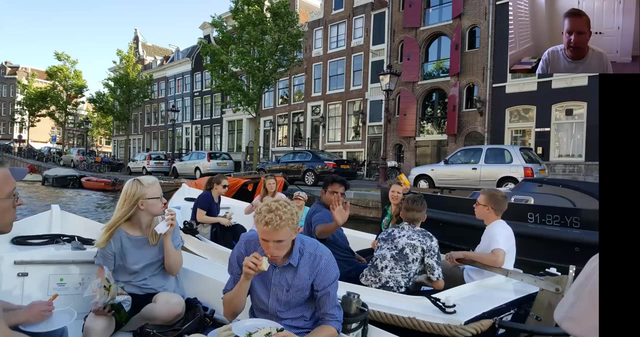 So, using old style technology, just build a big pile of dirt to keep the water out and leading edge computer technology to analyze it and stuff. Here we are inside A massive dam, or a ridge actually, and also having some fun. I'm telling you all this because you can maybe start planning ahead and plan to go on a study abroad program for your capstone. 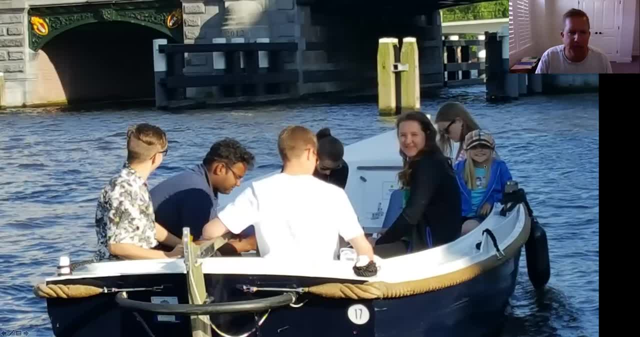 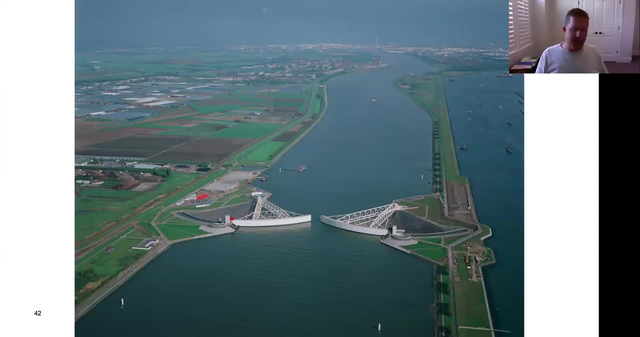 And that's my daughter on the far right there, The cute little one. Uh, this is the largest movable dam the world. water resources engineers built this together with electrical engineers, instructional engineers and geotechnical engineer. took took the whole group. 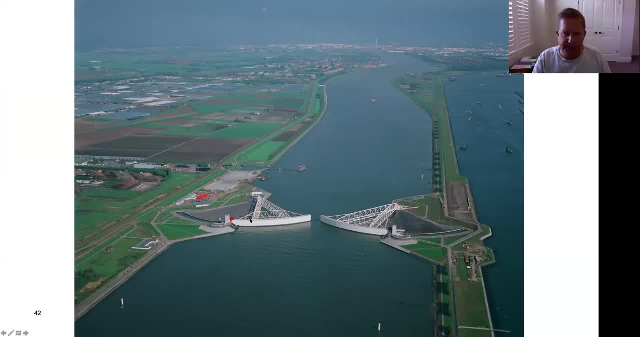 Okay, This is a- this is seriously a turn off Facebook and Instagram moment, because, look, look over here at what I'm showing you: each one of those arms. they move out into the river to block the river when the floods are coming up the river, and it's to protect the city off in the distance, that's Rotterdam, off in the distance, up there. um, back in the 1950s, uh, a large number of people in Rotterdam were killed, over 5,000 people- due to floods. 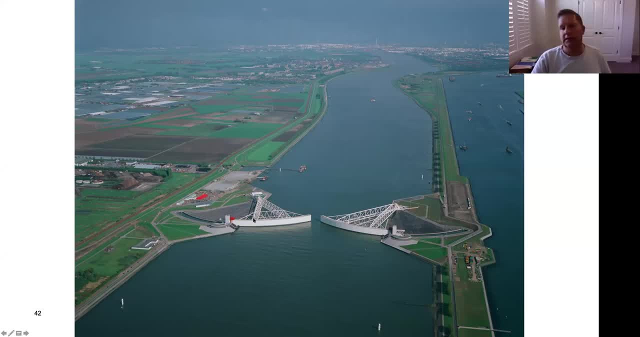 That came through, And so they spent, in the nineties and the early two thousands, a couple of billion euros to build these dams like this, all throughout this area, And this one, each one of those. if you took it and stood on edge, it's the height of the Eiffel tower in Paris. 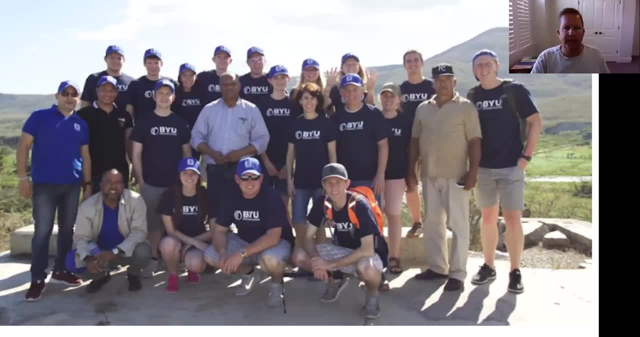 Amazing movable dams. Okay, Here is a group of our study abroad students down in the Dominican Republic together with some- uh, some- of the DR colleagues and people down there. There's Dr Nelson and his wife kind of in the middle of right over here. 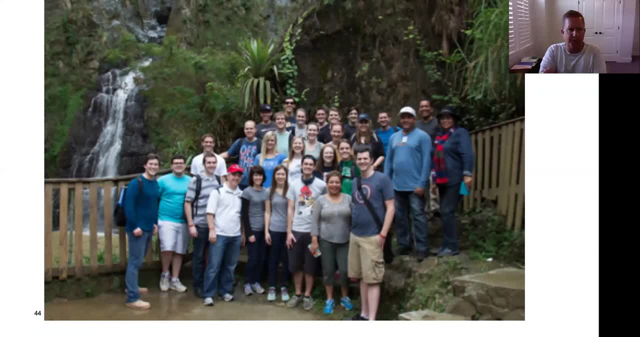 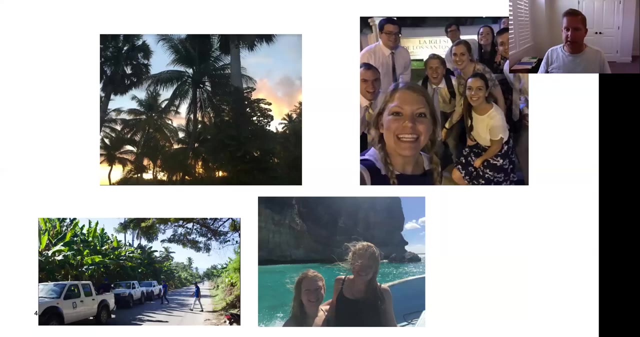 And you can see they also have fun. They go exploring interesting places and go floating down rivers And, um, actually that kid went to both of them. He was in my picture too, So somehow you've enabled it to go on both programs and they eat a lot of really good food and the DR, as you can imagine, and they have see some beautiful sites. 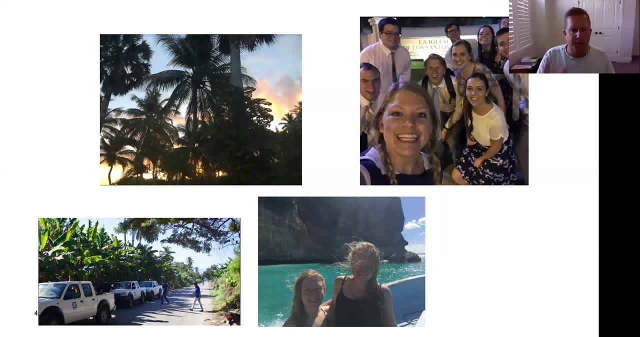 And then they also. they see the temple, We see the temple in the Netherlands, And then when they're in the Dominican Republic, they also do some cool um modeling and analysis for the local country there in the government agencies to show. 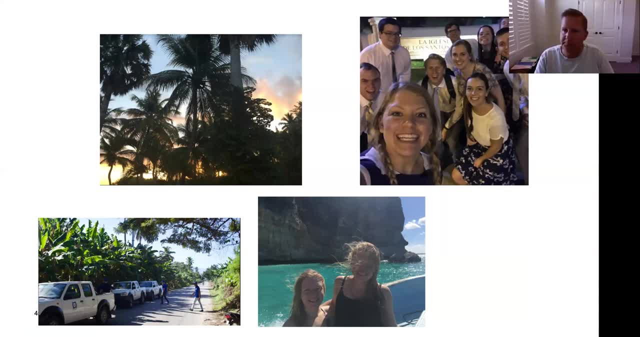 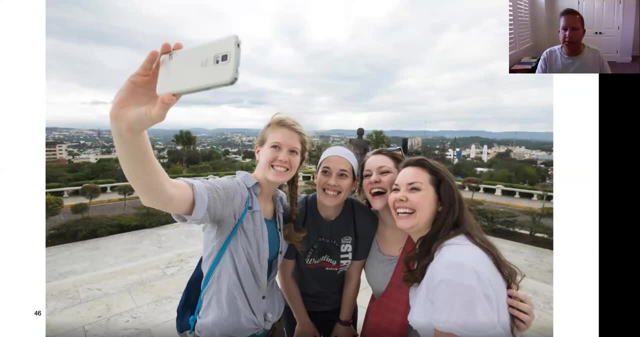 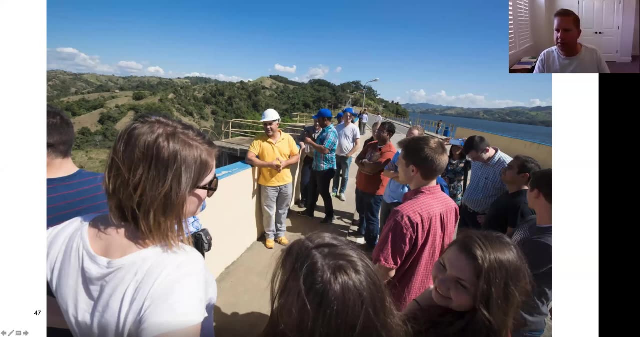 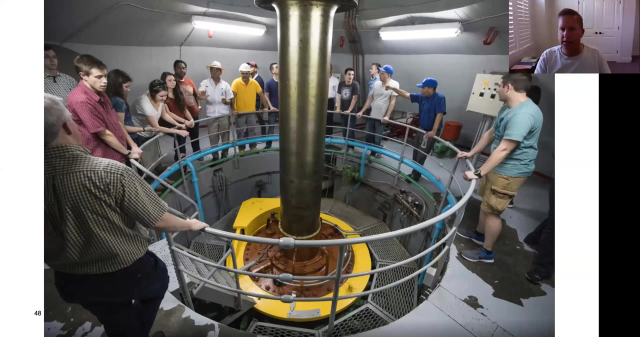 Show them where they could build dams or how they could better manage some of their water. happy, cheerful civil engineers in the Dominican Republic- And that kid too. actually that's Sardapola, He went on, both of them. So some people they just get all excited about study abroad and pack in as much as they can. look at this inside of a. there's a turbine inside of Dan. 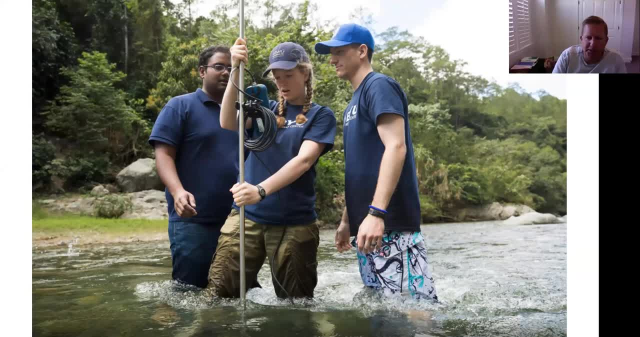 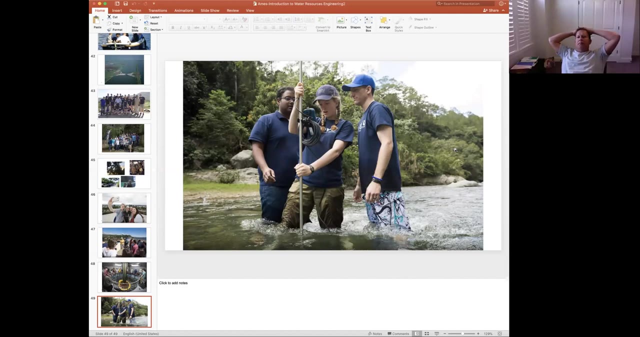 And this is a posed picture, but these folks are looking at flow in this river right here. So that's just a really brief, kind of quick and sudden overview of water resources and sharing. I would love to take the last two or three minutes and answer any questions any of you may have. 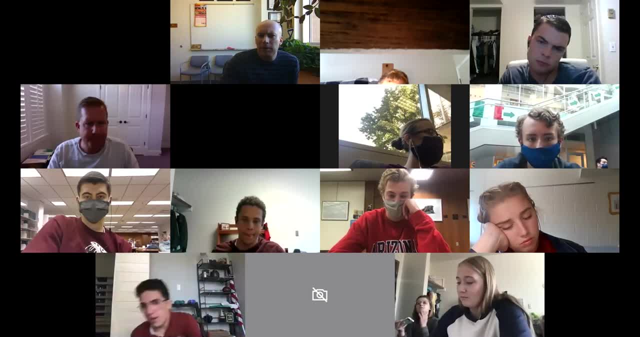 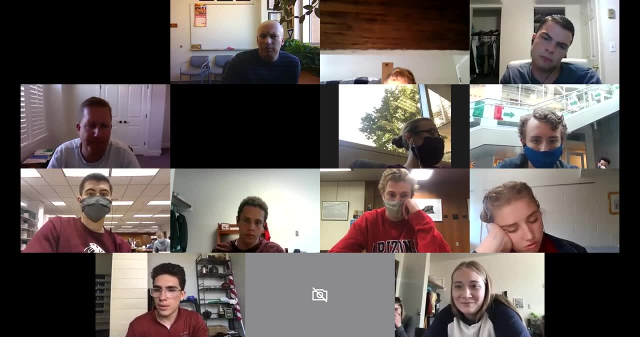 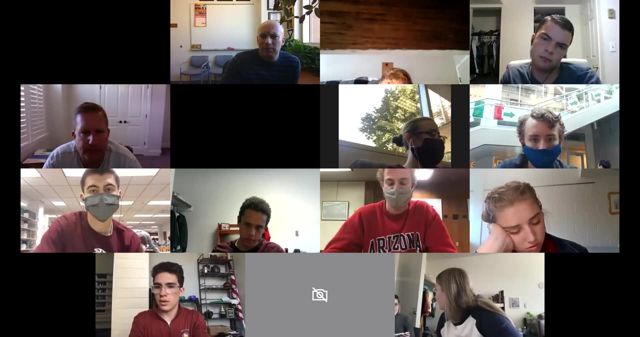 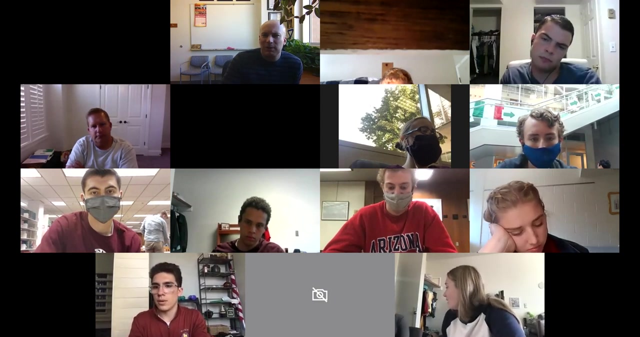 Yeah, so, um, if, why don't we have everybody lower your virtual hand and if you have questions, um, then you can raise your virtual hand? I see a couple of virtual hands raised. I don't know if these people have questions or they're just ignoring me, but, um, Trevor, do you have a question? 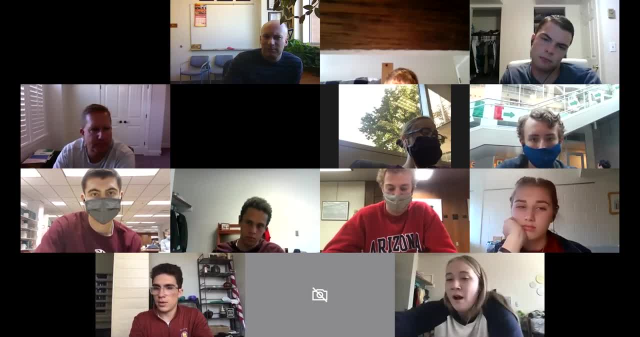 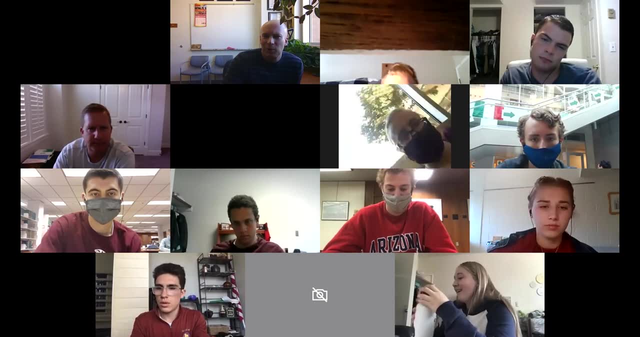 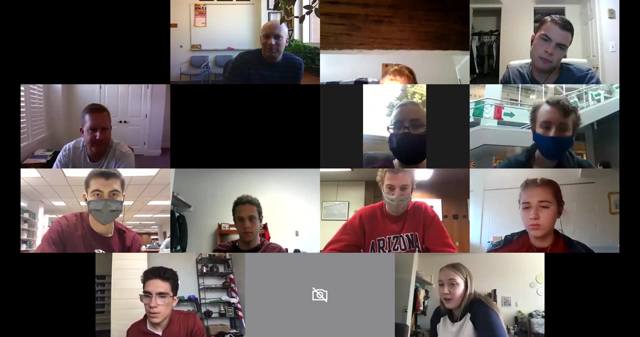 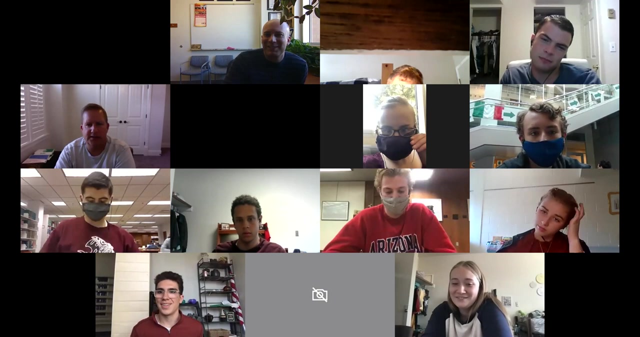 Trevor Trevor Hatch- Nope. Lydia, do you have a question? Lydia Coyle: Nope. How about Rebecca? Oh man, we're finding all the people who aren't listening. Maybe have people do the yes symbol, for if they have a question. 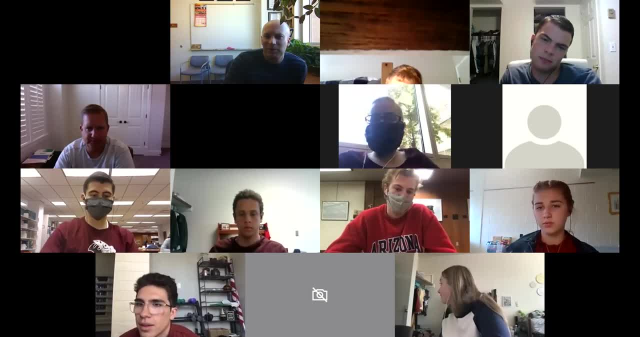 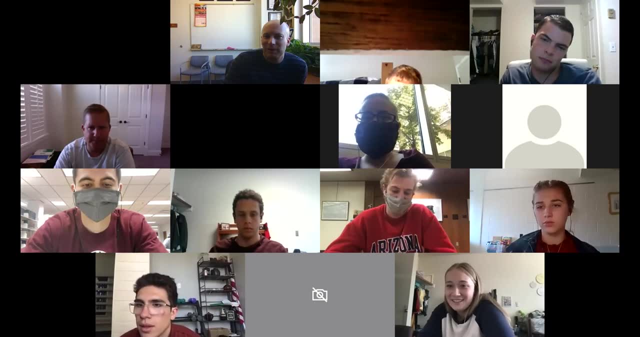 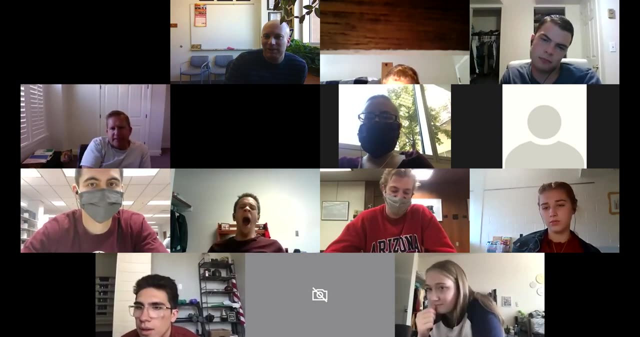 Okay. so if you have a question, do the yes symbol. I see one yes symbol. Where did it go? My problem with the yes symbol is it doesn't rise to the top. There, it is Okay. I see Jethro has a question. 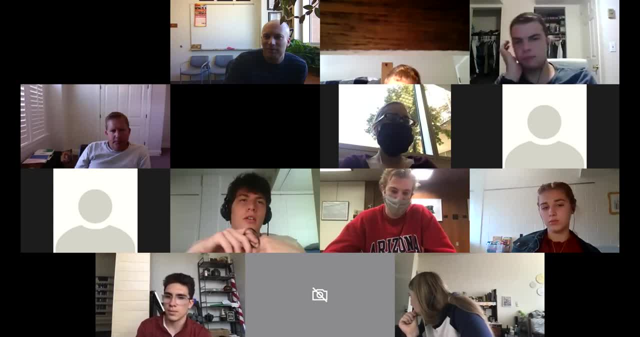 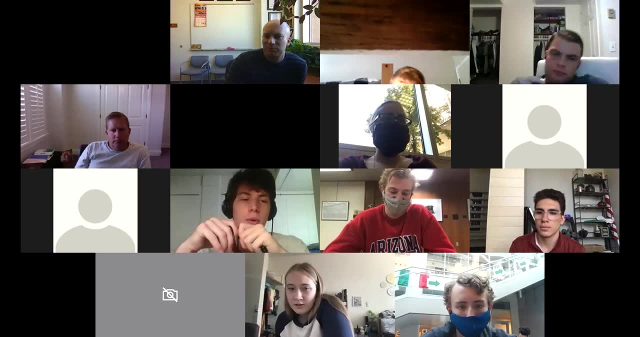 Yeah, I was wondering, like how is there a significant difference between jobs and and like water engineering from the West compared to the East, like are there more jobs out West? Oh wow, That's a really good question. 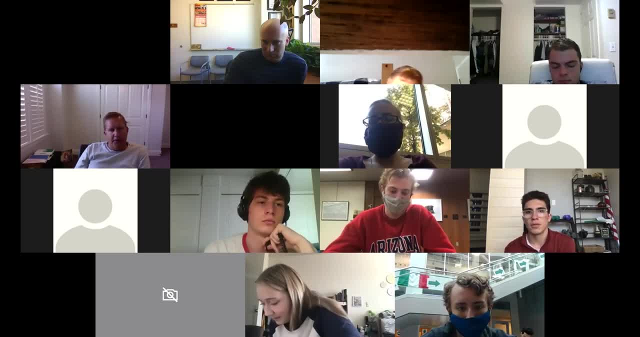 You guys know why he's asking that? Because we live in this drought, arid desert, right, Jethro? Is that kind of where you're going with that? Yeah, Yeah, So we're in the arid West. There's less water. 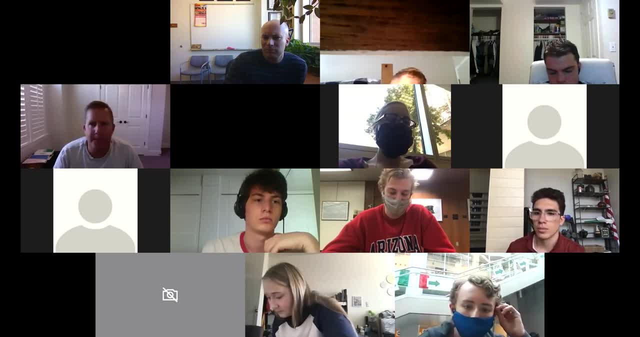 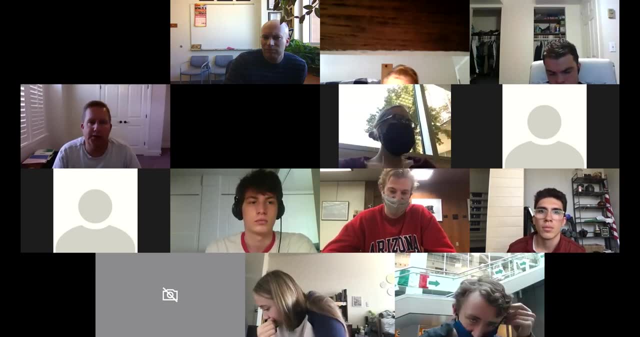 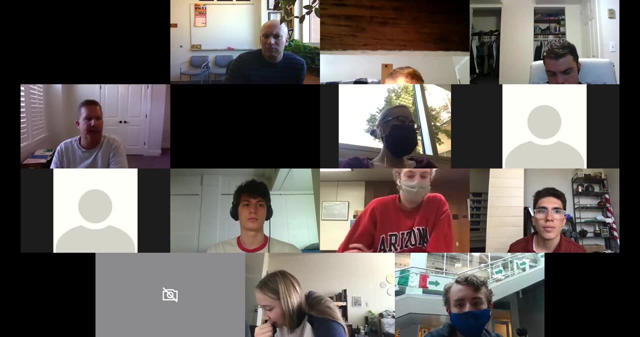 Um, I would say that the jobs are equally important and available in the West and the East. One of the largest water agencies in the country is actually the St John's um water district in um West. They're a district in Florida and they've got a ton of water and they're managing Everglades and sort of managing the too much water side of things or enough water quality for the habitat and the environment, versus out here in the West where we're managing the not enough water. 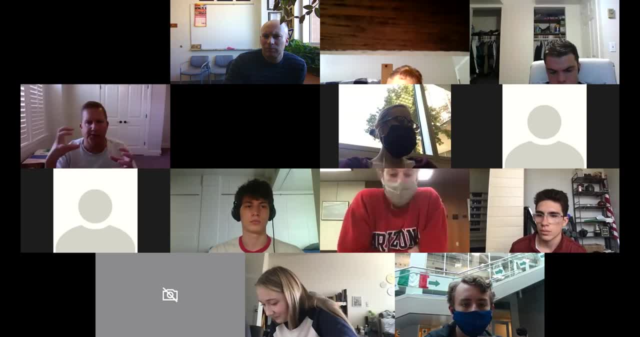 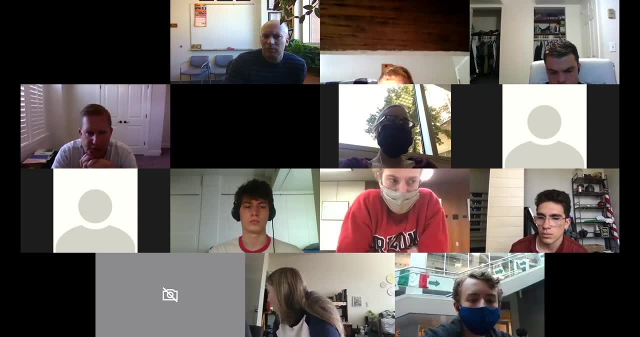 When we go to the Netherlands, we usually team up with a class over there of students and the students- the Dutch students, the American students- we get together and do a team project. It's fun because the Dutch students are always a little bit mind blown when we talk to them about how we have to build a dam to store water. 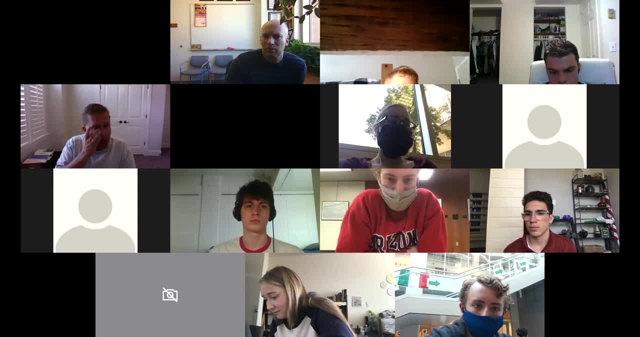 Yeah, So that we can have it to use for irrigation throughout the year, because most of what they're doing is just trying to get rid of water and try to hold it back and stuff. Both sides of the problem, Jethro, have lots of um, lots of jobs. 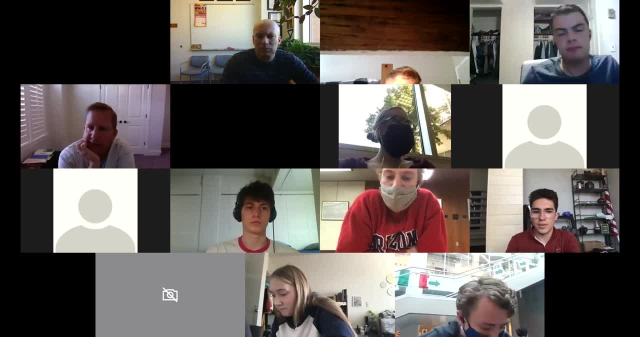 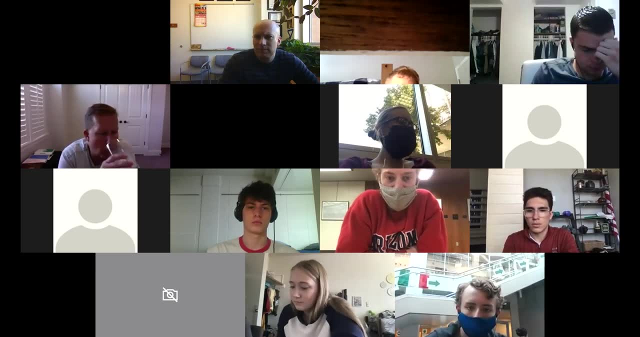 Yeah, Water engineers, if anything. there may even be more back East. I think Um Easton also has a question. Yeah, I have a quick question for you're talking about how lots of professors here at BYU have active research projects that you can get involved in, right? 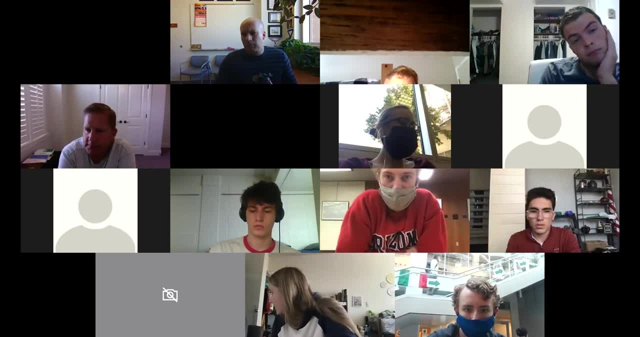 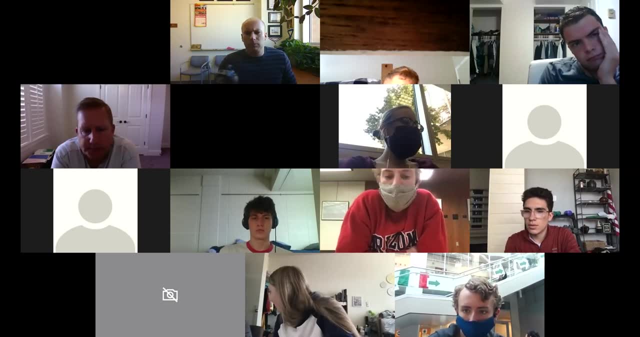 Yeah, Why? why? why you're studying. how can we um find those active research projects was the best way to get um find out those opportunities. Great question, Easton. you should all be wondering the same thing. I think um it's a matter of talking to the professors individually or emailing them. 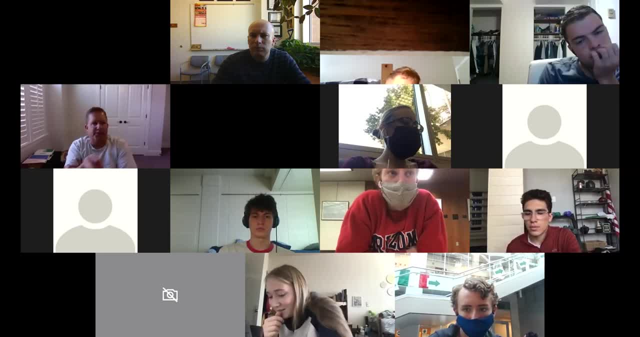 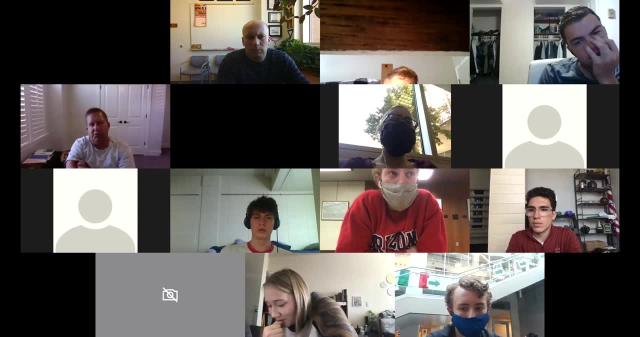 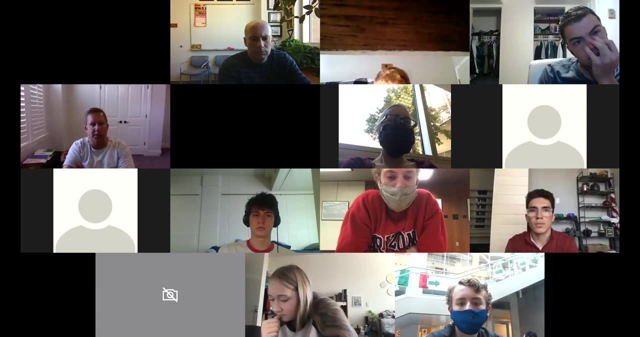 And so what you do is you get a professor that you are introduced to like in a case like this, or your teacher is teaching a class in civil engineering, or you look through the list of faculty and civil engineering on our homepage. You see something that they're doing that's interesting, and you just email them cold and say: Hey, I'm Easton Perkins just wondering if you have any cool, interesting research going on in the area of blah, blah, blah. 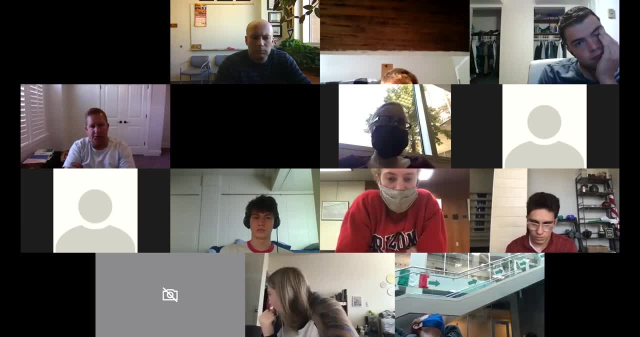 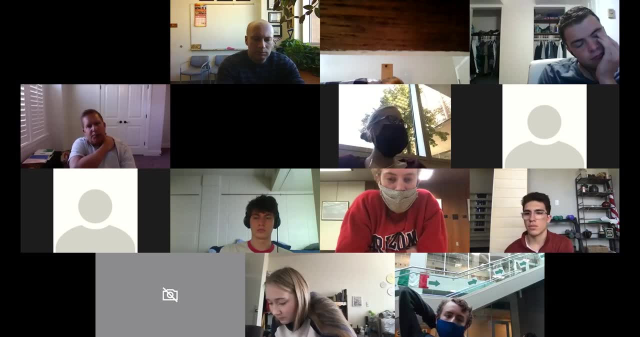 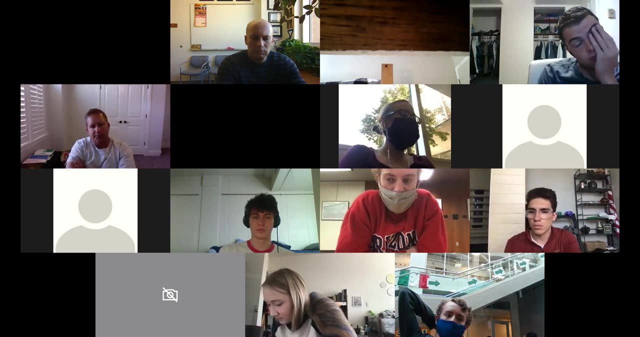 Um, I would, or if you're taking on any undergrad research assistants, cause I would love more than life itself to come and work for you, And when we get emails like that, oftentimes we we pick up students pretty quick. Um, so pretty much all the faculty hire some students and some hire more than others. 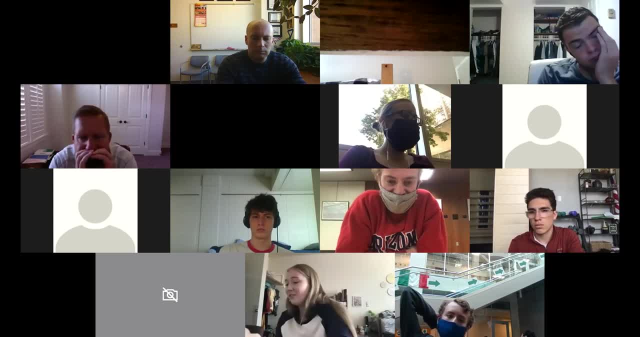 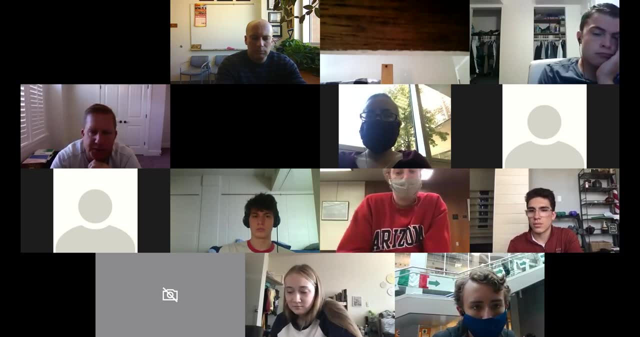 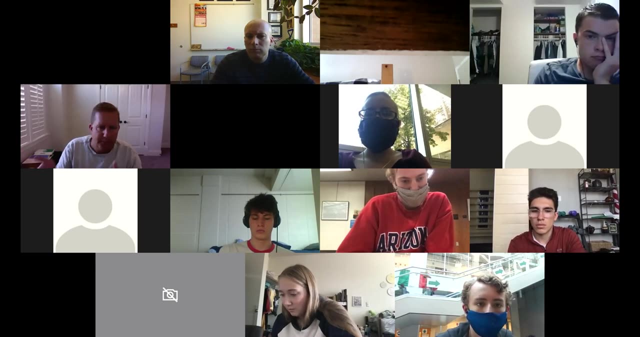 And, by the way, secret, Secret, secret- for those of you who are still paying attention and listening- secret, insider information that freshmen don't always know: Your professors don't spend all their spare time just grading papers. Like really, that's what I used to think when I was a freshman. like they come teach my class and then they go grade their papers. 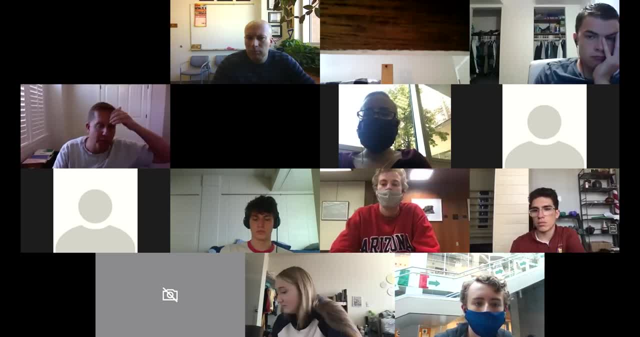 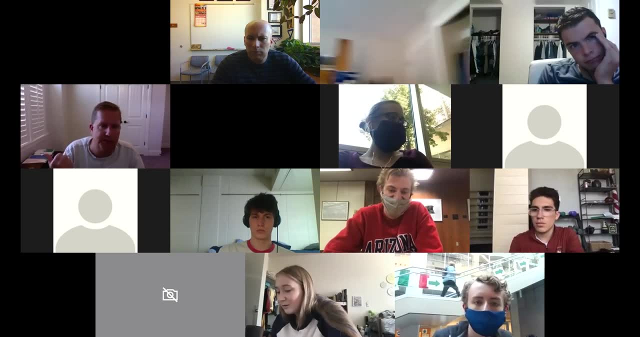 But in engineering we're not doing that. Maybe they do that in English and math, But what we're doing is we're teaching our class and then we're going off and doing these really cool research projects on the rest of our time. You should see some of the stuff that Dr Franke does. 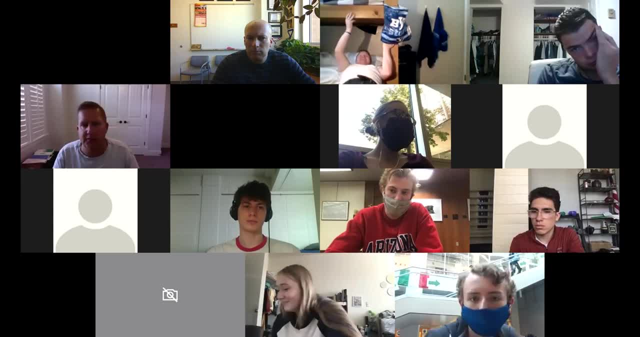 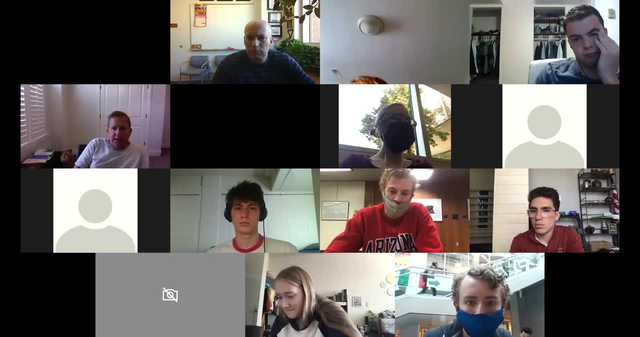 It's just like awesome, mind blowing, Fun, interesting stuff with drones, data and visualizations and analysis earthquakes and so forth. Your professors all have secret lives that they're leading and they have hired students to work with them to do that kind of work. 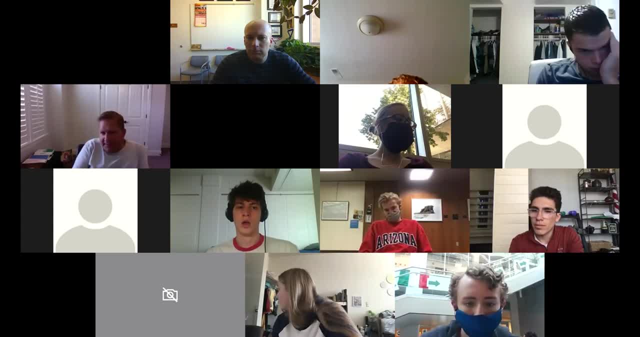 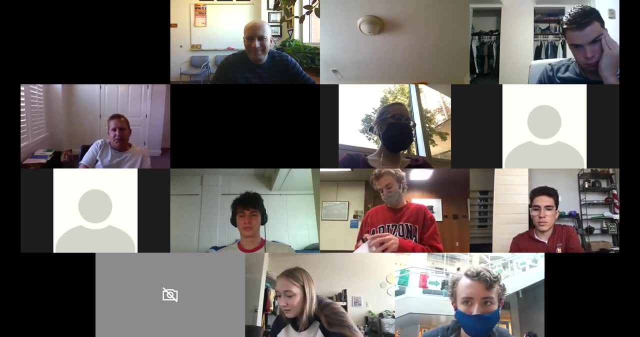 And really, yes, secret lives. And so somebody says Franke is pretty epic- It's true, He really is. And so, to answer your question, Easton, it's really just about you putting in the energy to read up on what they're doing. 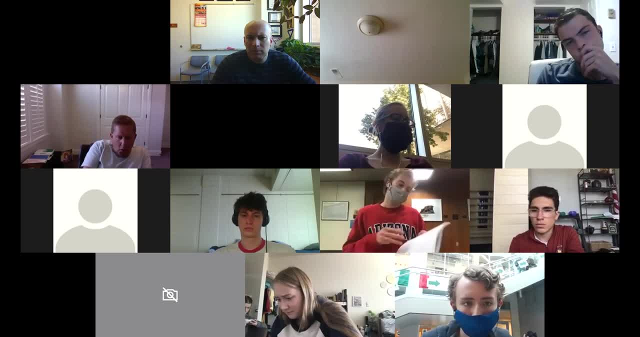 Find out what they're doing and then go and talk to them and say: hey, Dr Jones, I understand you're building water modeling models to simulate the water flow in Africa right now on a cool project. I just saw it on your Web page. 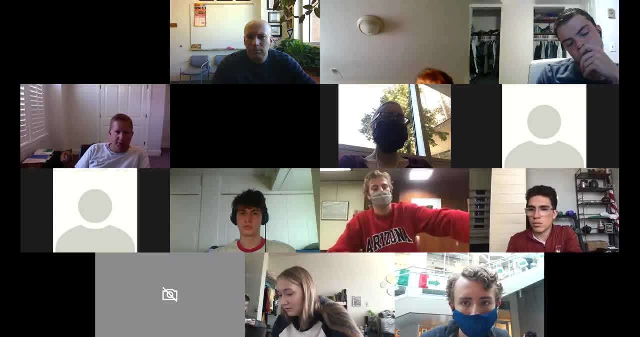 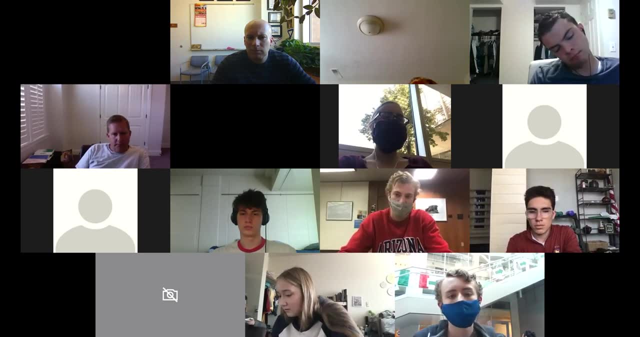 Can I come and talk to you about it sometime? Would you hire an undergraduate to process data for you this summer or this fall, And is? is it best just to follow up on that question- Is it best to wait until you're kind of a junior, getting into those classes and get experience? 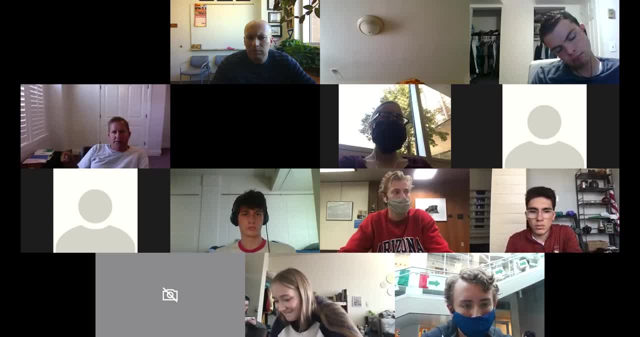 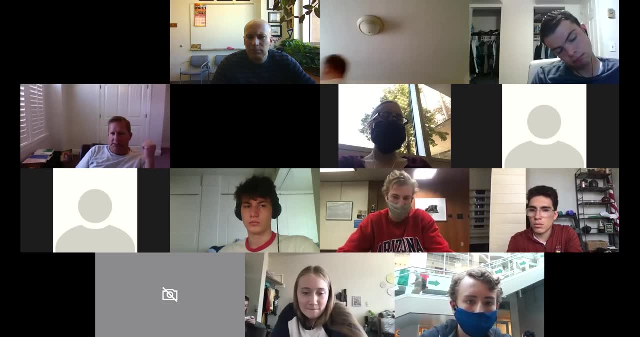 No, not at all. Our favorites are our best, I mean. in some cases, Yeah, but for the most part- like if a good, energetic, enthusiastic, hardworking student comes up as a freshman or sophomore and wants to work- they'll find a job. 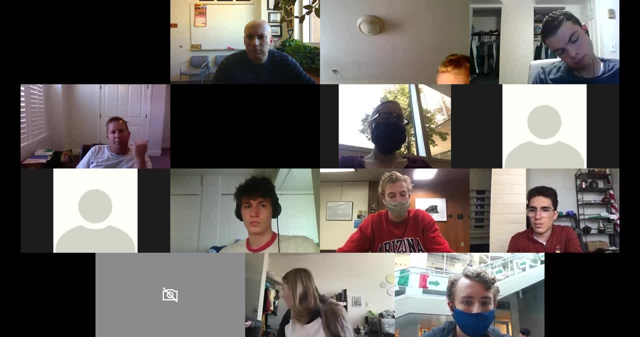 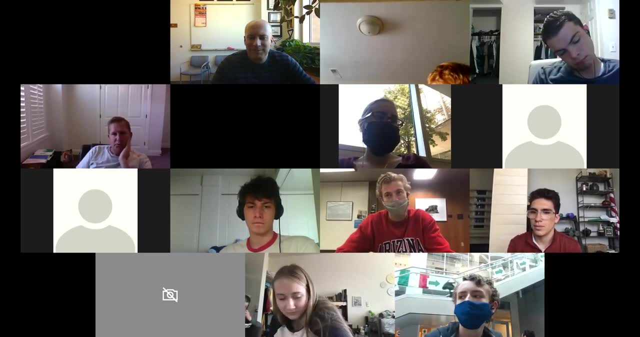 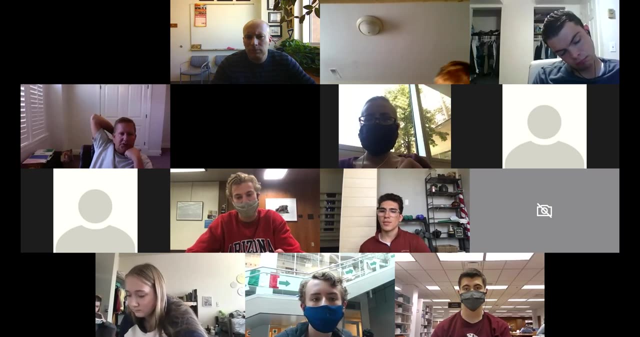 They'll find a team to work in. Now. they might be volunteer working part of their hours at the beginning. You know there might be or it might be. Yeah, I got five hours a week for you right now, But once you learn A, B and C boys, then next semester we can put you in a 10 or 15 hours a week and actually pay or something. 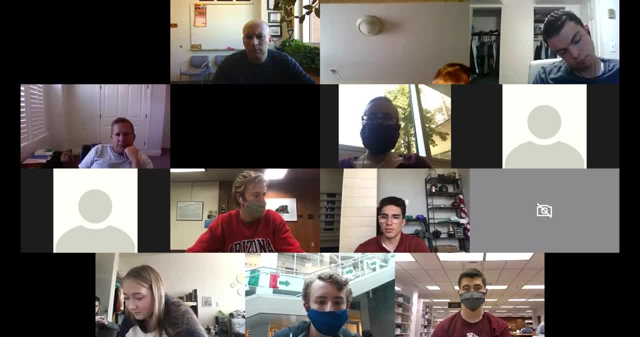 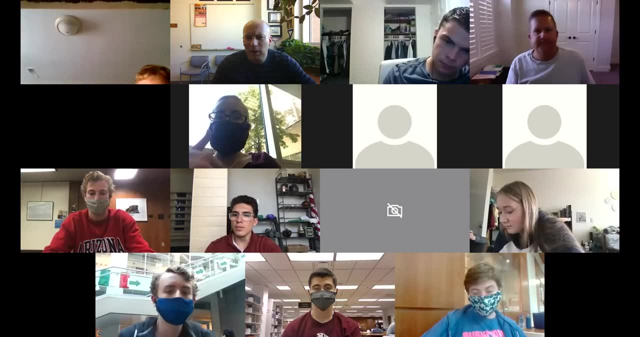 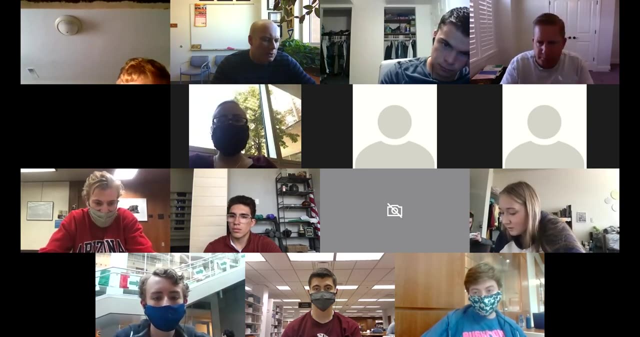 So, OK, perfect, Yeah, OK, great questions. Well, everybody, let's thank Dr Ames for coming in and talking to us about water engineering today. There are a couple more questions in the comments. I'll just direct you to email your questions to Dr. 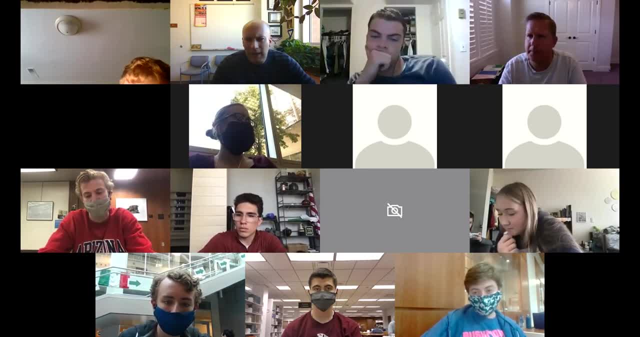 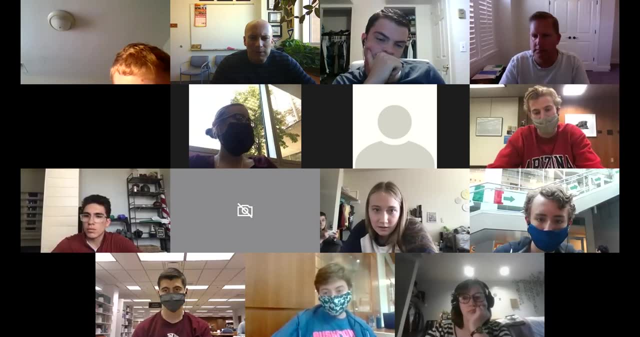 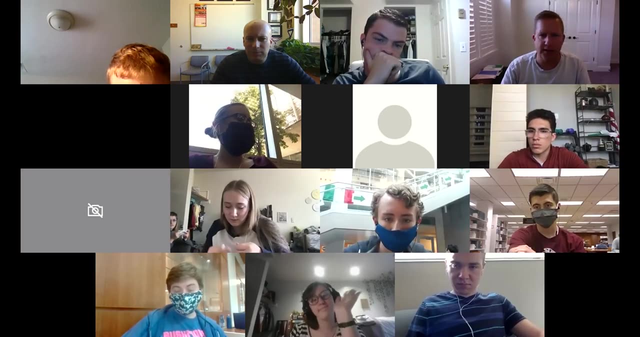 Ames or any of the water faculty That he talked about today, And they'll be happy to address your questions And I will look forward to seeing all of you next week. Thanks, Dr Ames. You bet Adios, Take care everyone.